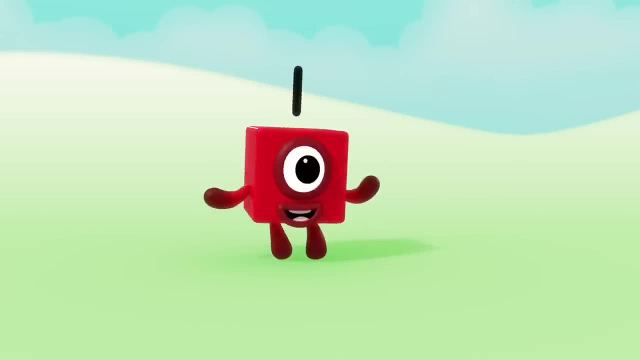 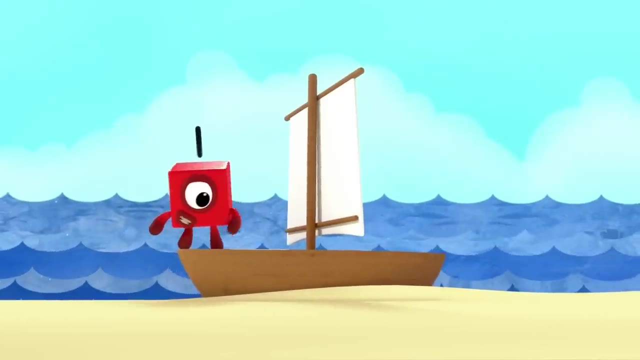 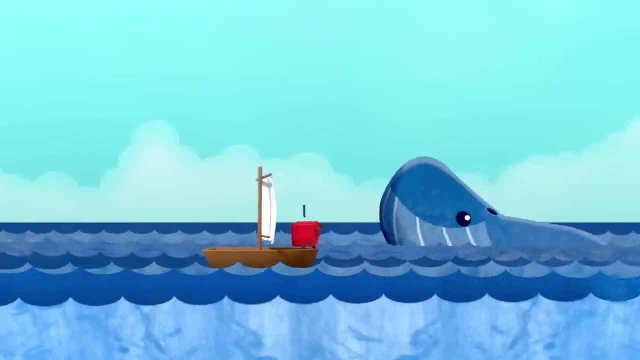 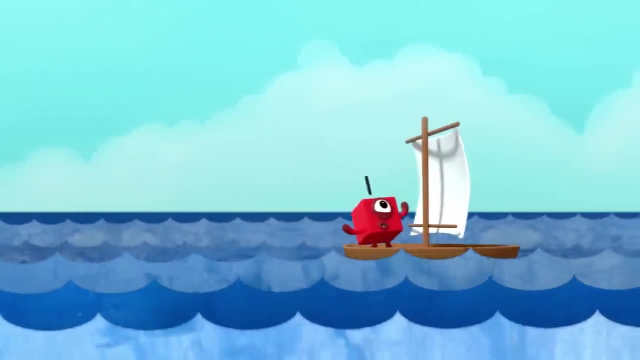 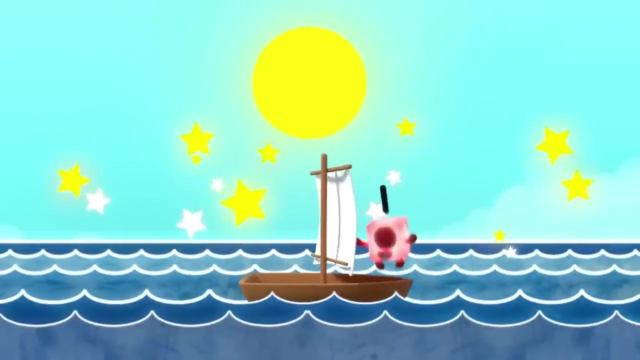 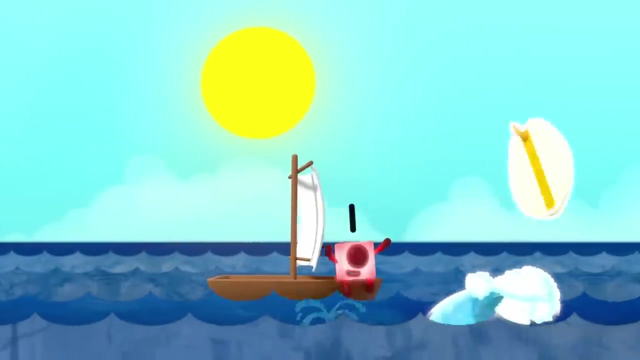 One wonderful world and one bee, One sun in the sky, One boat on the sea. One wonderful world and one bee, One whale swimming by One surfy chimpanzee. One wonderful world and one bee, One, one sun, One, one sea, One, one whale, One, one chimpanzee. 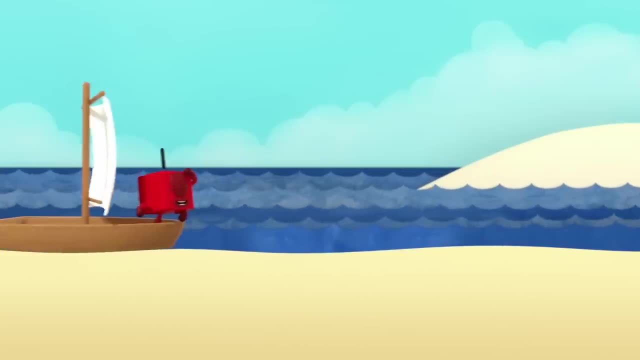 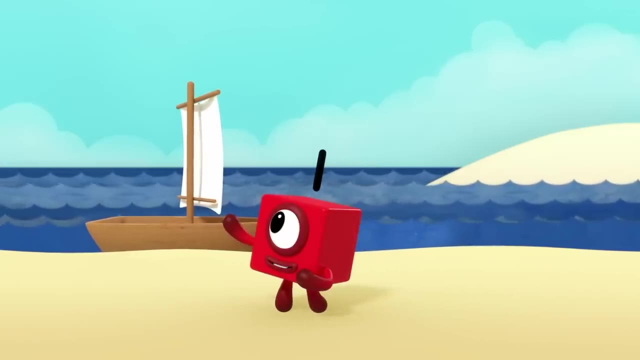 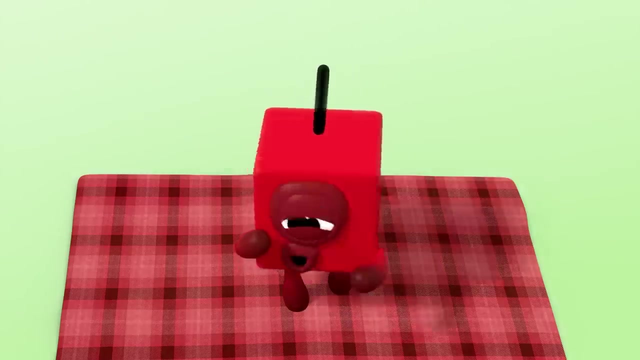 One wonderful world and one bee, One whale swimming by. When you start to count, I'm the right amount. I'm the first in line. You can count on me. I'm one in a million. I'm one of a kind. Oh, one, one blanket. 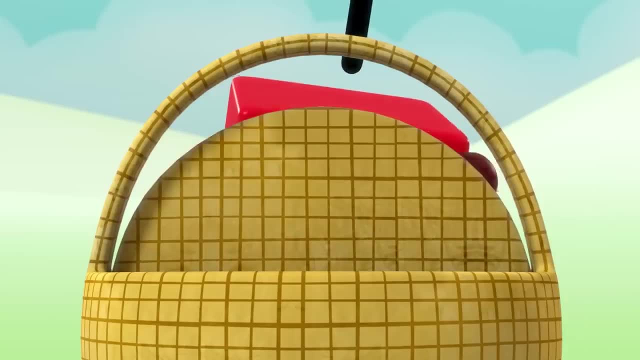 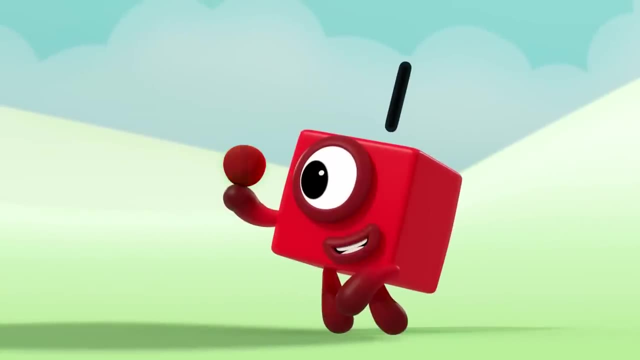 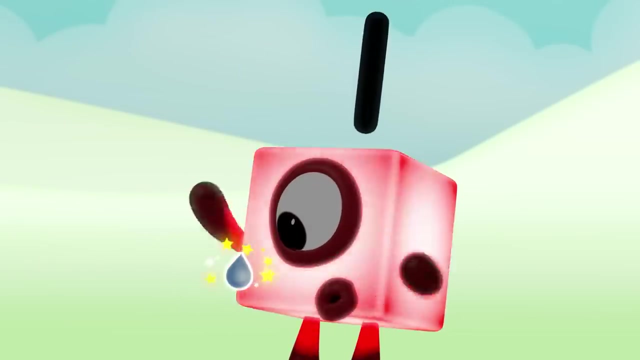 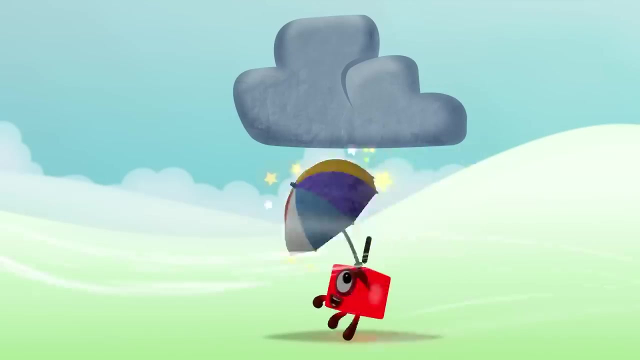 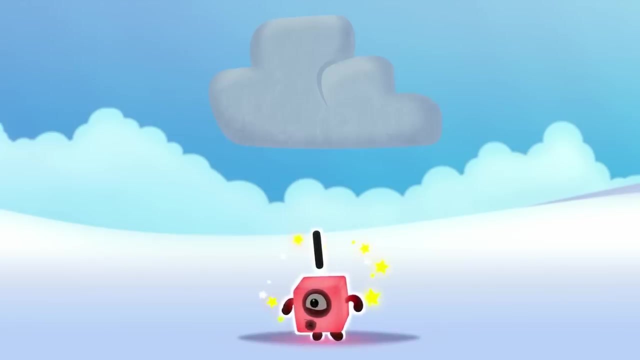 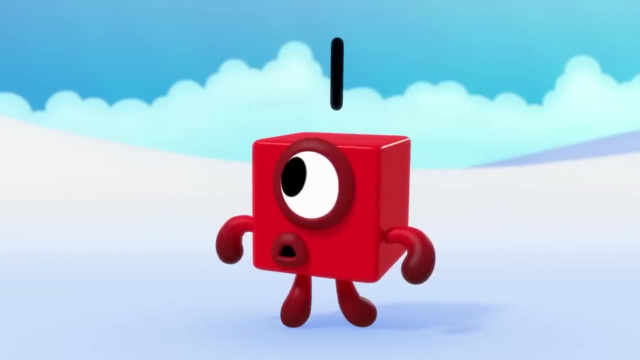 One one basket, One one apple- Hello, apple. One one cloud, One one raindrop, One one umbrella- Oh one, wet me. Did you see that, Hello? Oh, it could be lonely, But if I'm the only one, it might not be much fun being a single figure. 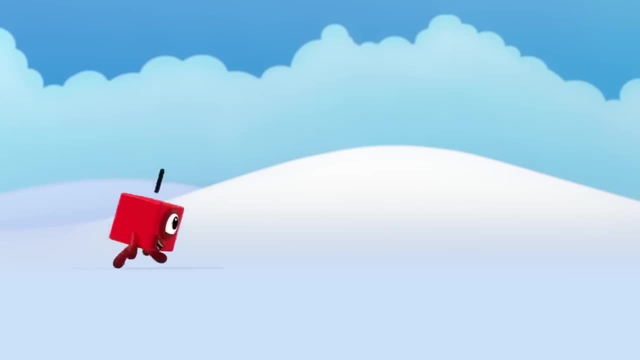 But I'm number one and I'm winning. I'm only at the beginning. I could be the start of something. maybe I could be part of something bigger. One mountain to climb, one step at a time. One horse in this race. one smile on my face. 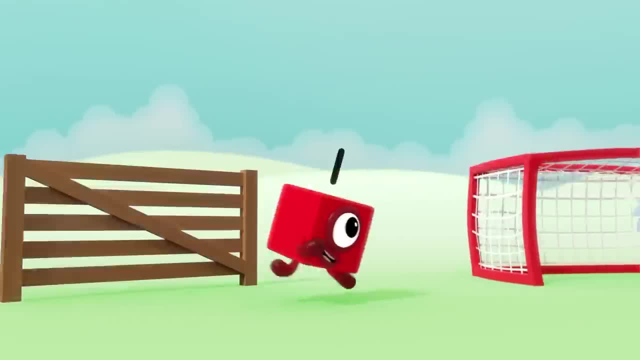 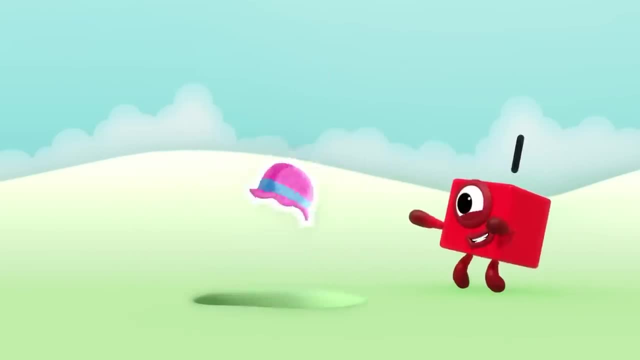 One bat, one ball, one box, one boat, one gate, one goal, one goose, one goat, one cat, one cow, one cake, one cat, one hole, one hop, one hen, one cat, One wonderful, beautiful view as far as the eye can see. 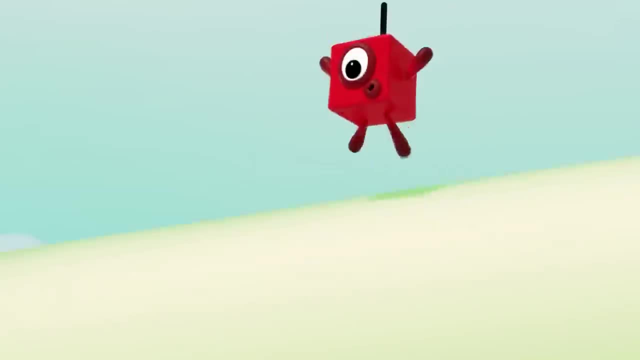 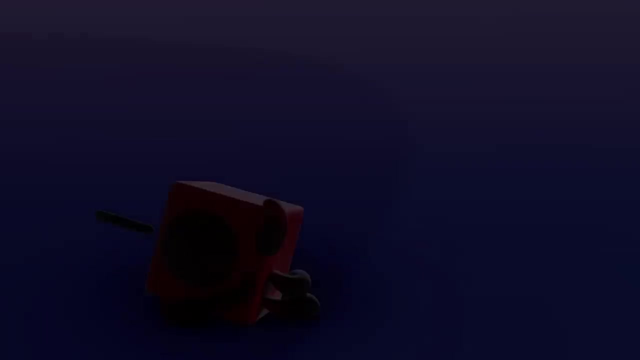 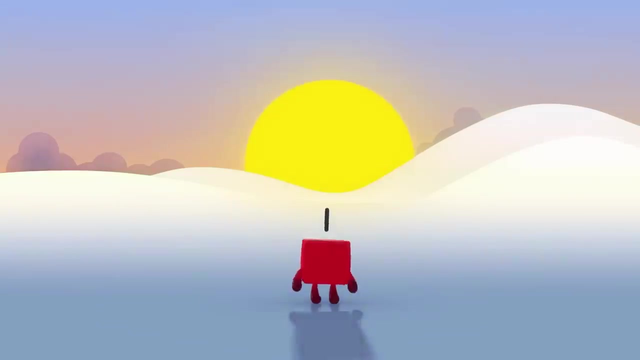 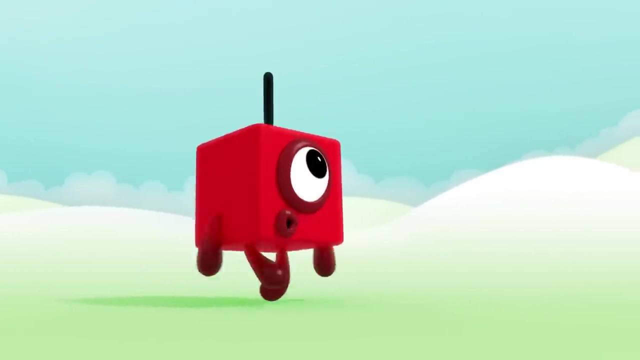 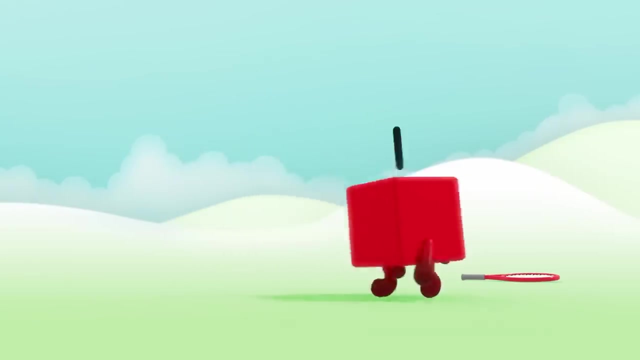 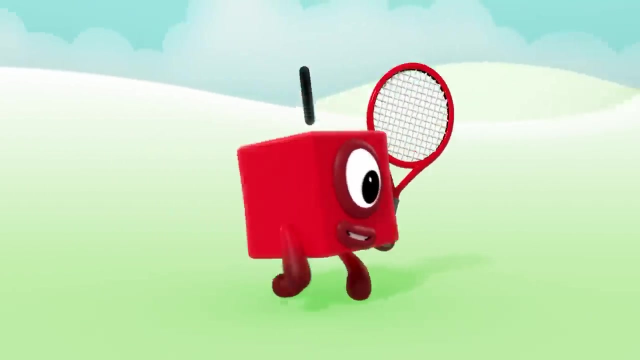 One wonderful world. one wonderful world. one wonderful world And one new world. I am one. One. One sun, Hello sun. Today is going to be one wonderful day. What shall I do? One One tennis racket. One One ball. 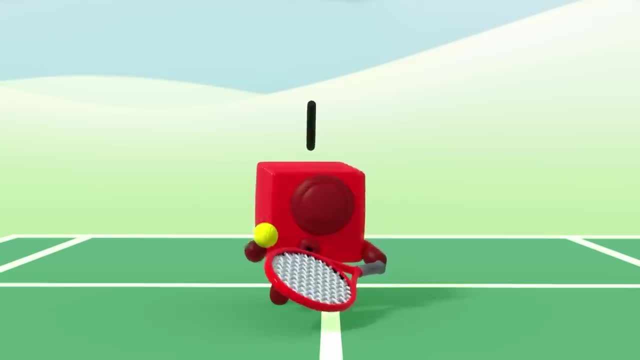 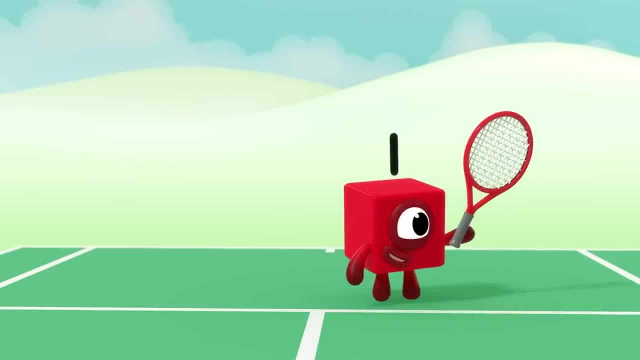 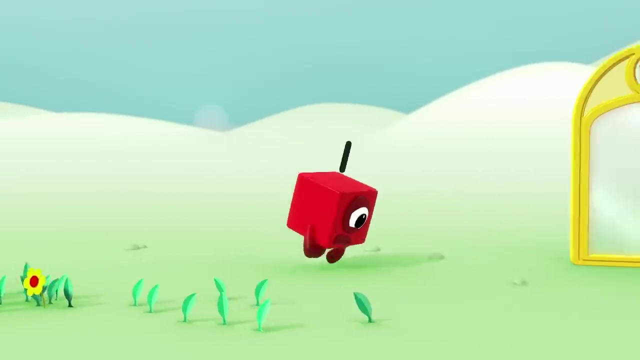 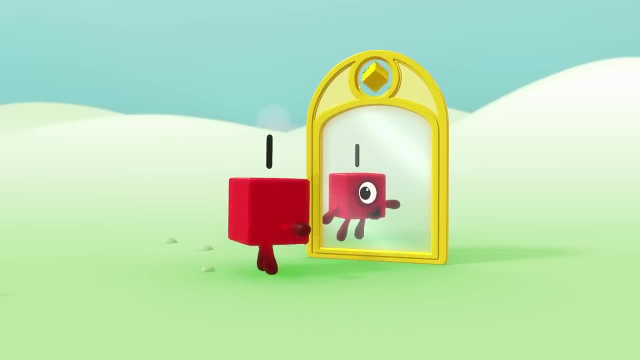 One One net. Anyone for tennis, Anyone, Someone, No one One. Oh, it's not much fun with one, One One, me, One One. whatever this is, Oh, a friend, Hello friend, I am so happy to meet you. 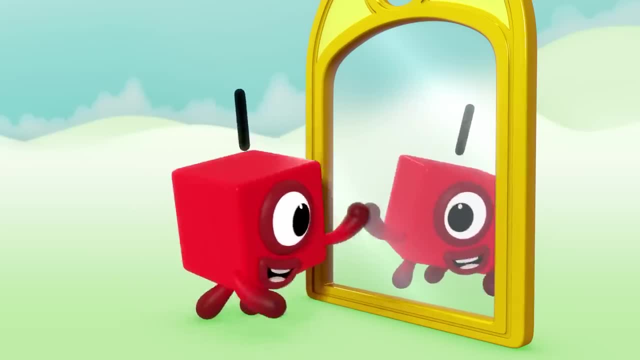 It's fun here, but I've been all on my own, and now here you are, Oh, Oh, you're real, I'm one. So am I. I'm another one. Hey, I've got one amazing idea. Tennis is more fun with one and another one. 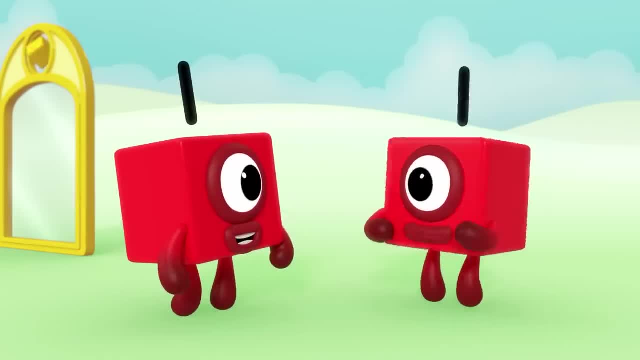 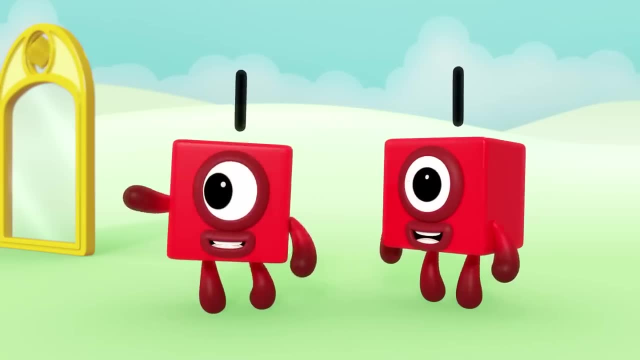 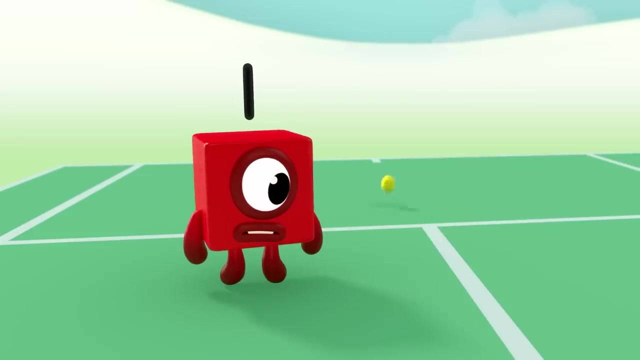 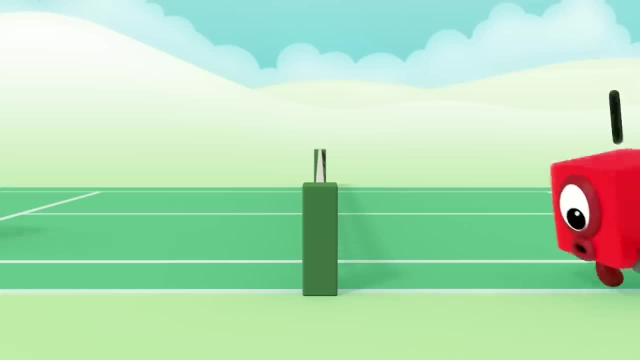 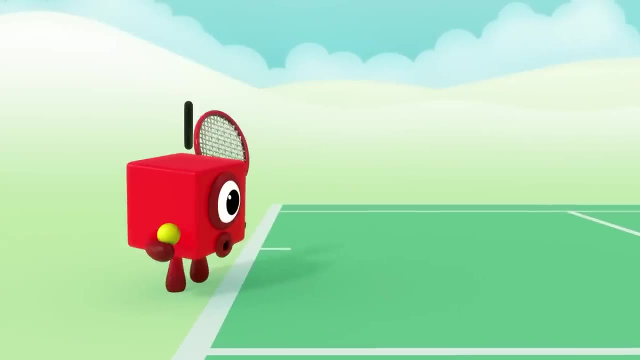 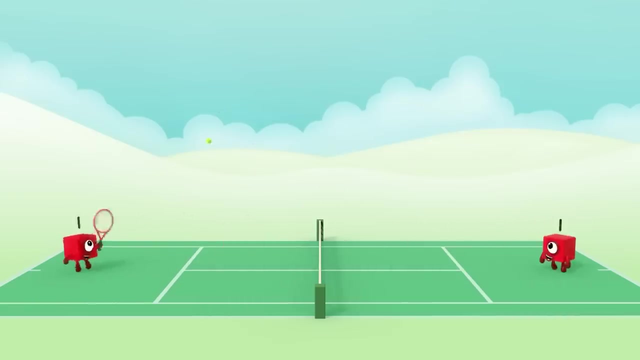 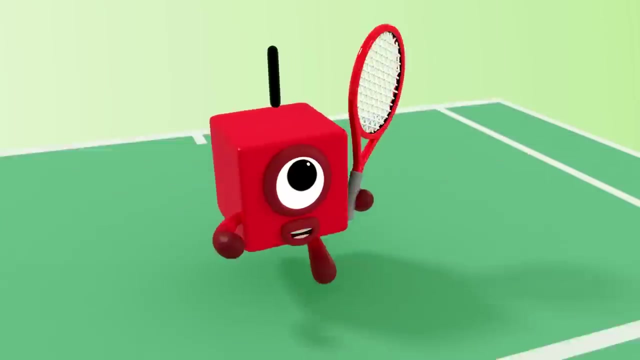 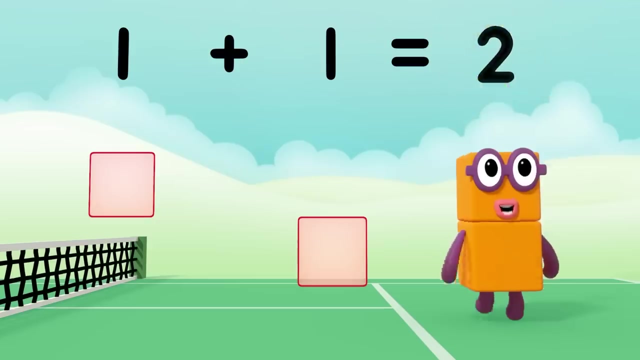 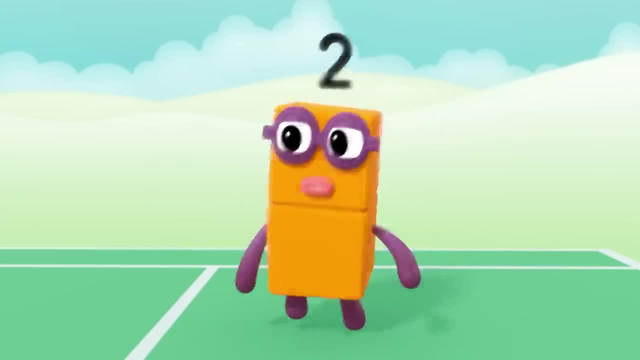 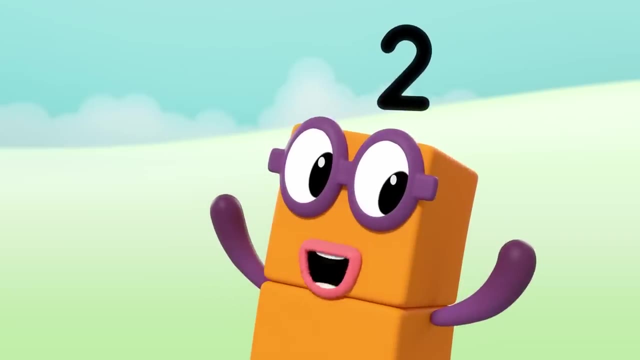 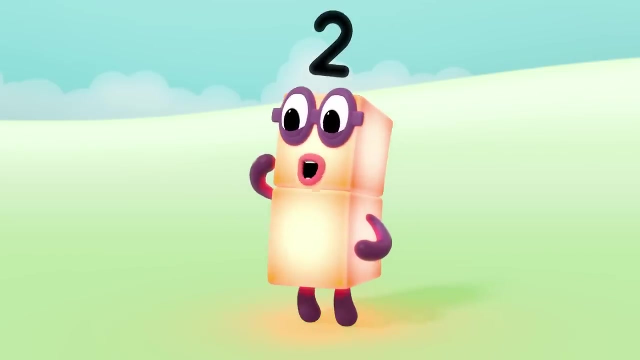 Where did they go? One and another one turned into me. They didn't go anywhere. One, two, Two blocks. I'd like to meet one. It would be nice to be her friend. Two equals one plus one. Wow, Did you see that? 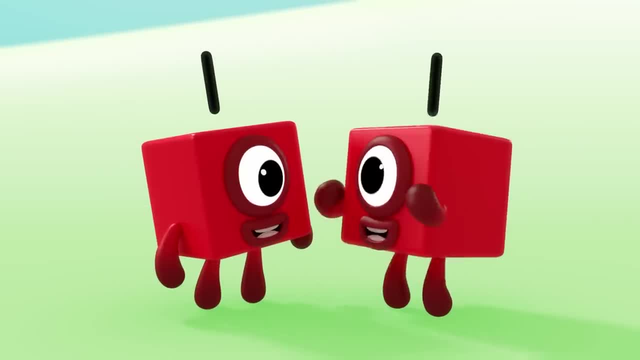 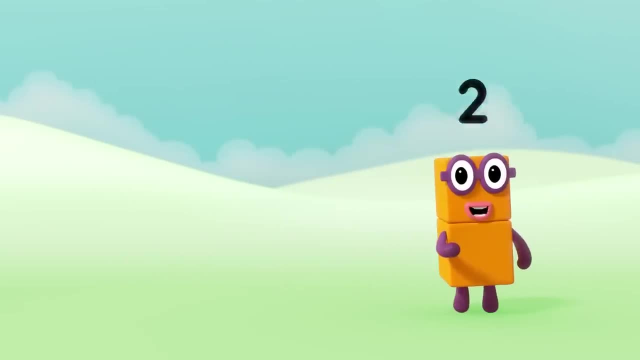 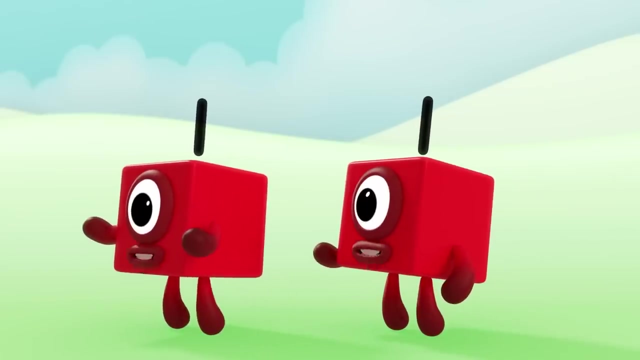 Let's do it again: One plus one equals Two. I am two. How do you do? Oh? Oh, Two equals One plus one. Pleased to meet you two-two. Oh, We already tried. One plus one. 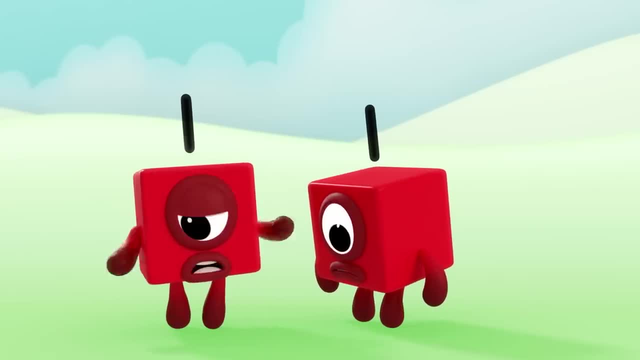 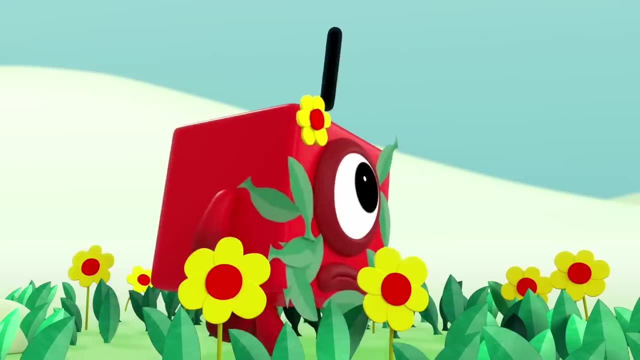 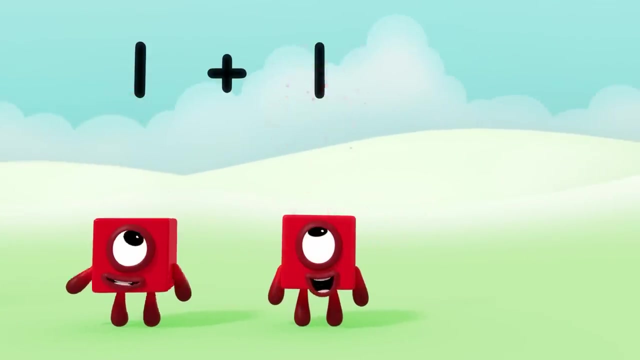 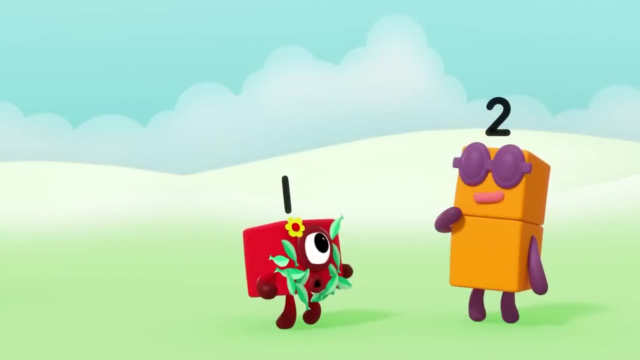 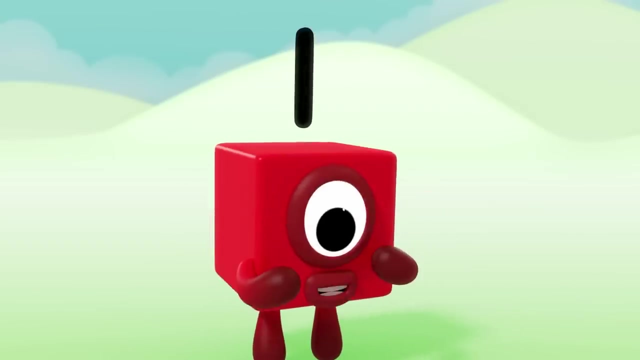 I tried that We need another idea. Got one: Oh, the magic mirror. Oh, Let's do it. One plus one equals Two. I am two. How do you do? Oh, I see, I'm one And you're two. 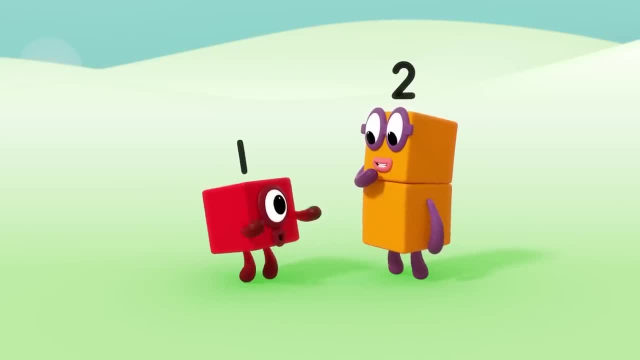 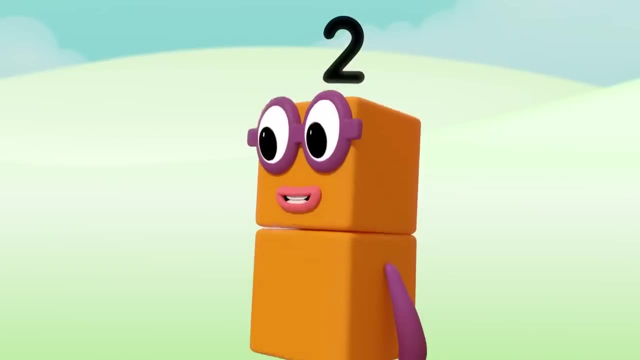 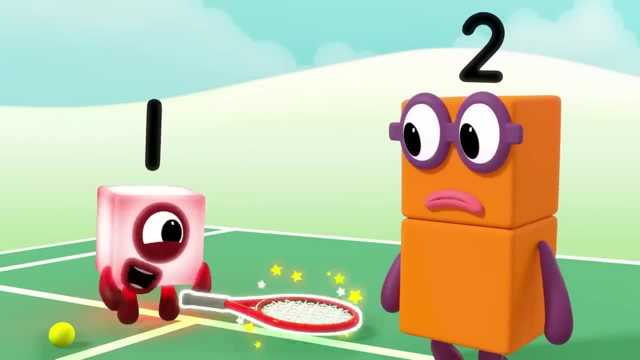 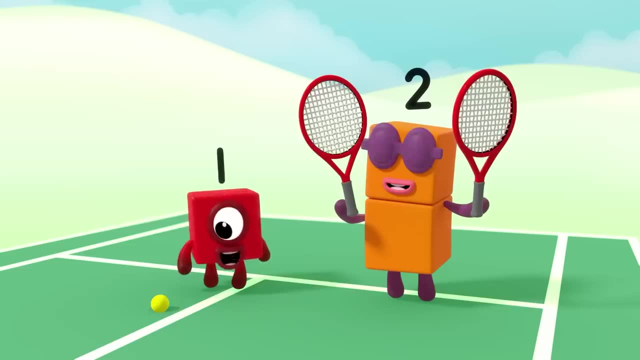 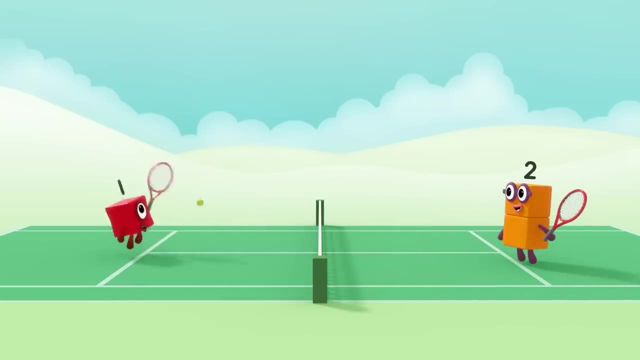 One One tennis racket. One, Two, Two tennis rackets. Oh, And one One ball. I'll go first. One, Two, One, Two. See, It's twice as much fun with two. Ha-ha-ha-ha-ha. 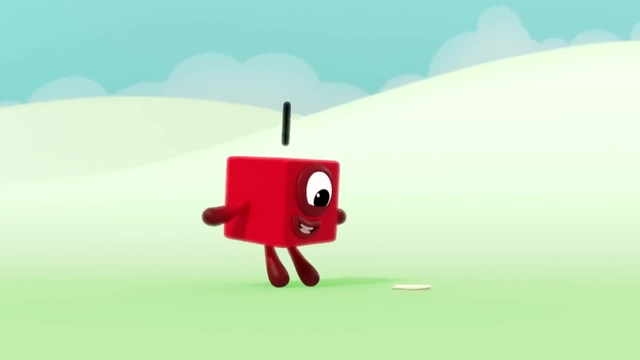 One, one, one, one, Oh One, One sock. Hmm, Something's missing. Two, Two. Come and see what I've. Oh, One, One shoe. What's missing this time? Two, we'll know. 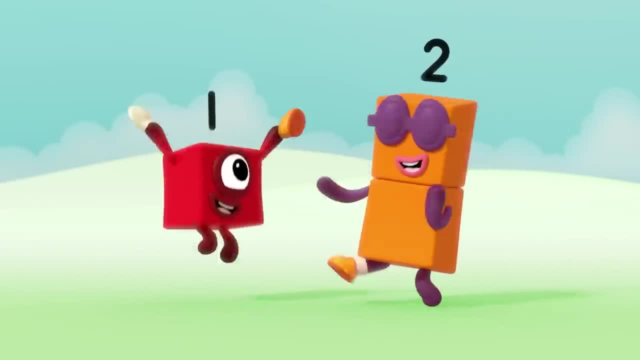 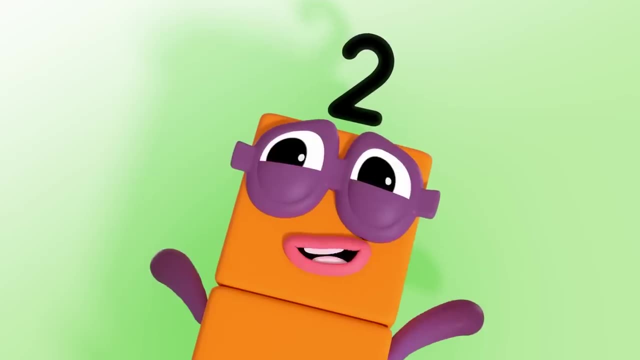 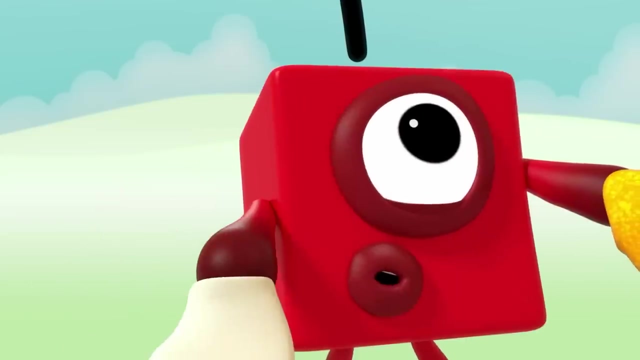 Two, One two, One two, One two. Look what I've found. Watch One two, One two, One two, Uh-oh, Oh-oh. Try yours on No two. These are for you. 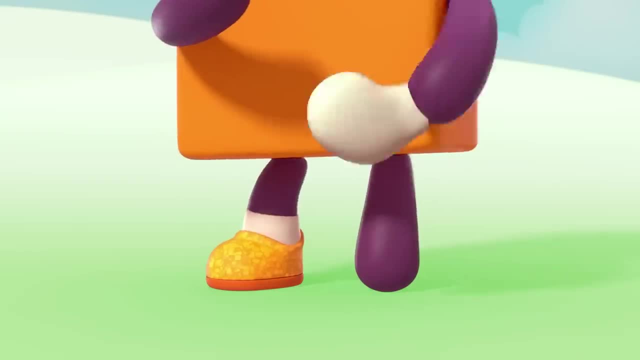 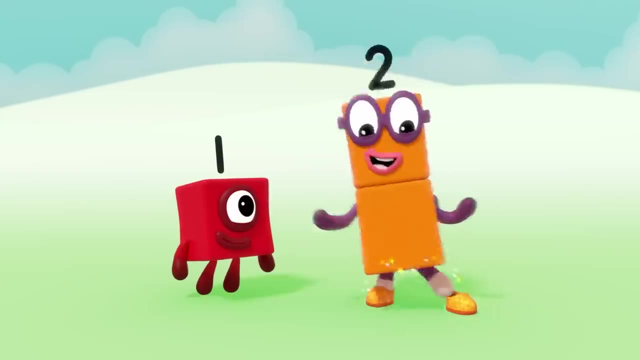 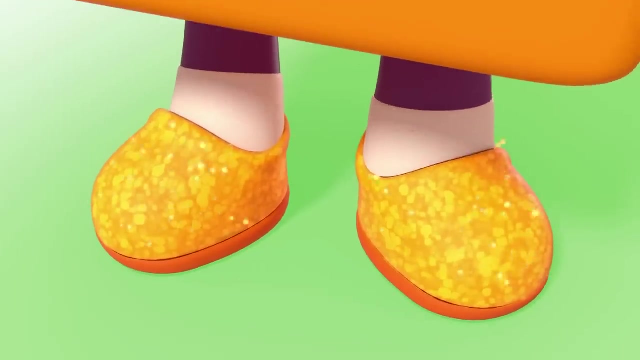 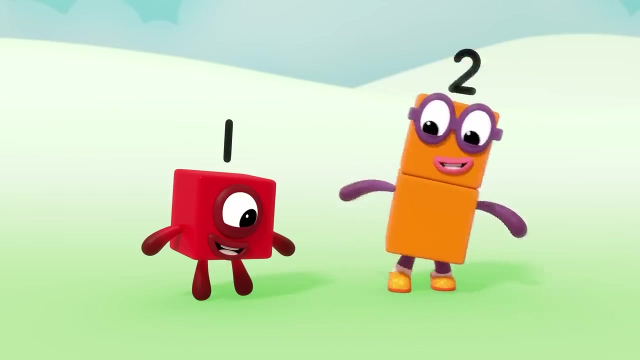 They belong together Like friends, Like friends. One two, Two socks And one two, Two shoes. My very own pair of shoes: One two, one, two. Hey, these are dancing shoes. One, two. 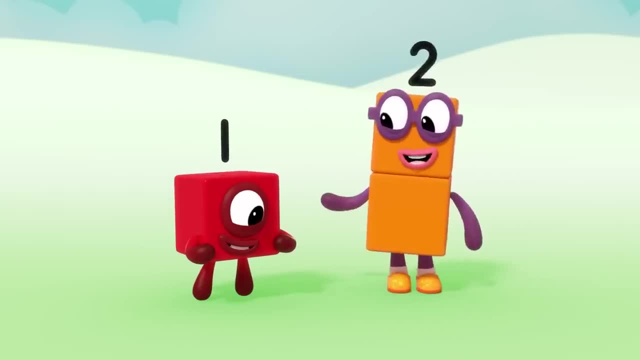 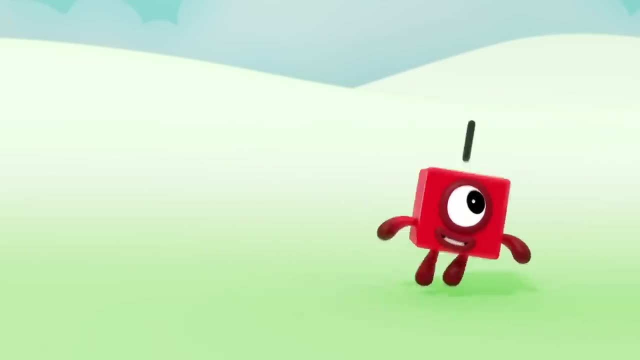 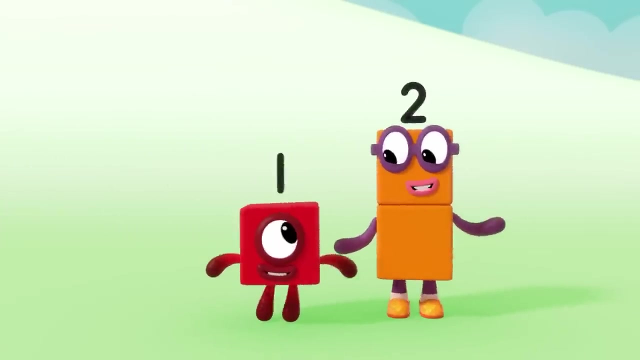 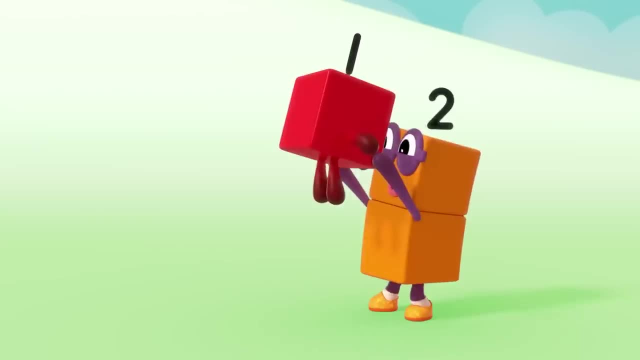 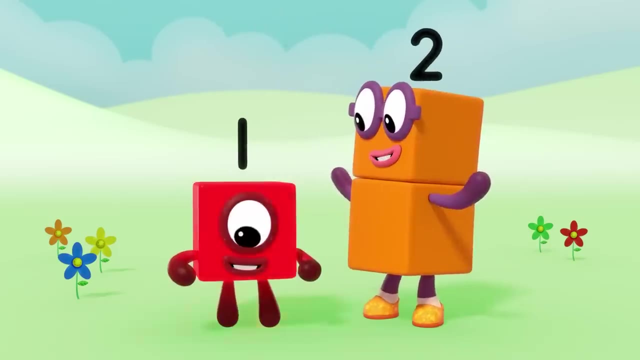 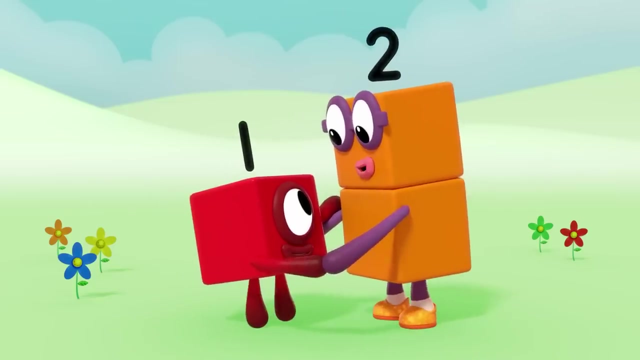 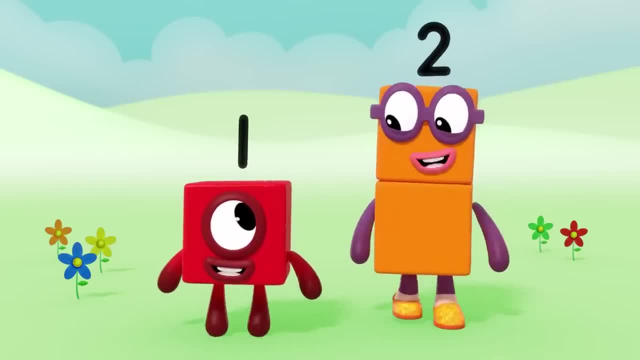 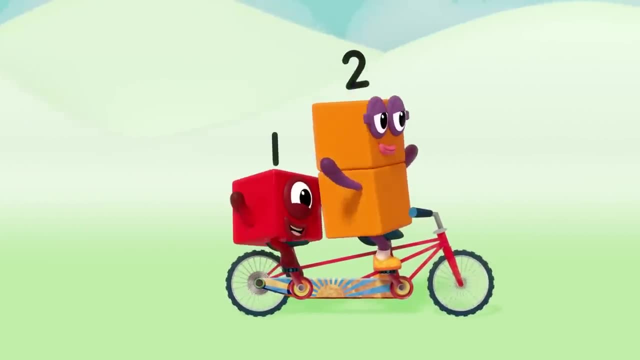 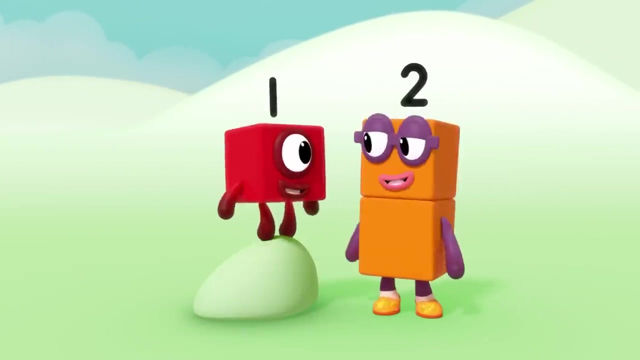 With one you can do the hop One One. With two, you can learn a new step And be spun right round like a spinning top. With two, you can ride a tandem, But you haven't seen anything yet. With two, you can give a piggyback. 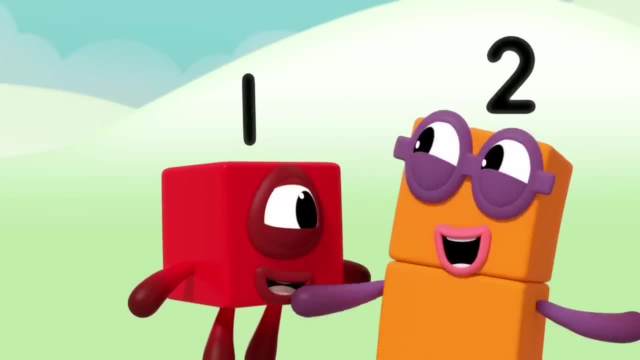 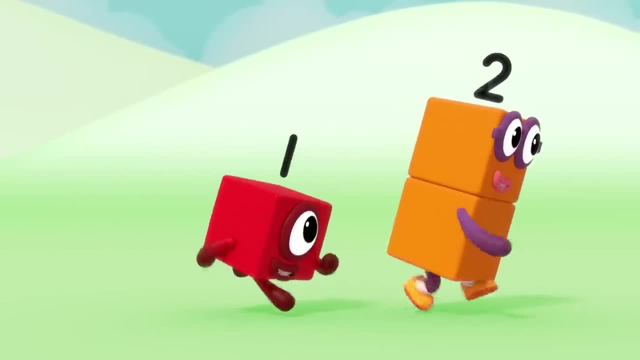 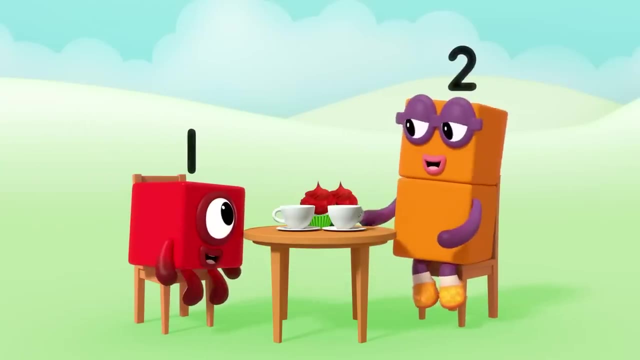 With two, you can sing a duet: Na na na, Na na na. Everything is better with two, The two of us together, just me, and you. Imagine all the crazy things we can do with two. With two, 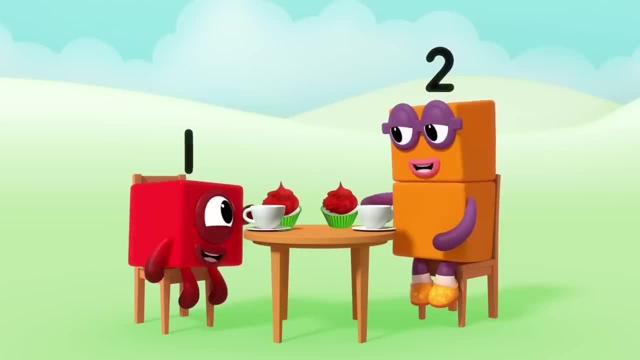 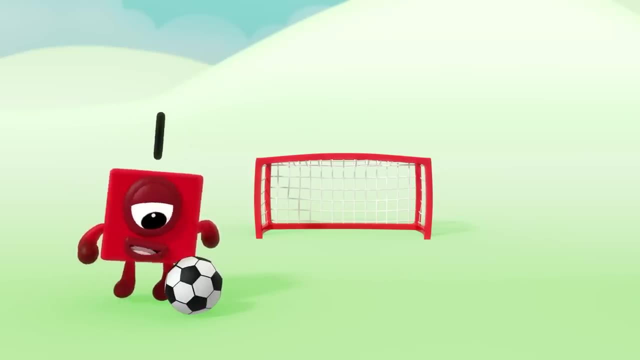 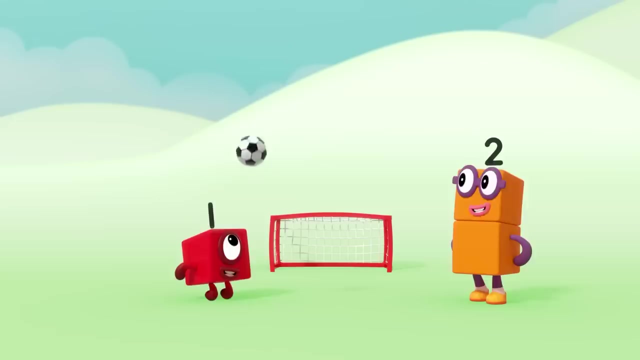 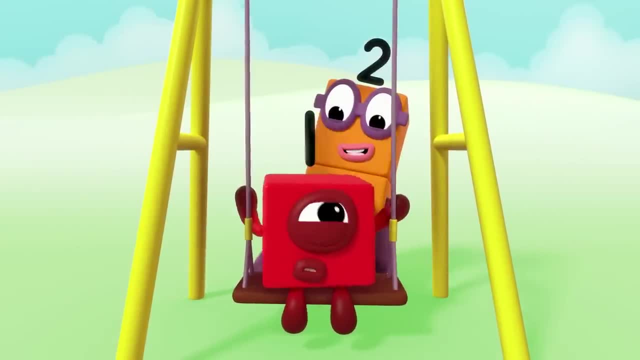 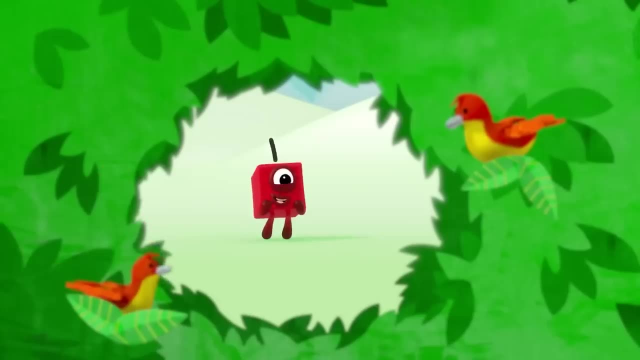 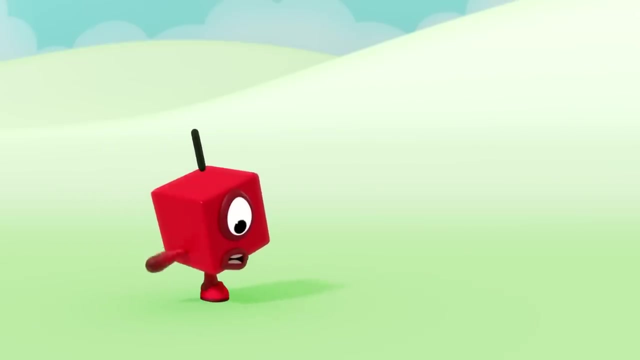 With one, the swings are boring, Cause you need a friend to give you a push. With one, you can get a bird in the hand. Oh look, there's two in the bush. One shoe just won't do. You'll end up all lopsided. 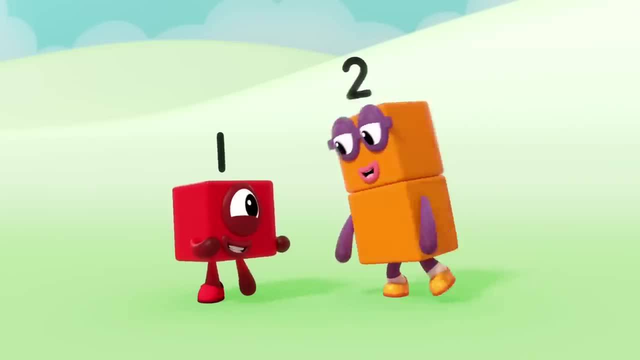 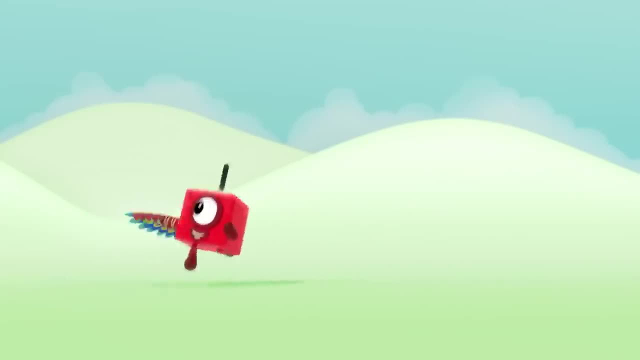 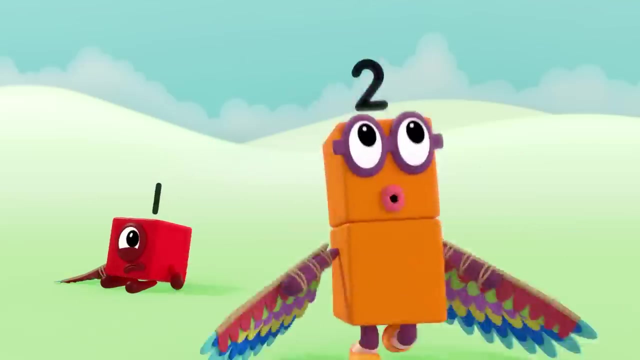 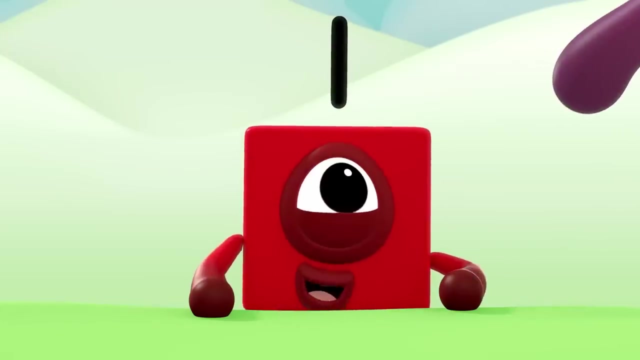 One, two, two shoes You can use to dance, Just like I did. One wing tied with string, No point even trying. One, two, Two wings and zing, You'll soon be flying. With two, you can get a leg up. 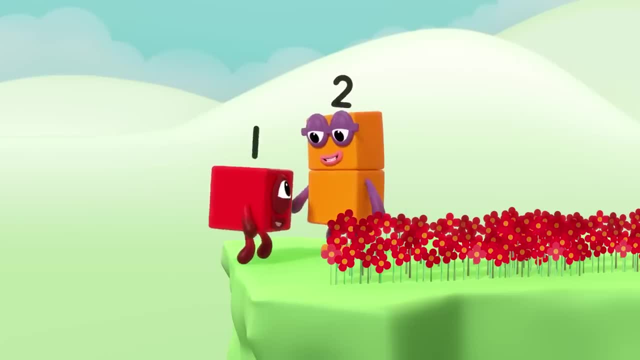 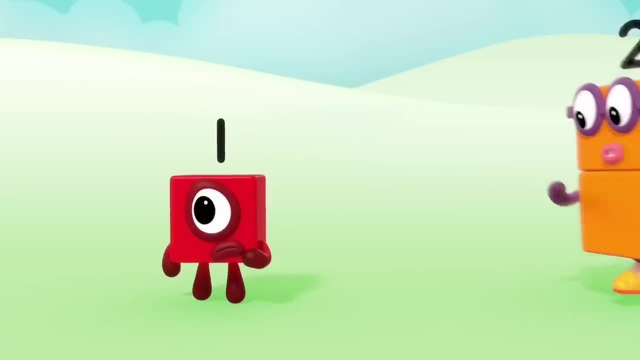 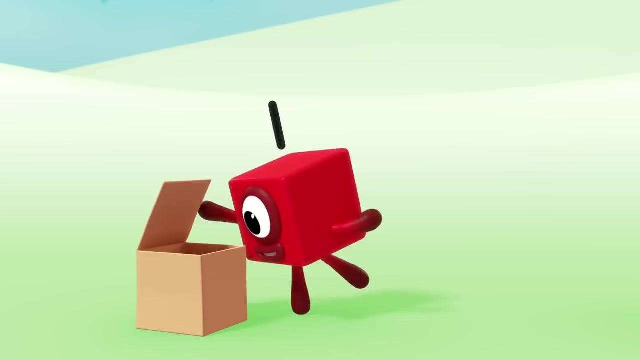 With two, you can offer a hand. With two, you'll never be fed up, Cause there's always someone to understand. With two, you won't be lonely and you're never going to have to pretend. With two, you can play hide and seek. 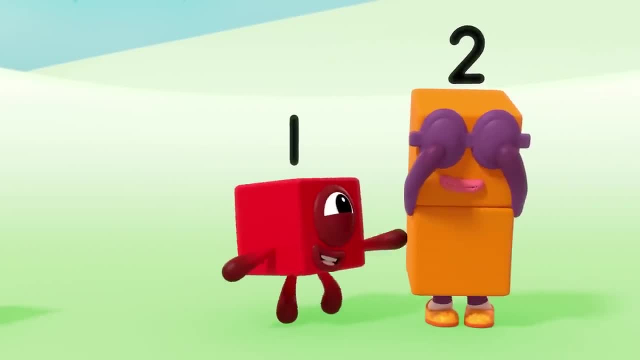 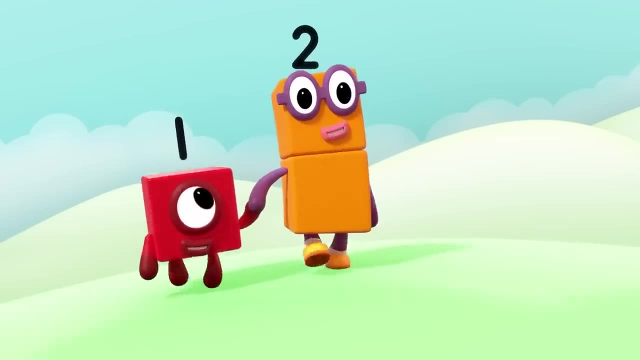 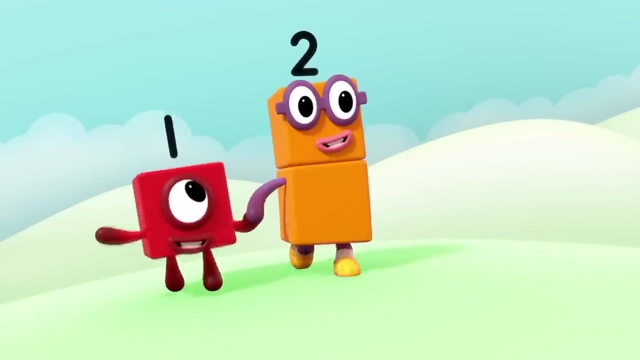 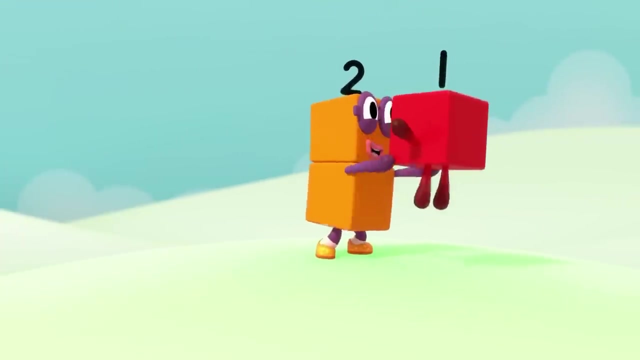 With two you can find a best friend, Because everything is better with two, The two of us together, just me and you. Imagine all the crazy things we can do with two. with two, With you and me and me and you, with two, we'll see what fun can be. 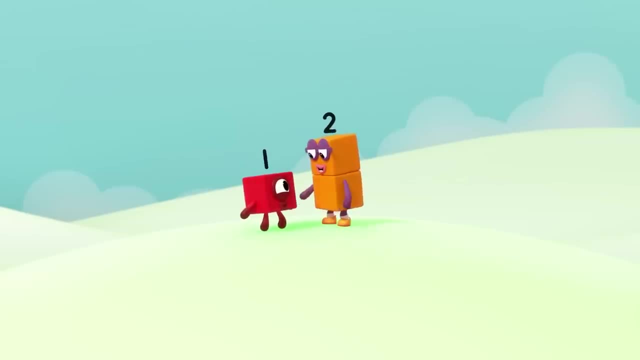 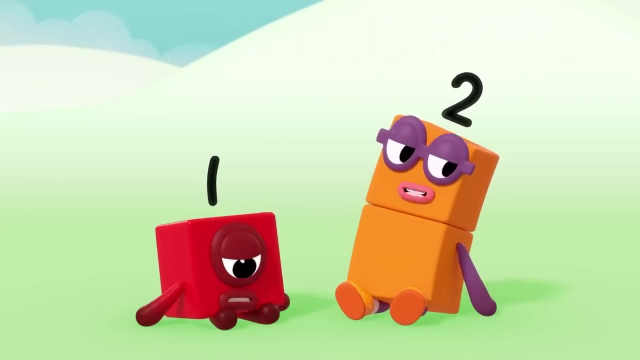 With you and me, and me and you, and all the things we can do with two Best friend, Best friend One two. what shall we do? One two: what shall we do? One two want to see a trick. 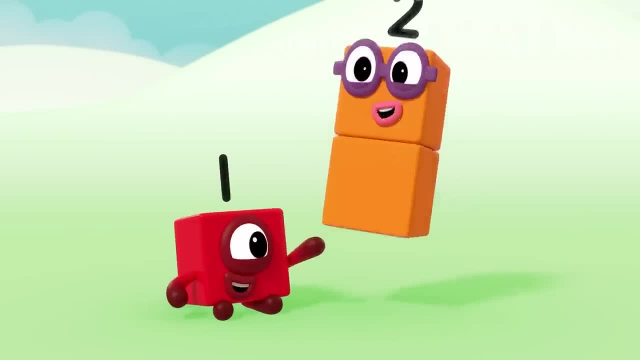 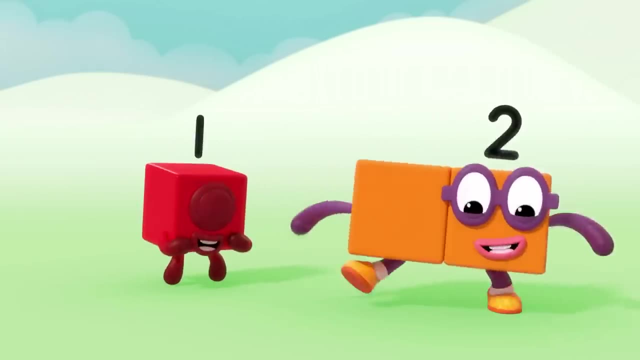 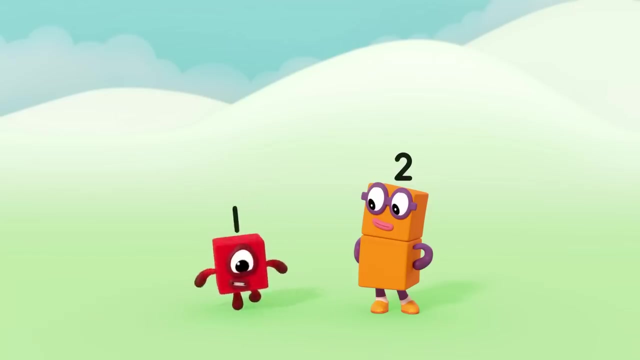 Yes, Tap me Two. are you okay? Your turn? I can hop One one one. one, Two Plus one Equals three. I am three. Look at me. One, two, three, Three juggling balls. 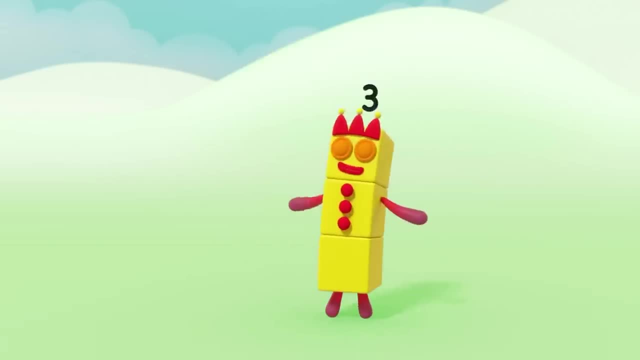 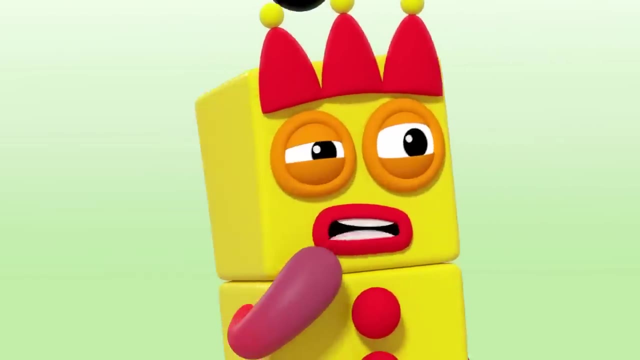 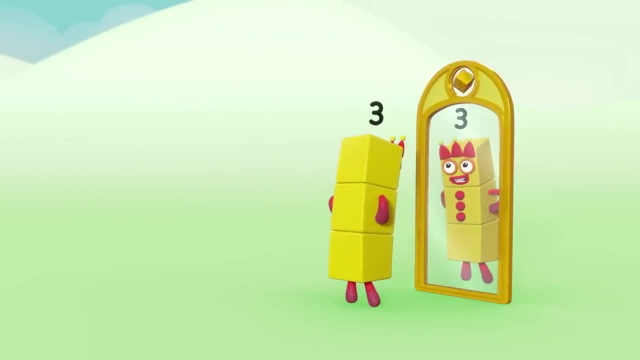 One, two, three. Thank you, Thank you, Thank you, Where did they go? Where's my audience? One, two, Three. I like what I see. Take it away three. Three minus one Equals two, My audience. 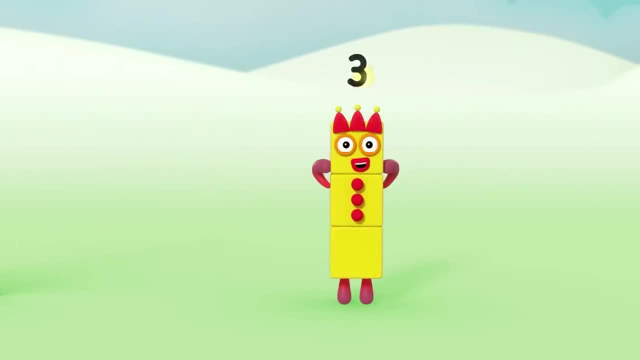 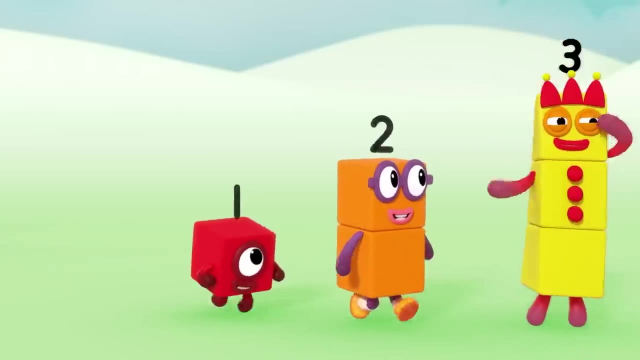 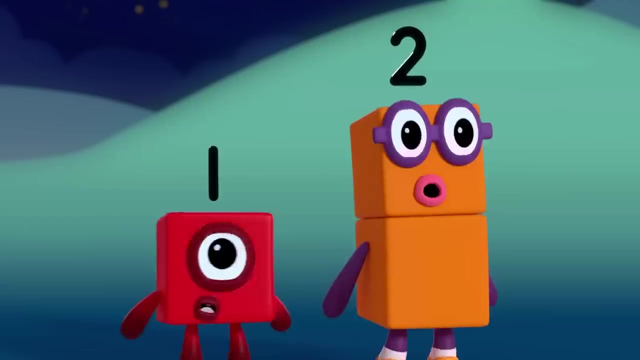 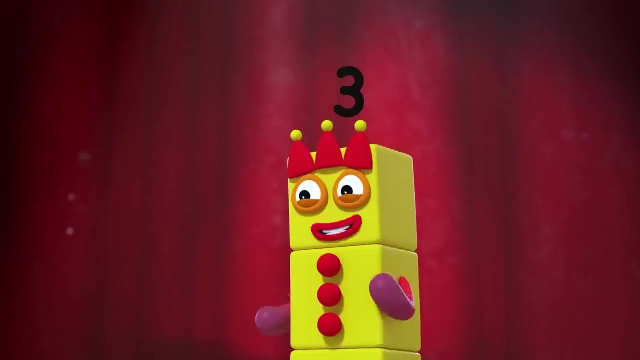 That's better Ready. One, two, three. One, two, three. Everybody. look at me. I'm here to entertain you with this funky melody. I'll juggle three balls as I dance and dance. I don't have to do the arm wrestling, except she does. 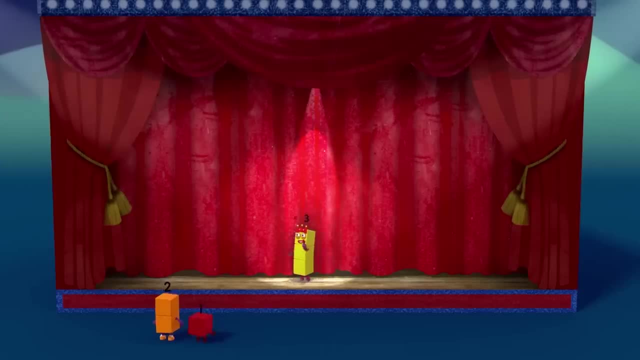 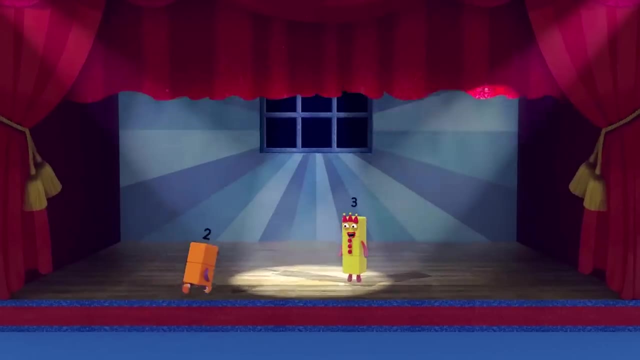 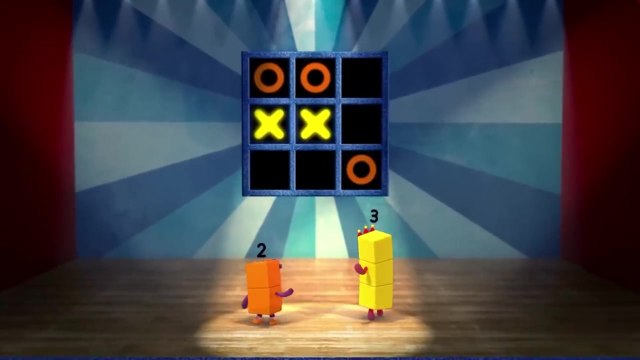 in the air and everyone will cheer. everything's gonna be all right now. number three is here. i'm in tic-tac-toe, i'm in, ready, steady go. you're gonna have to count to three to get three in a row. you'll find me hiding everywhere you look in a fairy tale or a picture book. 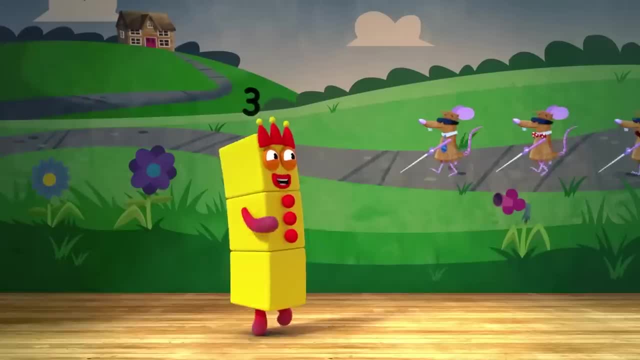 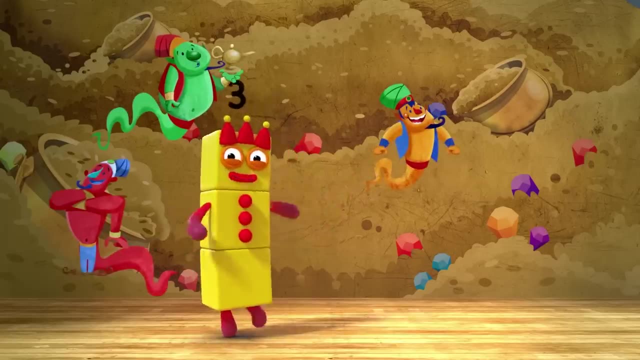 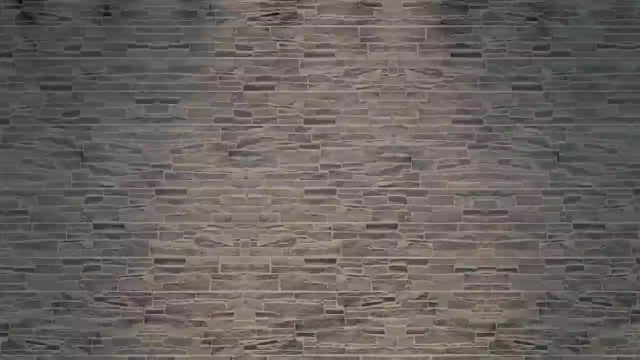 one, two, three. can't you see i'm in? three blind mice, three wishes would be nice. you should try and try and try again. that's my advice. goldilocks came across three bears, one, two, three, three balls, three chairs, three beds upstairs. i'm here, i'm there, i'm everywhere. 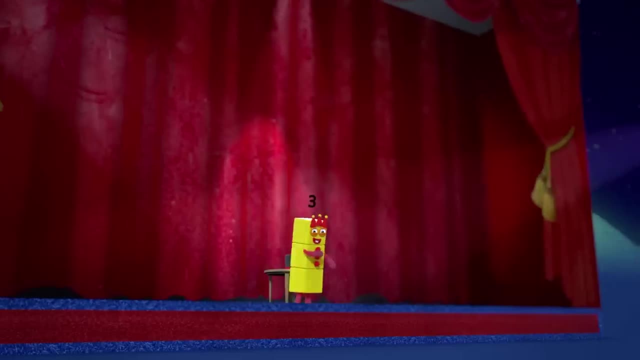 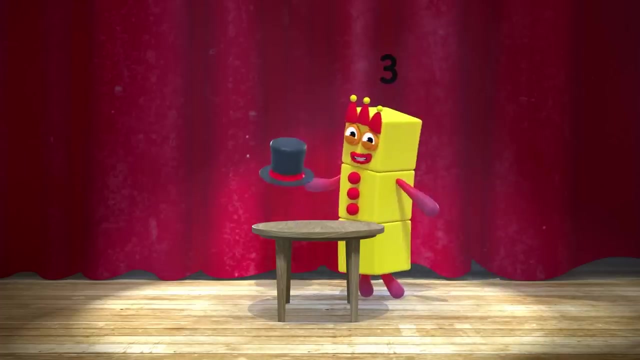 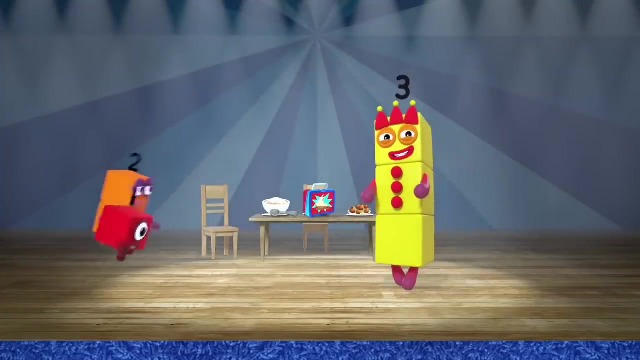 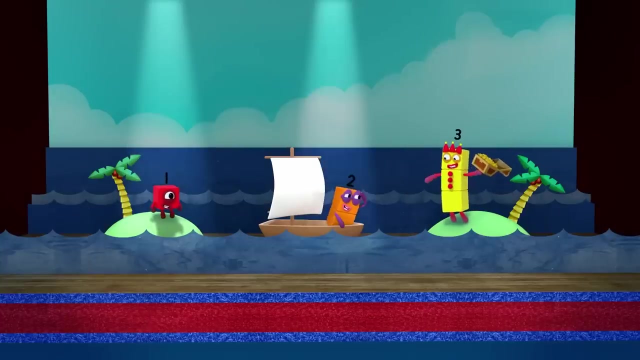 one, two, three, everybody. look at me, i'm here to entertain you with this funky melody. i'll pull three rabbits from a hat and make them disappear. everything's gonna be all right. now number three is here. three meals a day, three sections in a play: beginning, middle and an end. that's the only way. 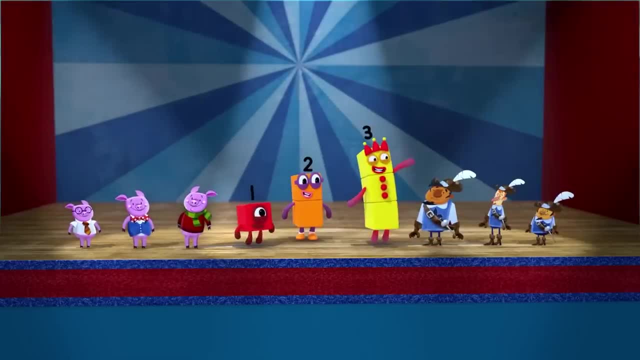 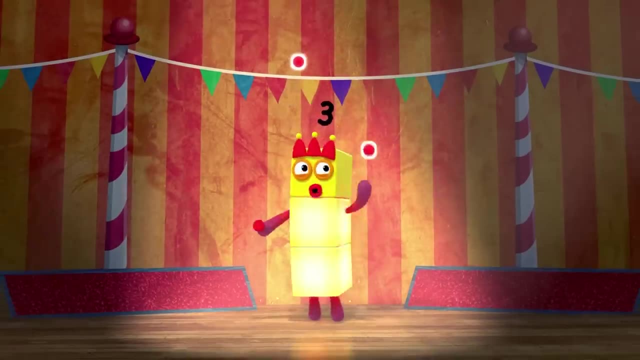 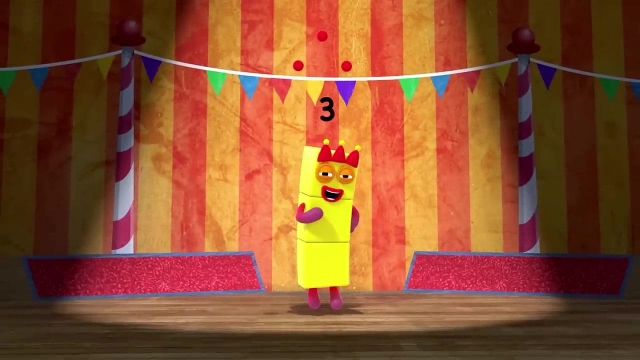 everybody. better give three cheers, three little pigs, three musketeers. one, two, three, stop. you see, i can keep three balls up in the air: one, two, three. sometimes they get stuck up there. one, two, three. the juggling balls can be your guides: one, two, three to make a shape that's got. 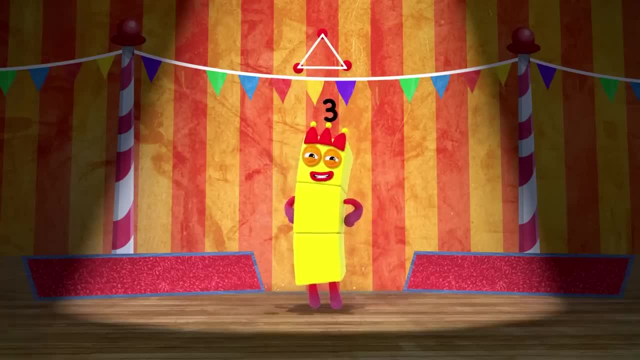 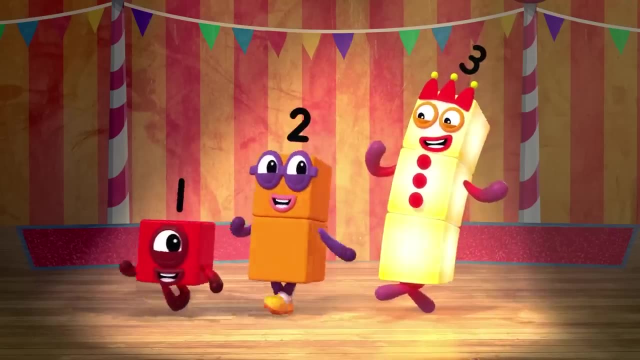 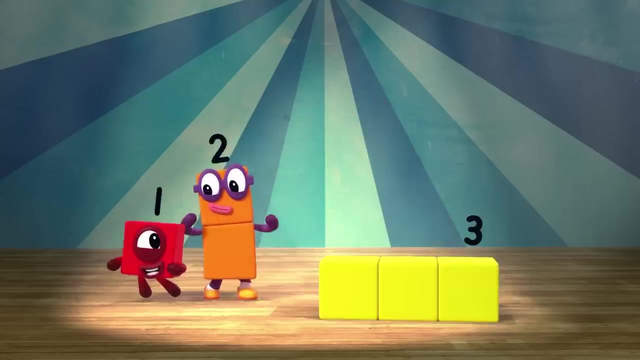 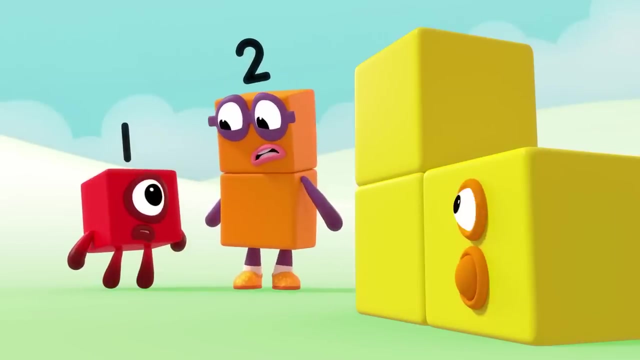 three sides: one, two, three. do you know what it is? bingo, it's a triangle. one, two, three. everybody look at me. i'm here to entertain you with this funky melody, with jokes and jigs and throwing shapes. i take it off the gear. oh no, i've broken three. everything's gonna be all right. i'm three and i'm 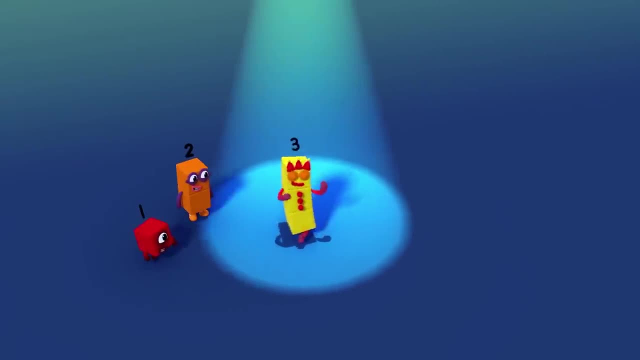 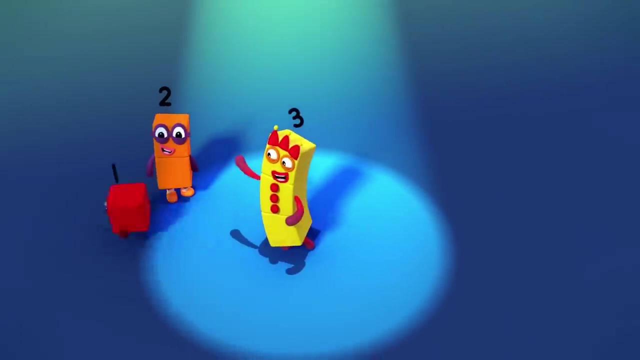 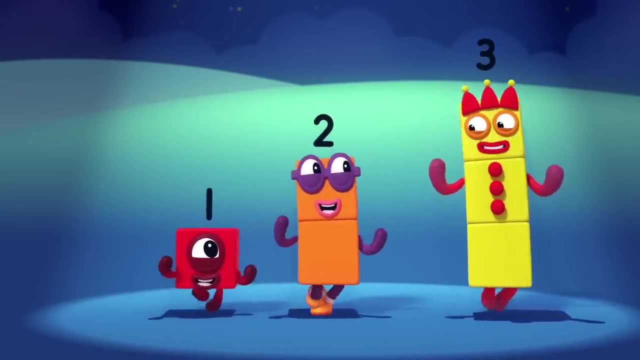 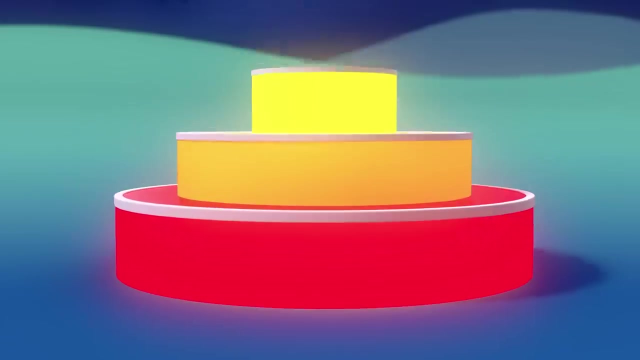 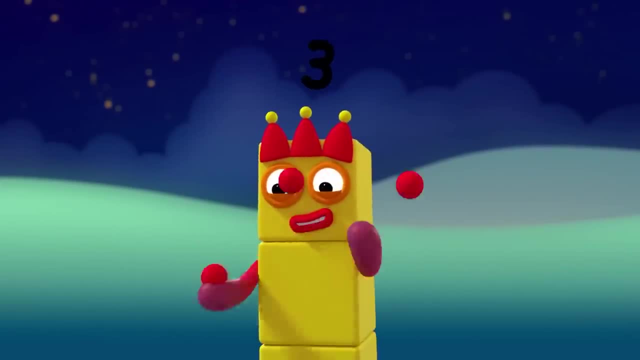 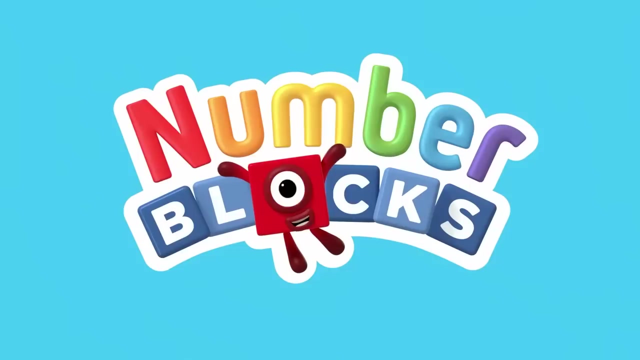 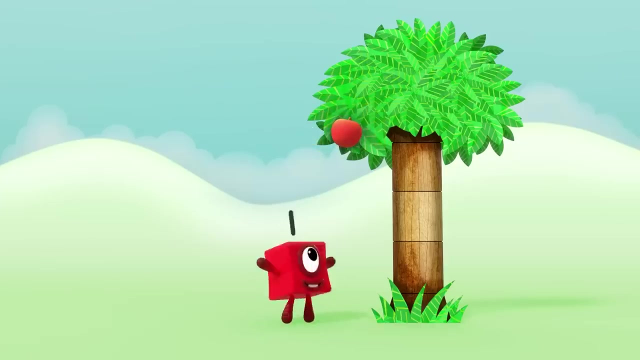 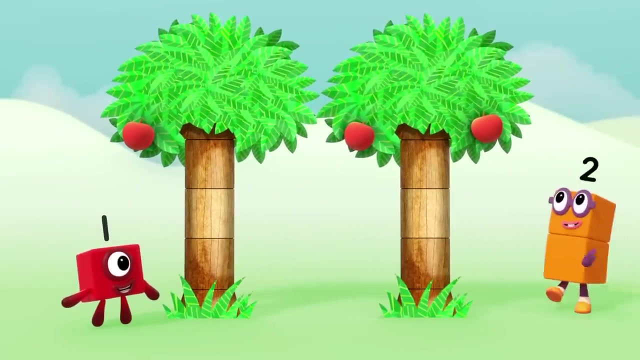 melody: i'll juggle three balls in the air and everyone will cheer. everything's gonna be all right now. number three is here. everything's gonna be all right now. number three is here. one, one apple, yum, oh two, one, two, one, two, one, two, oh one, two, two apples. 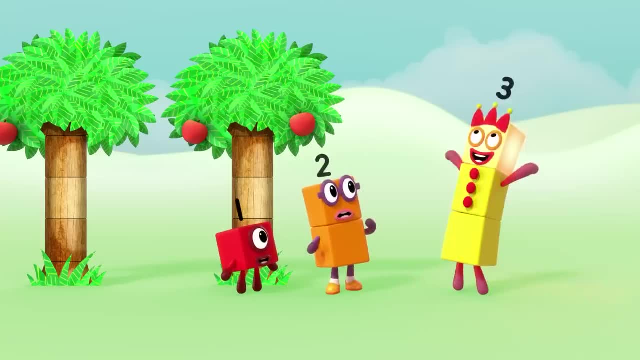 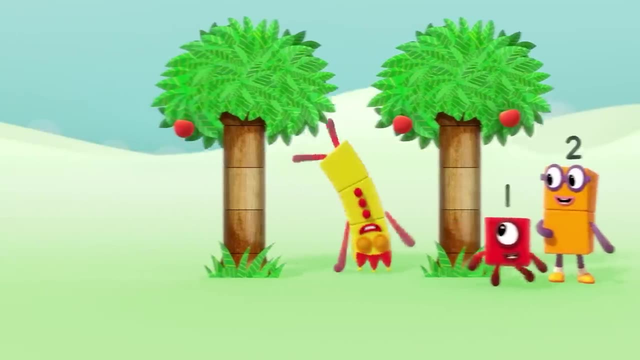 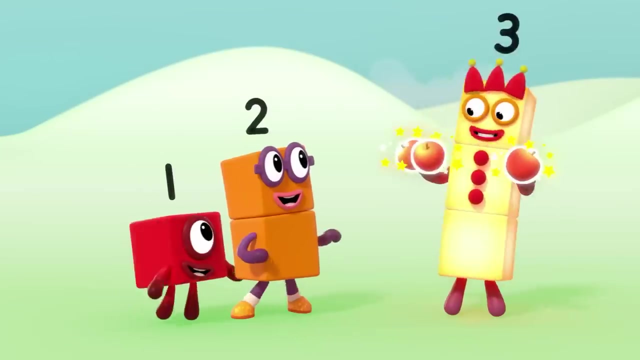 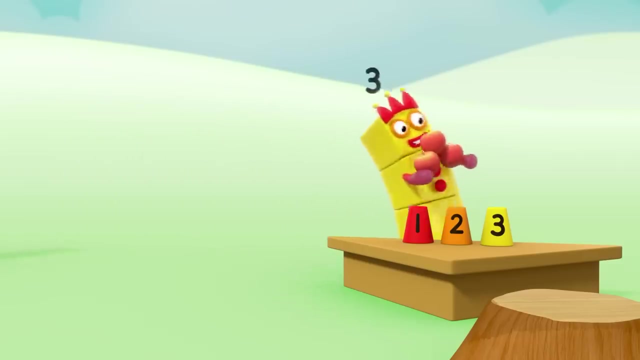 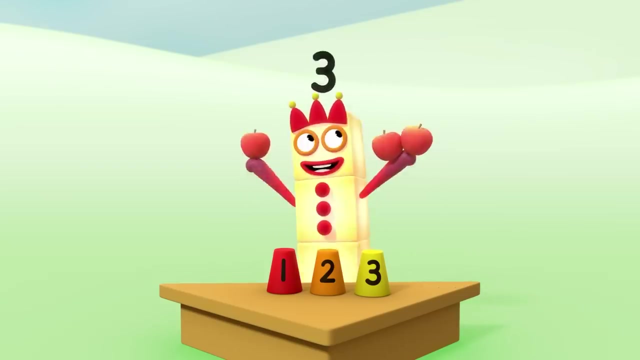 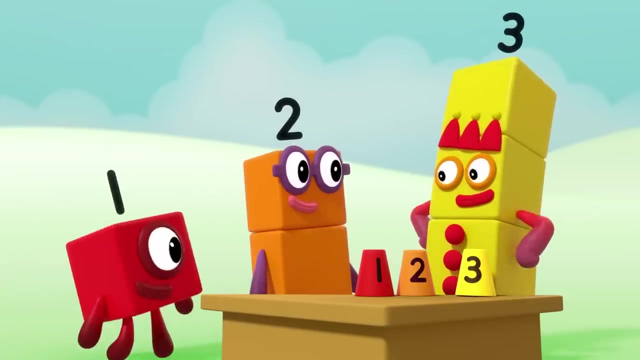 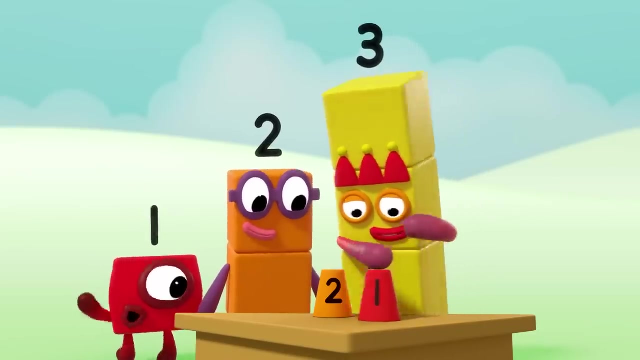 we're both too small. three, look at me, i'm big enough to reach. you see, one, two, three, three apples, oh, three, you see, come with me. the show is just beginning. let me show you a trick or two or three. let's play. find the apple. round and round and round, round and round and round. 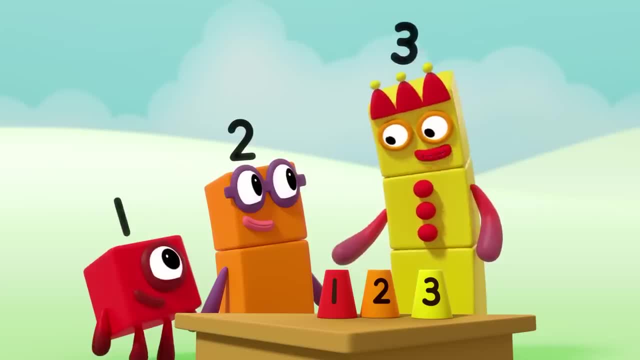 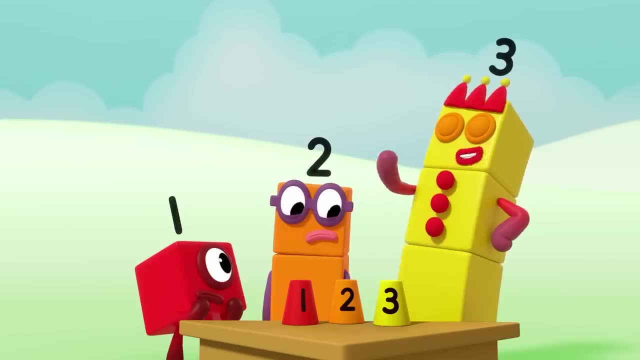 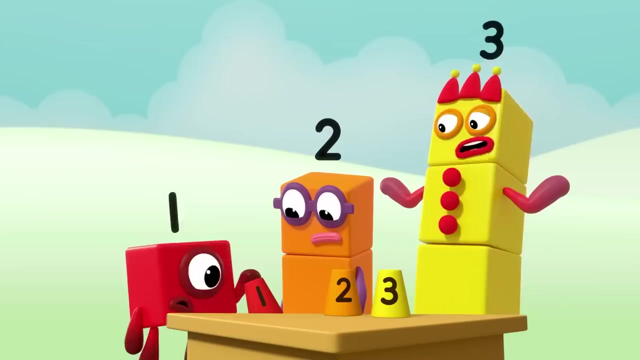 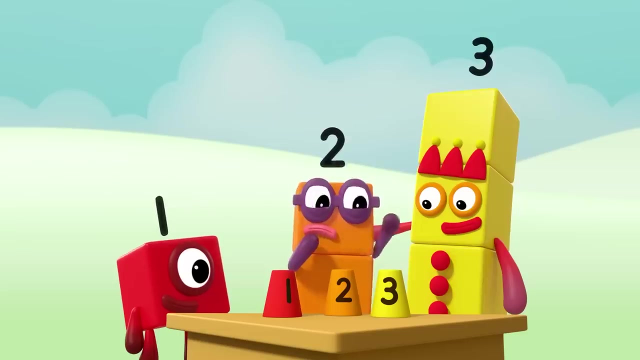 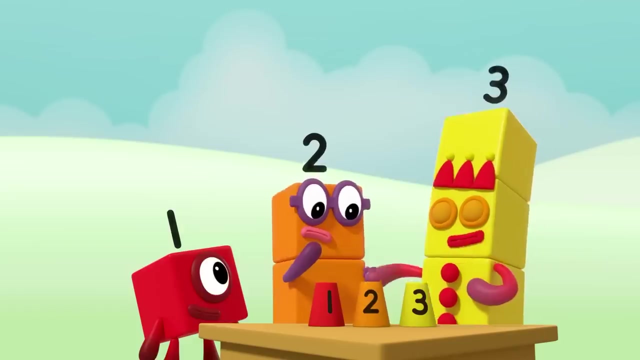 ready, steady stop. so which cup is the apple under? one, you're the first number, so you can have first guess this. one, the first cup? oh, bad luck. one. two: you're the second number, so you get second. go this, no, that, oh. oh, Like this, good luck. 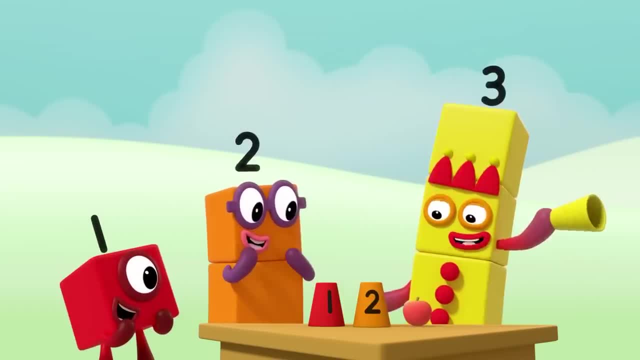 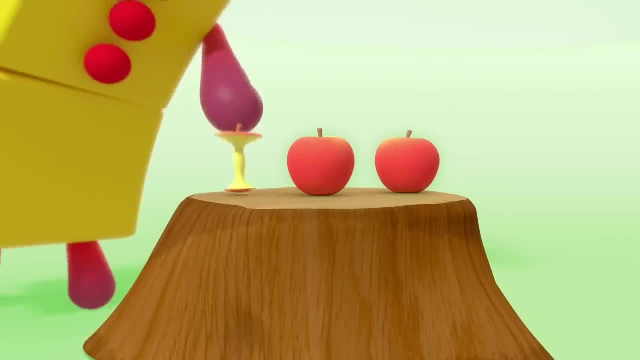 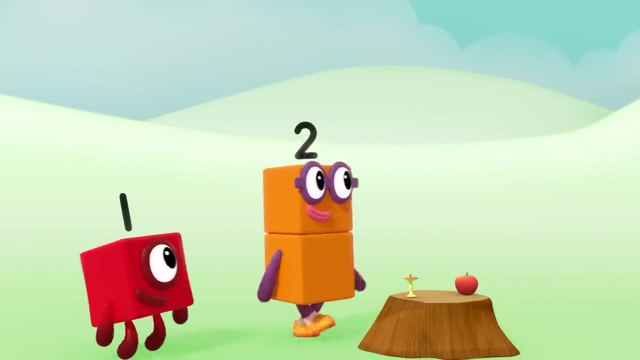 let me have third one. so how you guys feeling it's going to be利, you will be getting that happy juice. yep, i'm reaching cars. 3 is the third number. add one, two, three, i've got my own little jar. um, all we got is a little time. 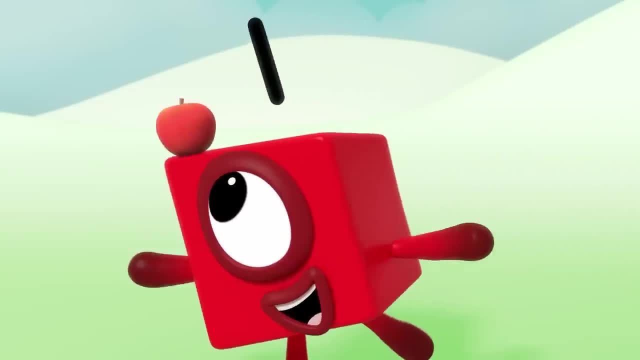 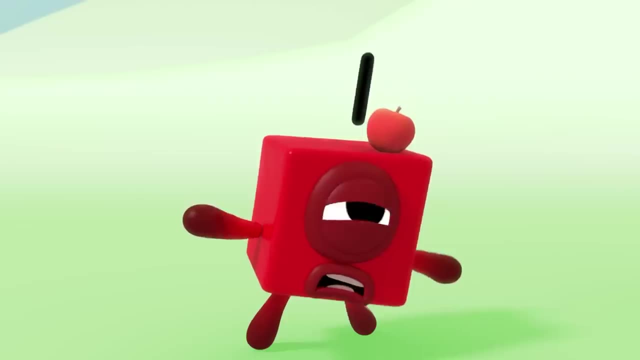 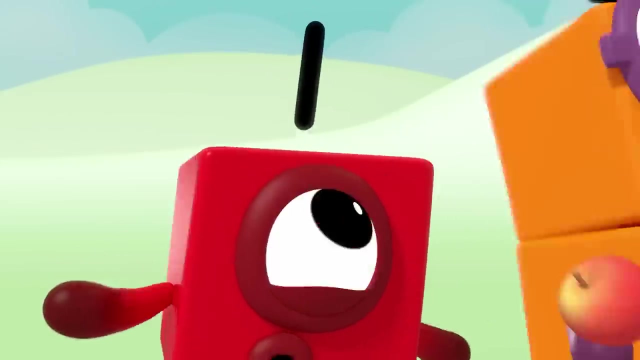 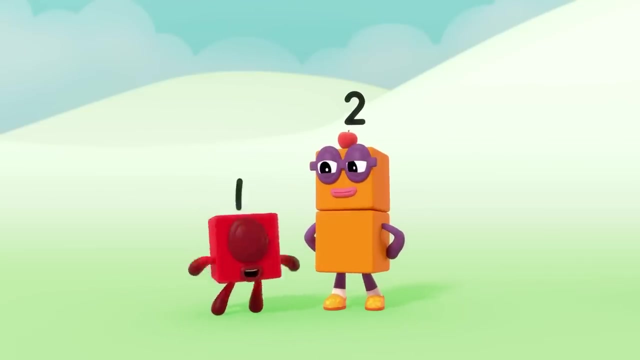 his: oh, let's win. well done, Simple rules. Apple on top, don't let it drop. Now try and swap. Hey, I can't reach. I'm smaller than you. I'm the smallest number, Then I'm bound to win. I'm bigger than you. 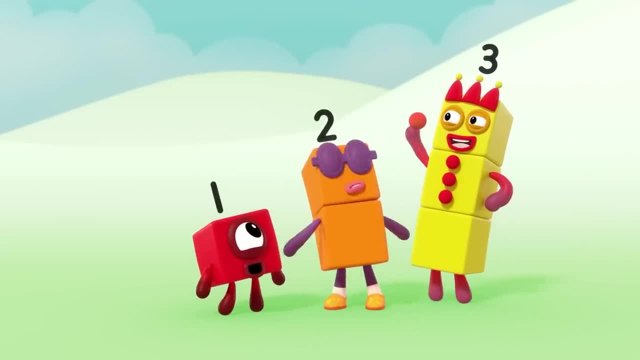 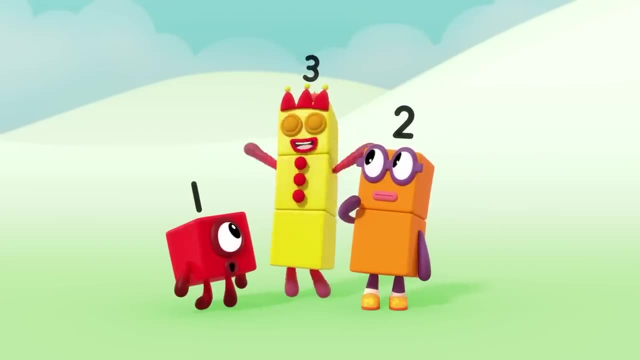 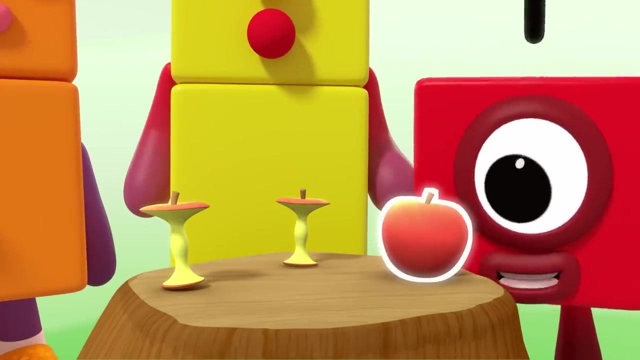 Oops, Silly me. I'm bigger than one, but smaller than three. I'm bigger than both of you, I'm the biggest. So I guess I win again. One, two, three, Two apples gone, One apple left. Surprise, It's the final game. 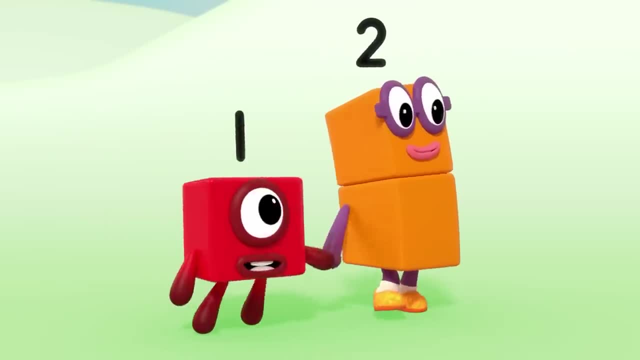 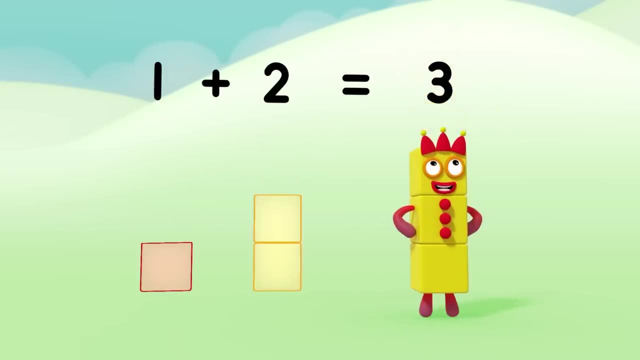 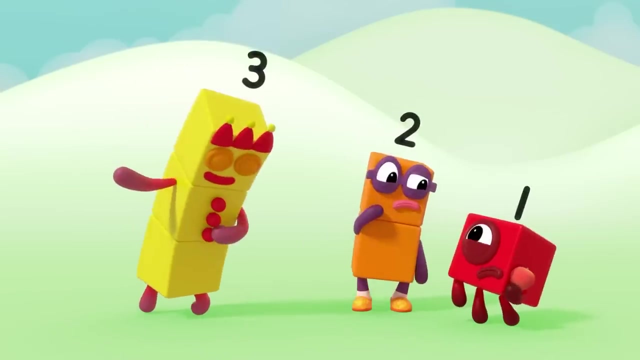 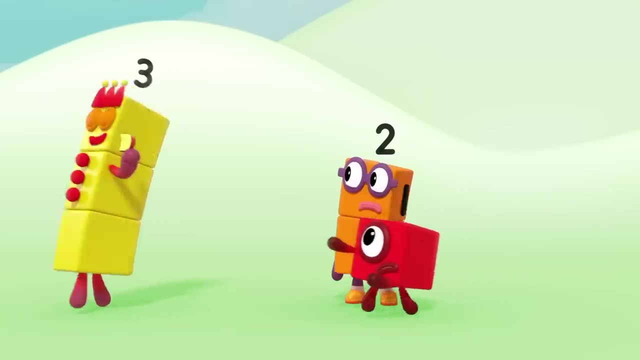 The biggest surprise wins: One plus two equals three. One, two, three, Three equals two plus one. Wow, But how Very good. You win best surprise Three. One, two, three, All for me. Oh, that was the last one. 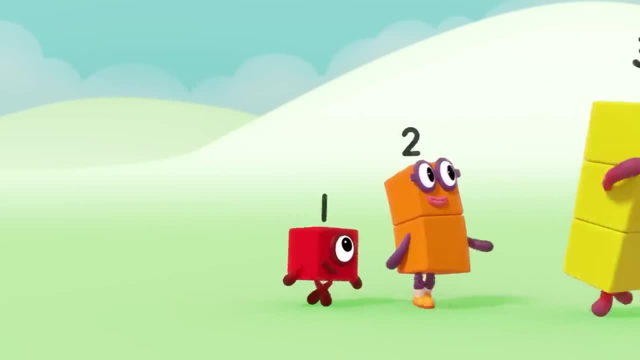 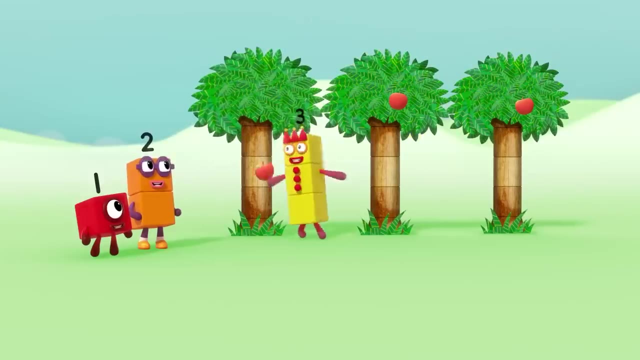 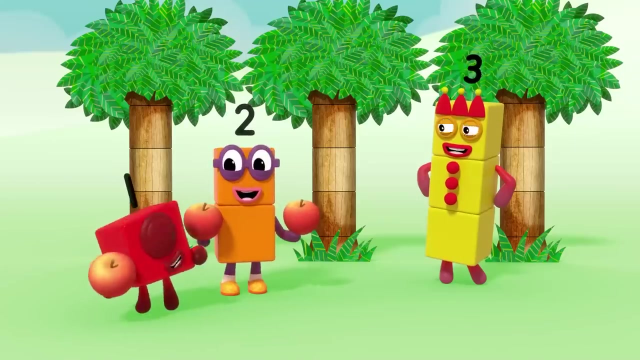 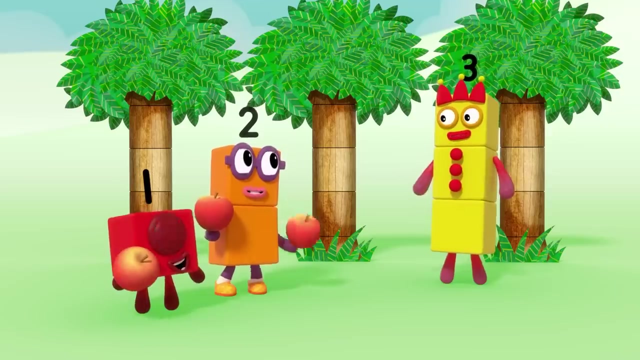 Don't be sad, Don't be mad, Be glad. One, two, three, Three trees with one. One, two, three, Three apples, One for me And two for me. I've already eaten three, I don't mind sharing. 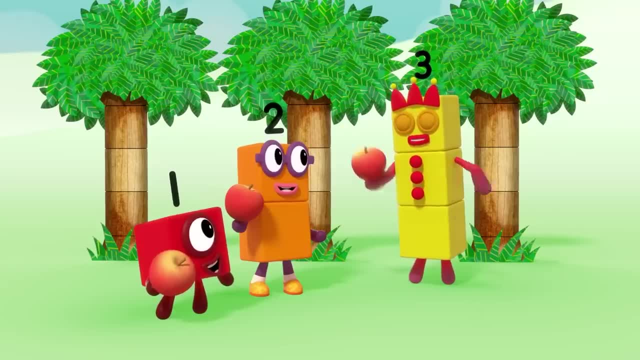 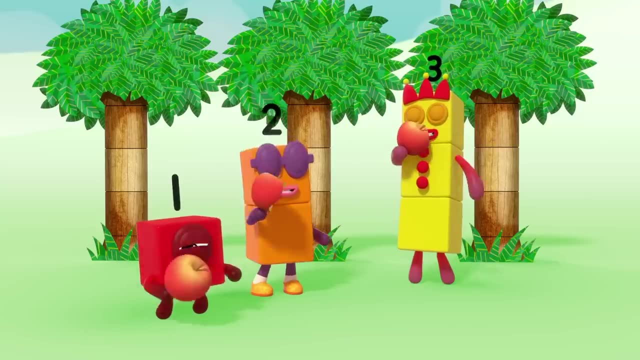 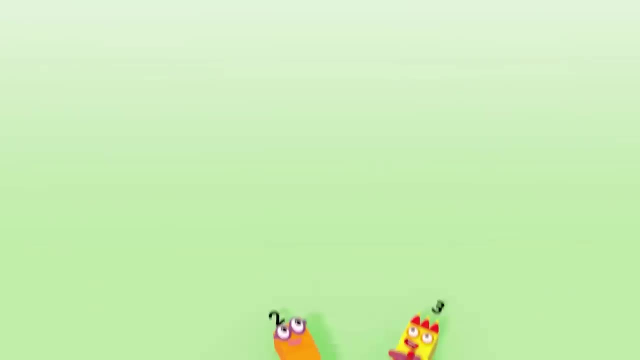 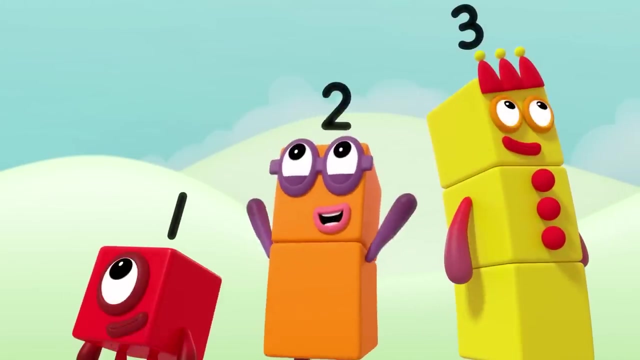 Thank you two. Now for my final trick. Let's make these apples vanish. One, two, three. One, two, three, Three apples. Oh I know, One, two, three, Three apples. One, two, three, Three apples. 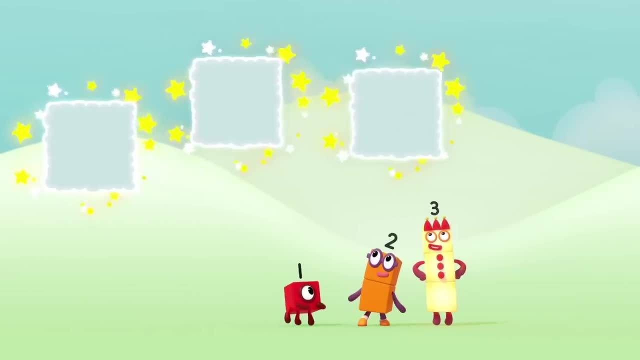 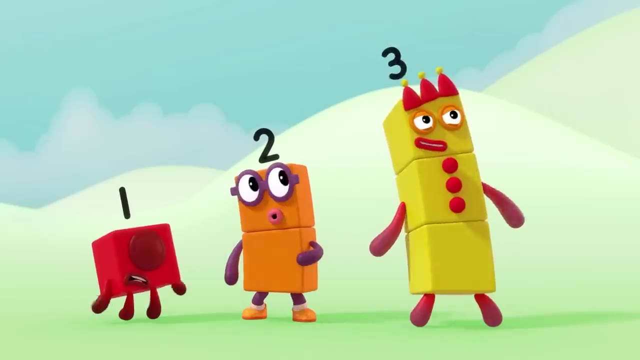 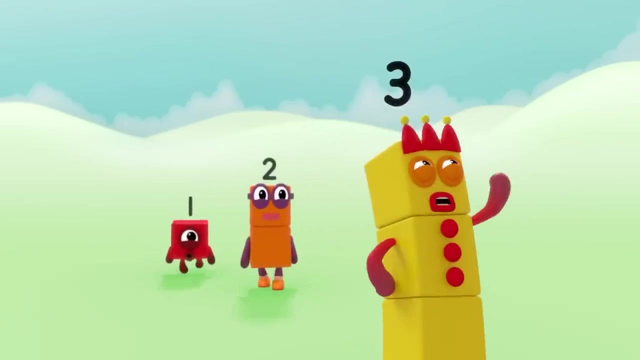 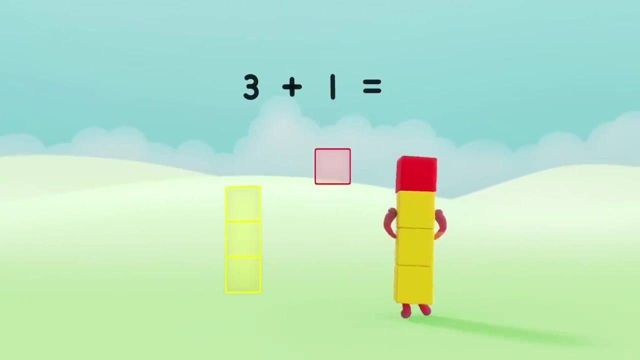 Only one. One, two, three, Three apples. No one cakes apples. We need to get rid of that. one, One, two, three. No one's bigger than me. Three plus one equals Four. I am four. I'm one more. 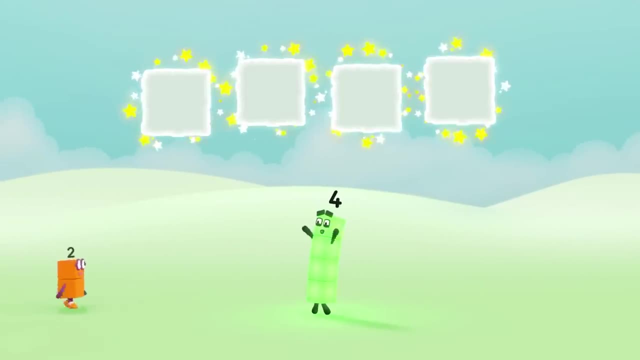 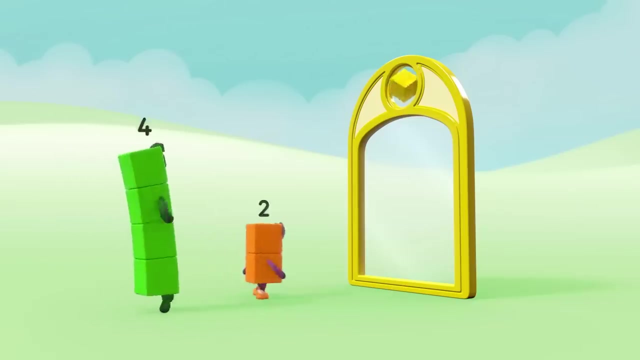 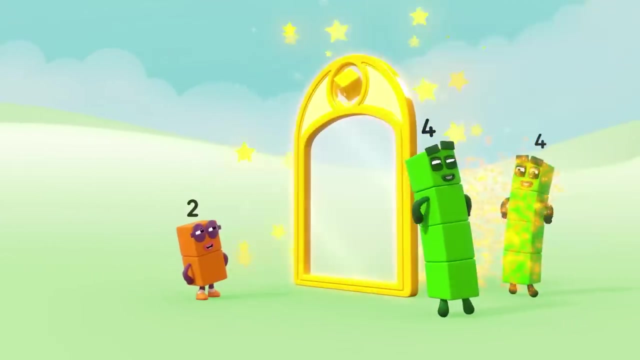 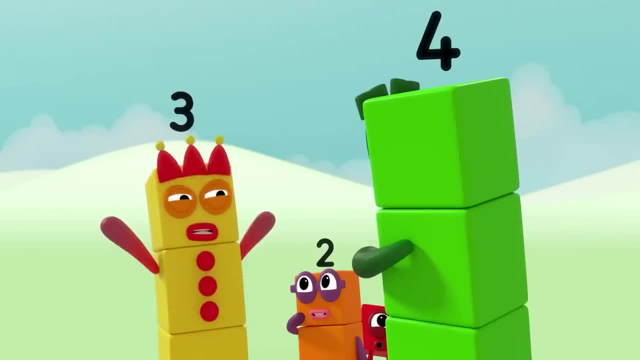 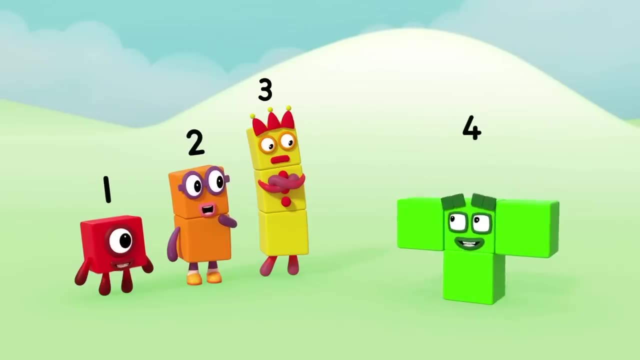 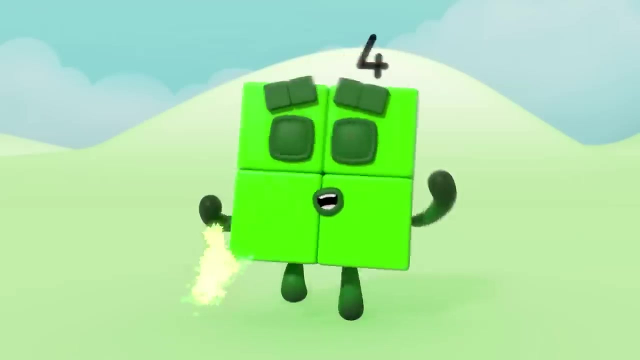 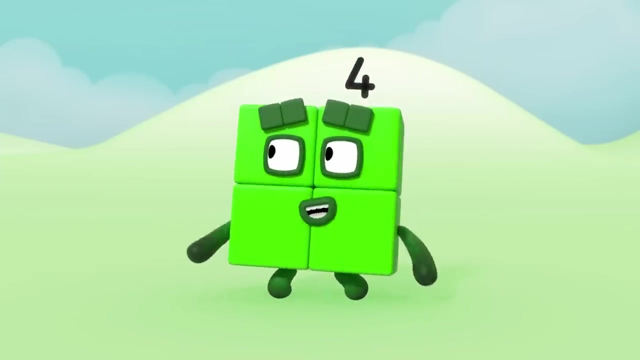 This won't do. I'm three, I want to be the biggest. Oh Oh, I can be shorter, That's much better. Oh yeah, I am square. What's so special about being square? I'm so glad you asked. 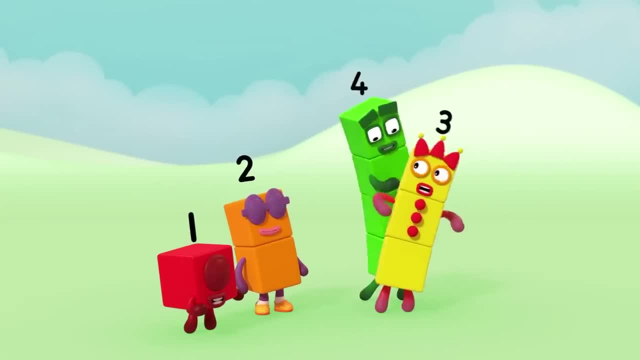 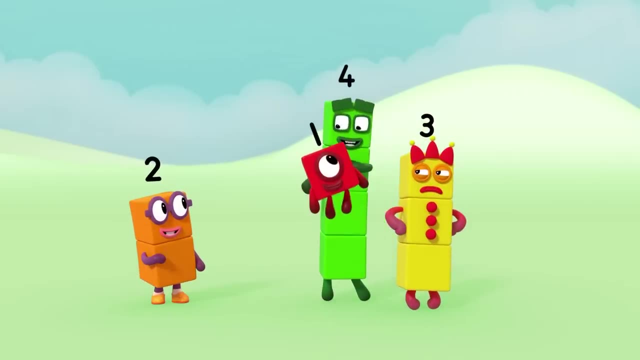 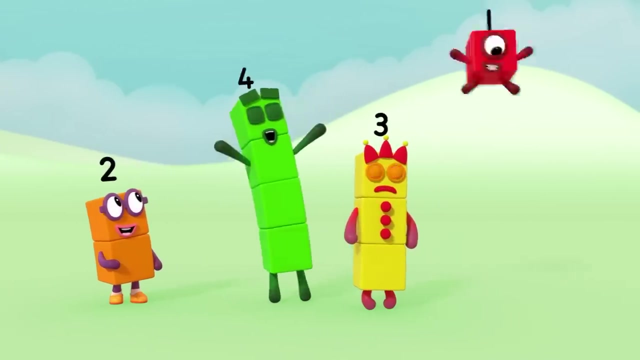 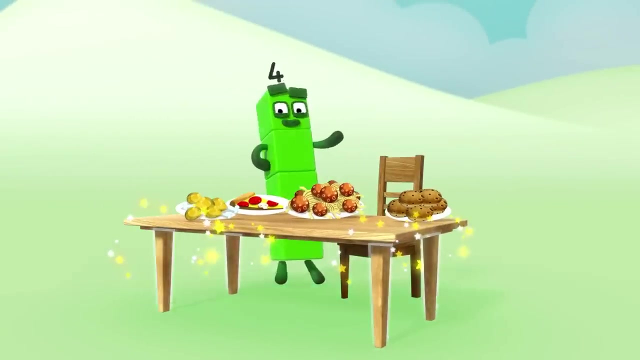 I'm four. Have you met me before? I'm one more than three. That's plain to see. Three plus one equals me. I'm four. One, two, three, four. Four legs on a table: One, two, three, four. 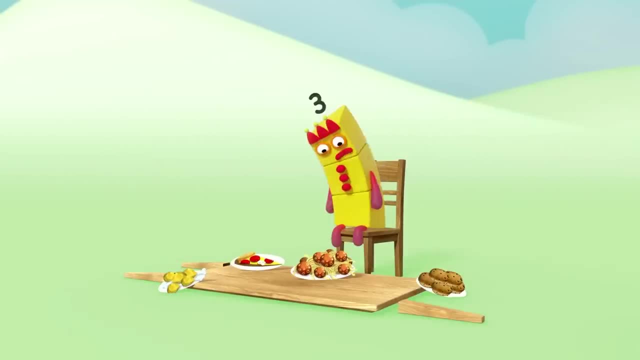 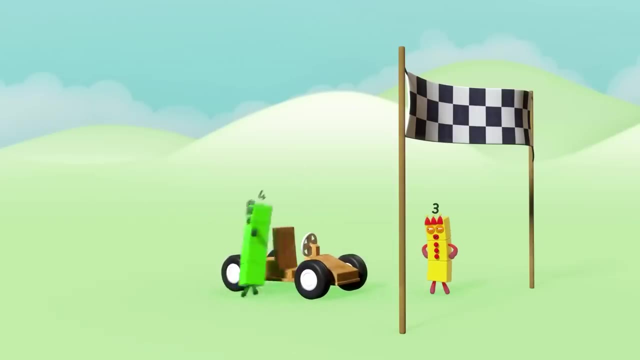 Four legs make the table more stable. Oh, One, two, three, four, Four wheels on a go-kart. Without four wheels, you no go-go-kart. We'll be stuck right back at the station. Yeah, No, I can't. 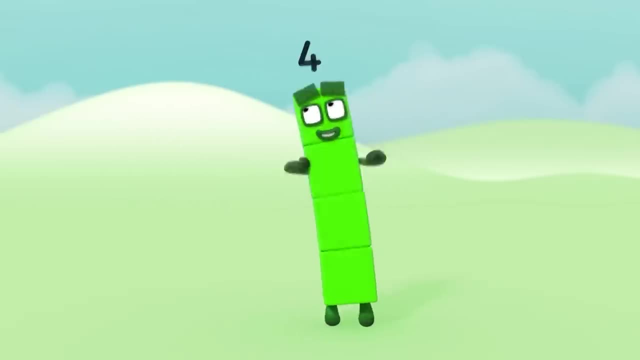 I'm four. Look at the start. I'm four. Have you met me before? I'm four. I'm four. One more than three. That's plain to see. Three plus one equals me. I'm four. One T-h-e-e-e. 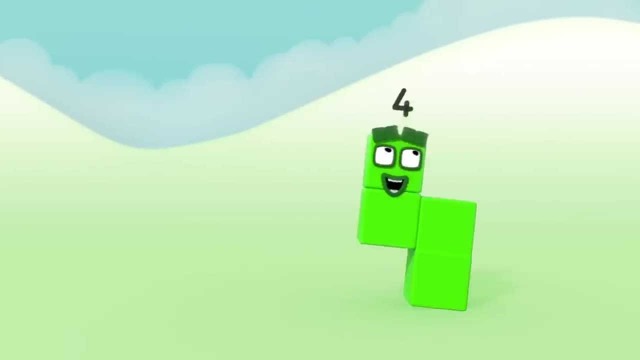 E-e-e, f shades T-h-e-e. The best shape of all is stout and strong. What shape is this, can't you tell? I like to be square. I like to see square things everywhere. Anywhere there's a square, You'll find me right there. 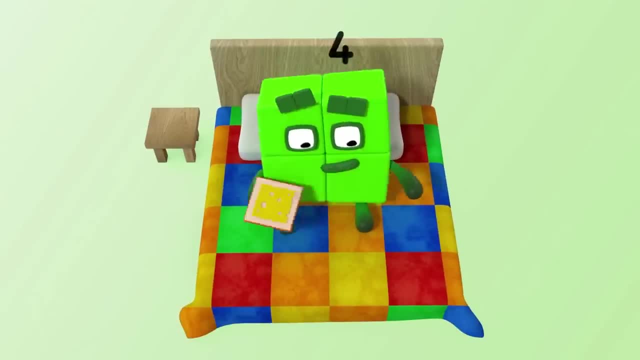 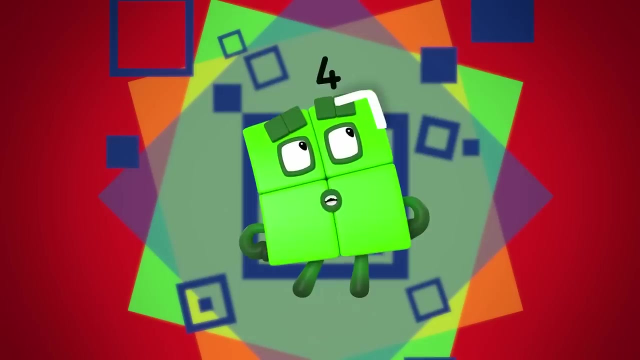 Square cheese on square bread Square, quill on a square bed. Square is where it's at. Of that you can be sure. Anywhere there's a square You'll find more. One, two, three, four, Four sides. One, two, three, four, Four corners. 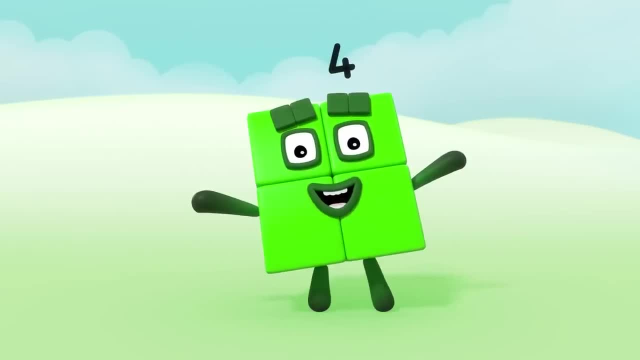 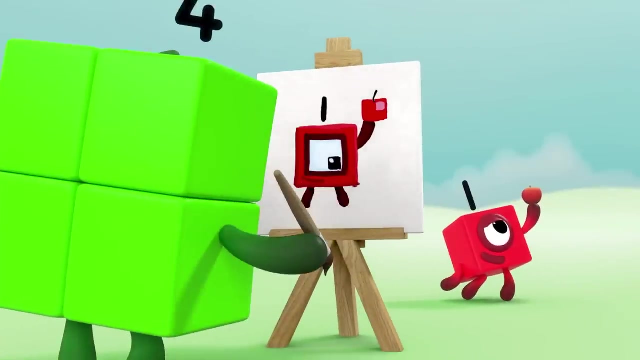 Square is the shape for me. It has four corners and four sides. you see, When four blocks make one big block, I'm solid as a rock. I like to be square. I like to see square things everywhere. Anywhere there's a square, You'll find me right there. 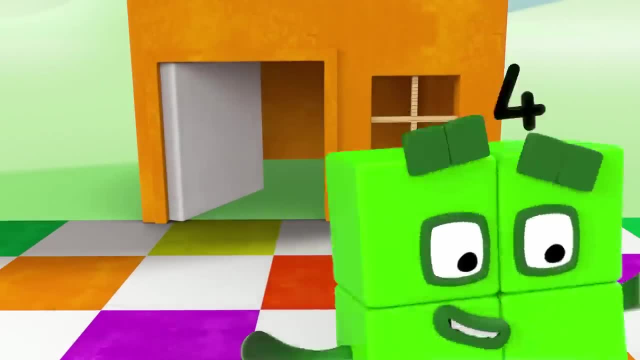 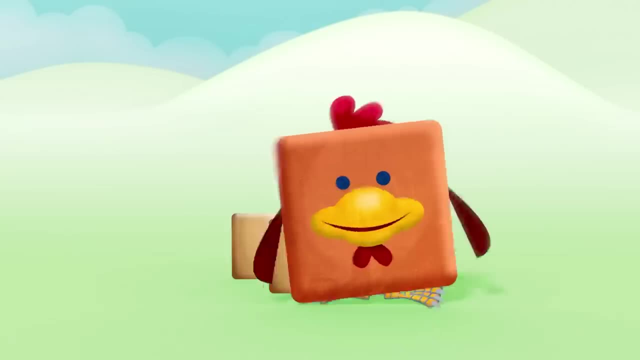 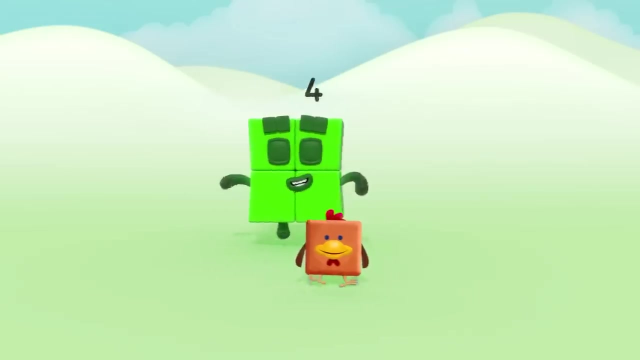 Square window, square door, Square tiles on a square floor, Square sun, square, clouds Square flowers and square cows. The square oath for, square pets, Square chickens and square eggs Square is where it's at. Of that you can be sure. Anywhere there's a square You'll find four. 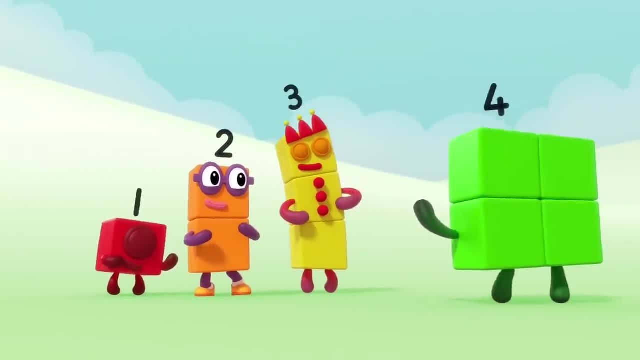 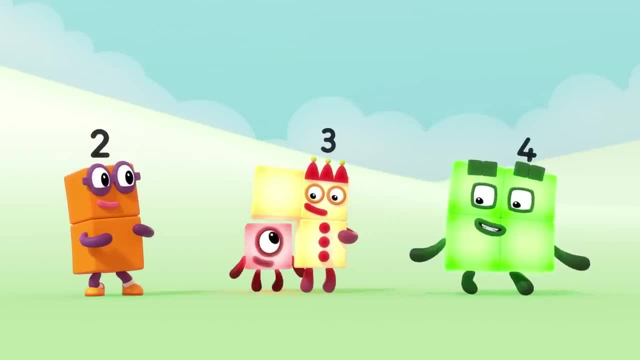 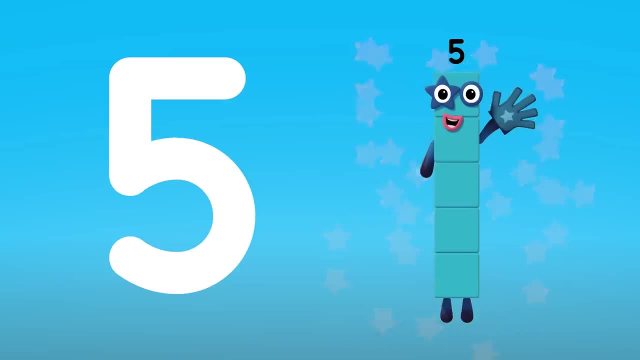 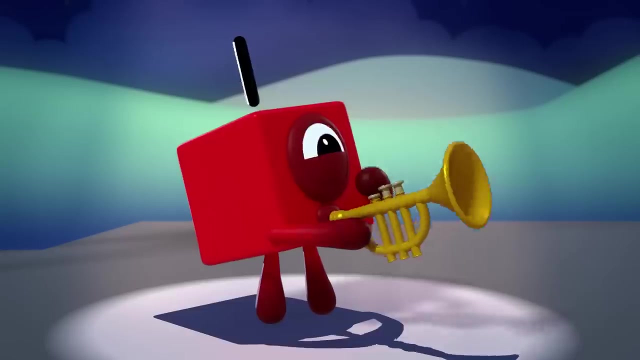 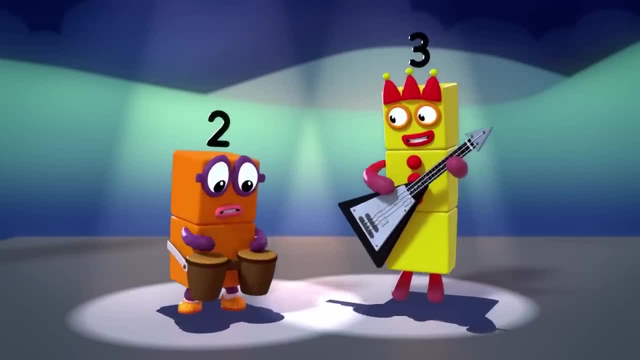 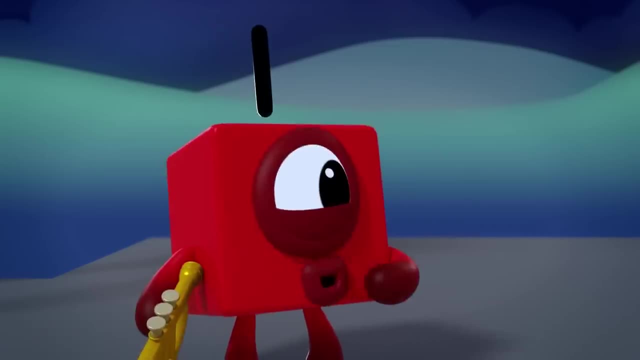 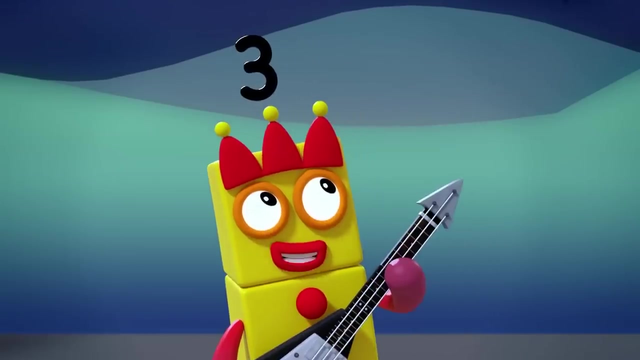 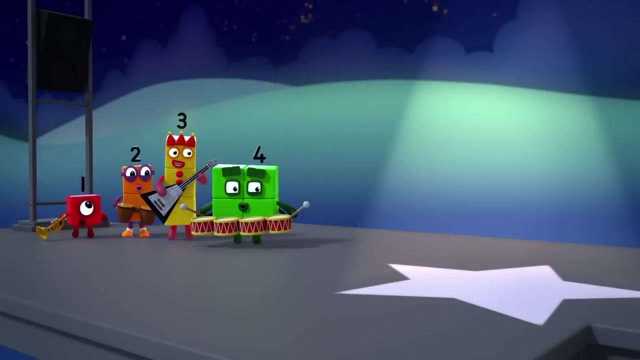 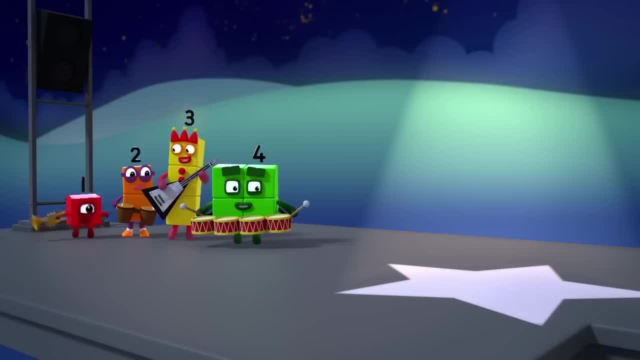 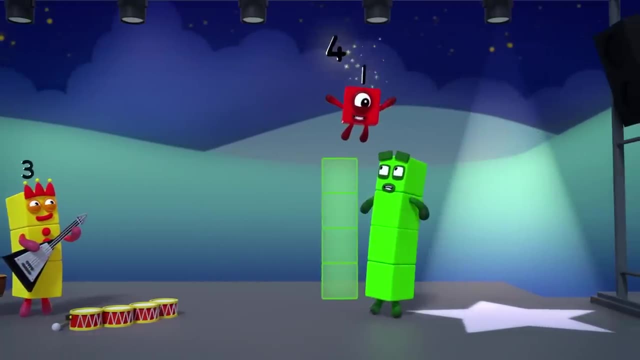 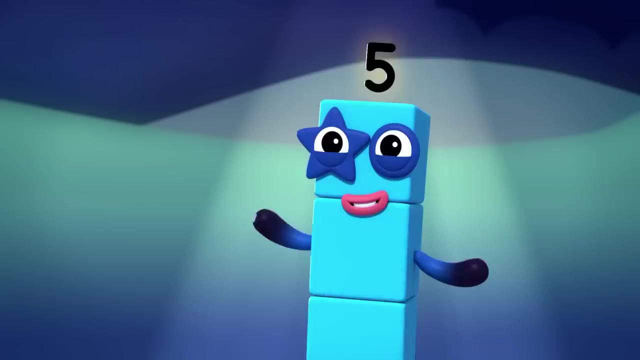 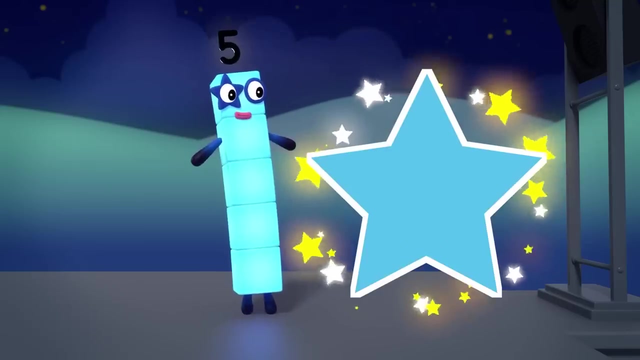 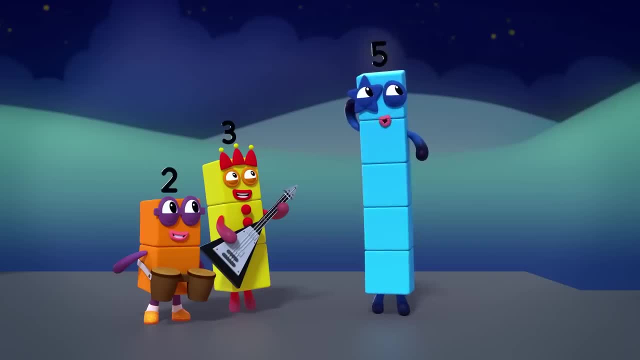 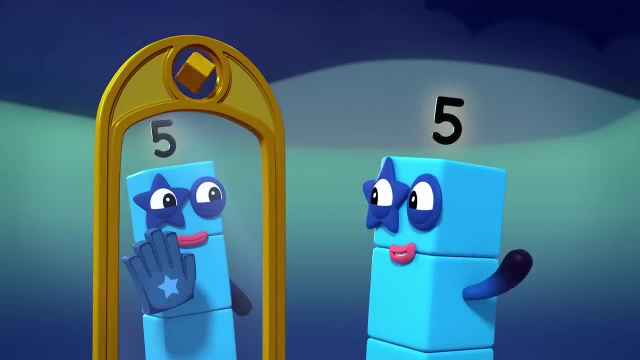 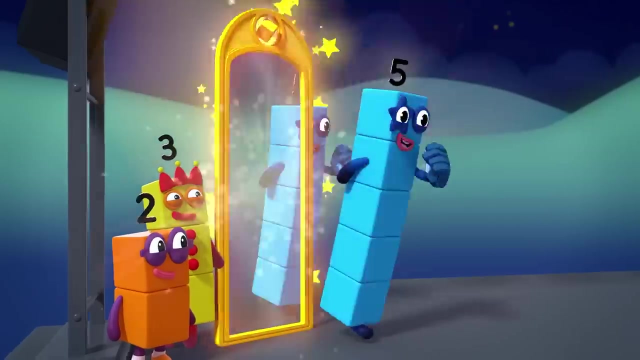 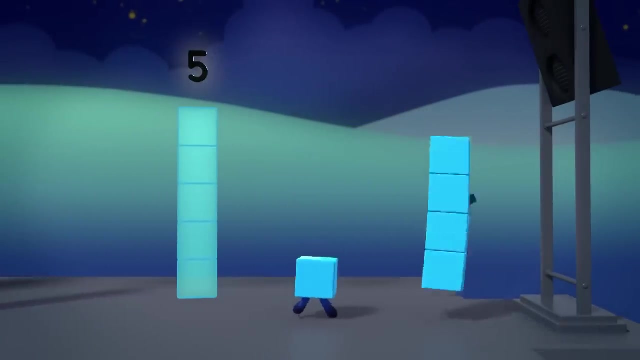 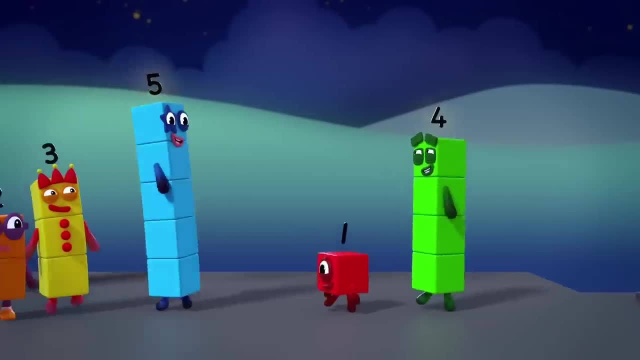 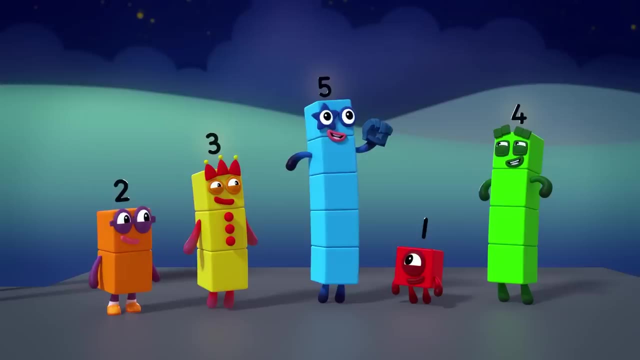 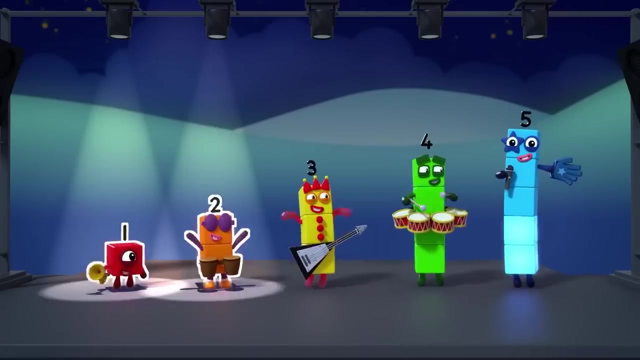 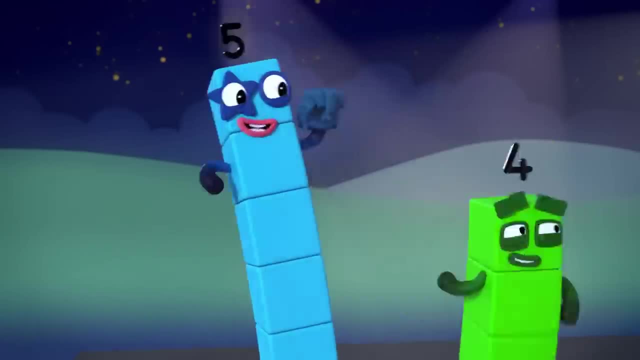 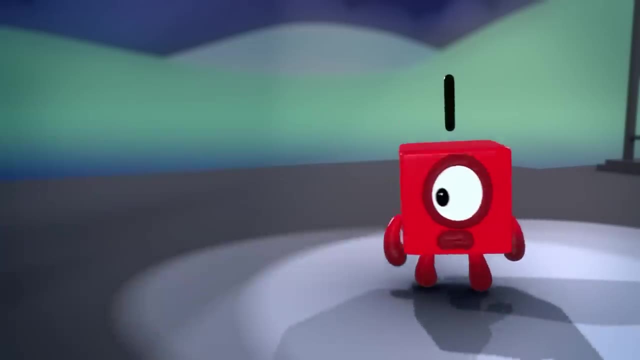 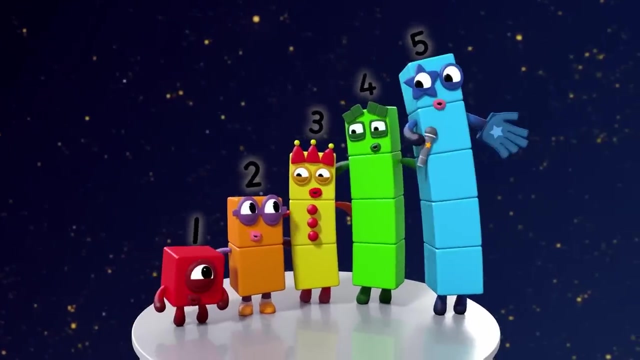 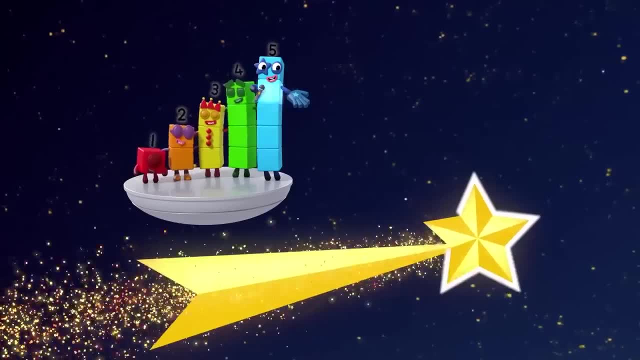 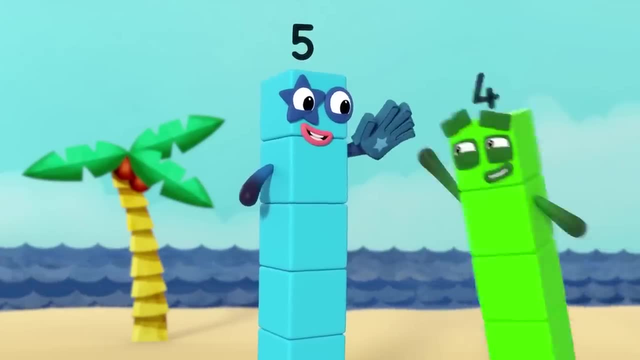 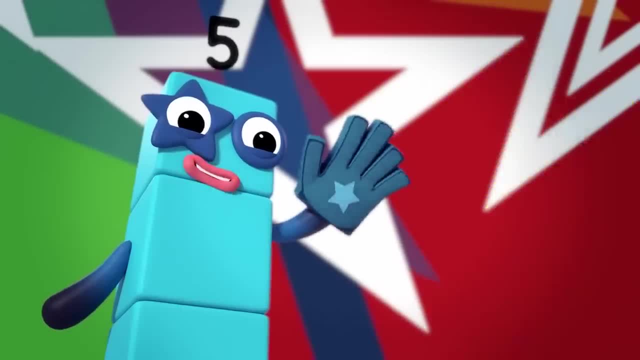 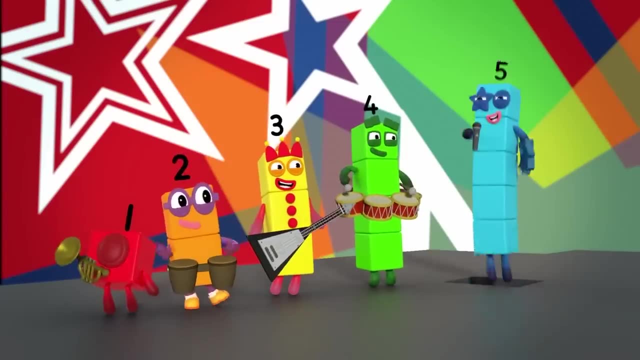 High five, High five To the side, up above, down low, too slow. High five, Ooh, I feel so alive. You know that you'll arrive when you're with number five. Five fish fingers on a plate: One, two, three, four, five. 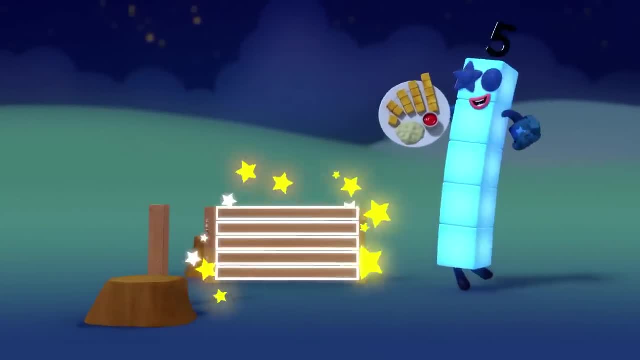 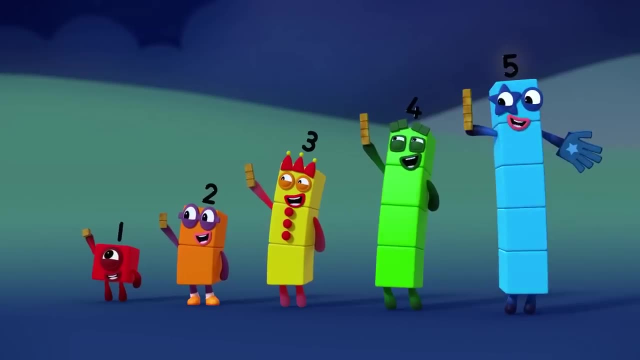 Five bars on a five-bar gate: One, two, three, Four, five, I'm five. Ooh, I feel so alive. You know that you've arrived when you're with number five, I'm number five, And I hope you understand. 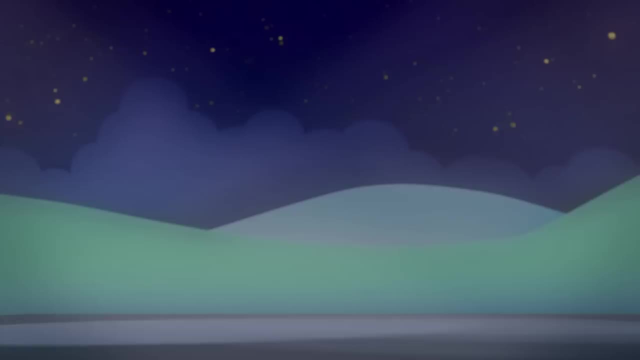 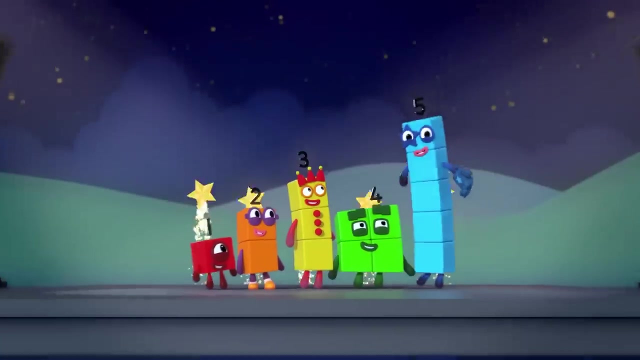 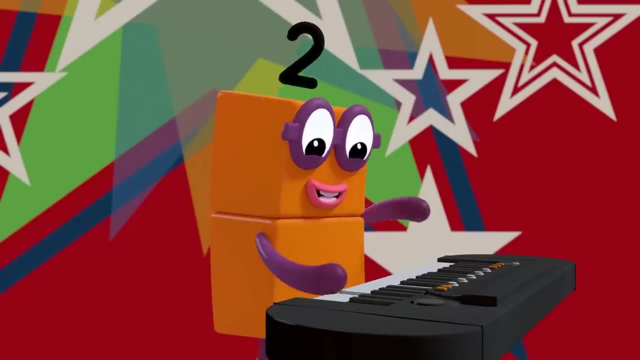 Whenever you need help, I'll be there to lend a hand. Now the band is all together. The rest can join the queue. We'll be five stars forever, And there's nothing we can't do. Three, two, one, two and action. 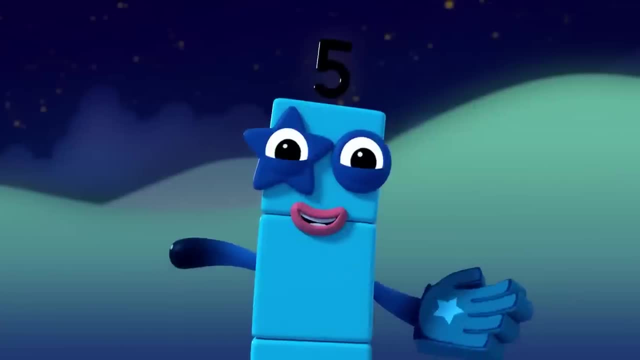 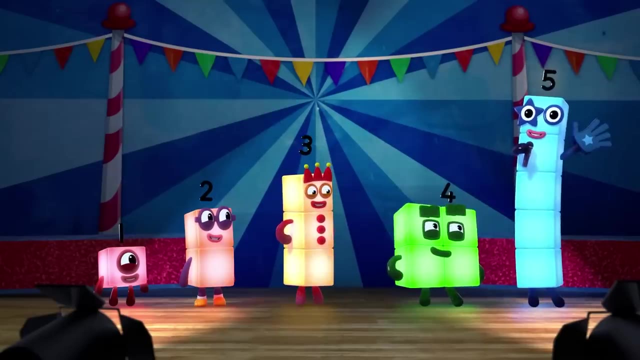 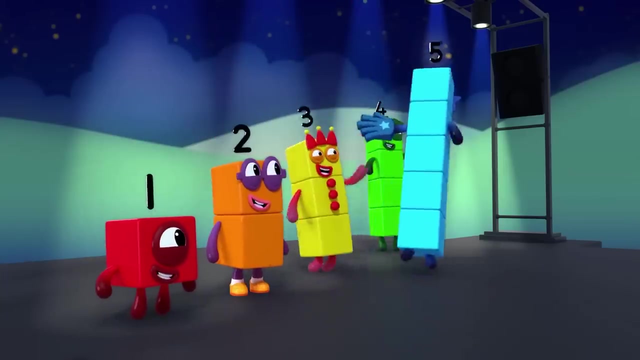 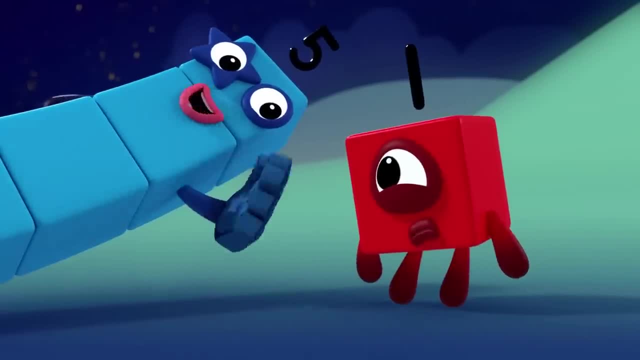 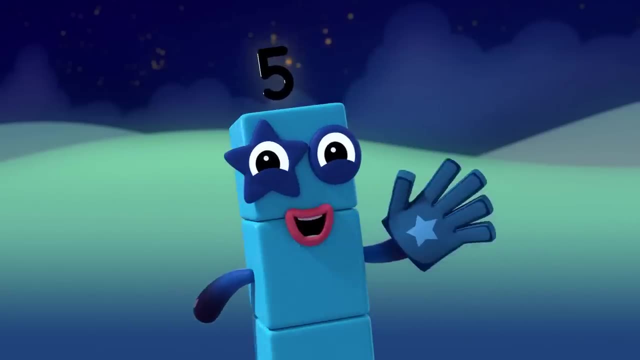 To the side, up above, down, low, too slow, High five, Ooh, I feel so alive. You know that you'll arrive when you're with number five. You know that you'll arrive when you're with number five. you've arrived when you're with number five. five birds, five trees, five flowers, five bees, one, two. 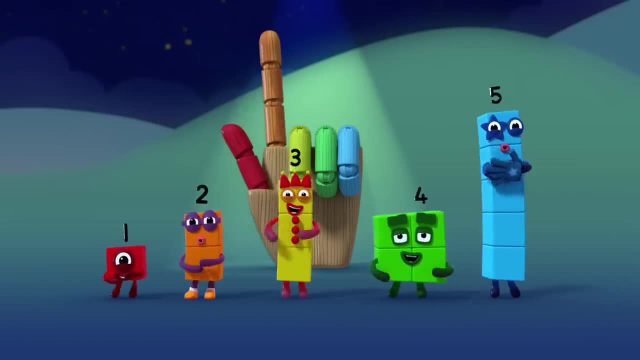 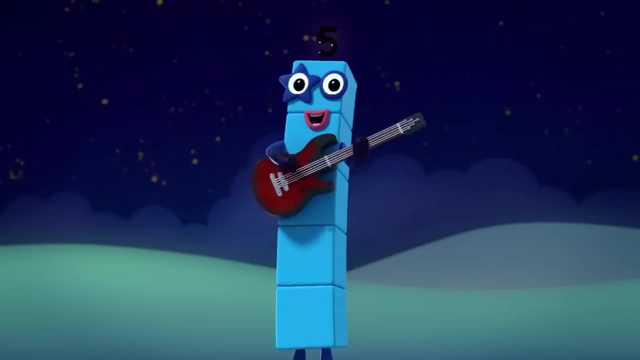 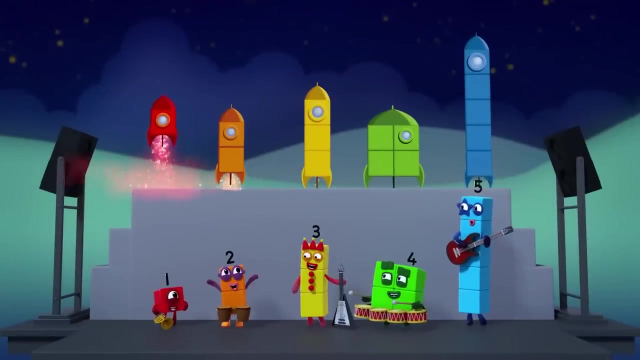 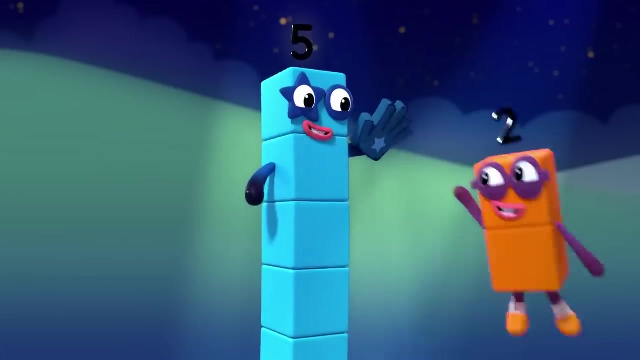 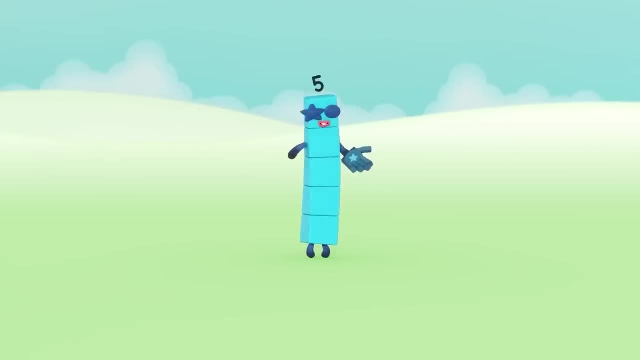 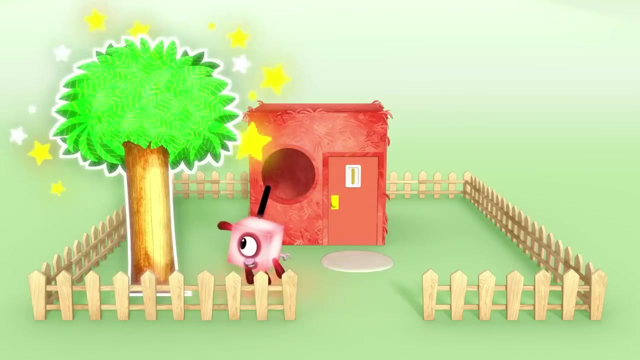 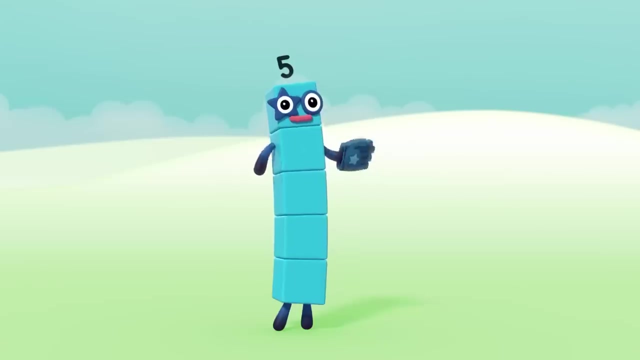 let me tell you a story. once upon a time there were three little pigs. the first little pig had a house with one room. look, it has one one window and one one tree in the garden and there's a number one on the door. but then came the big bad squirrel. 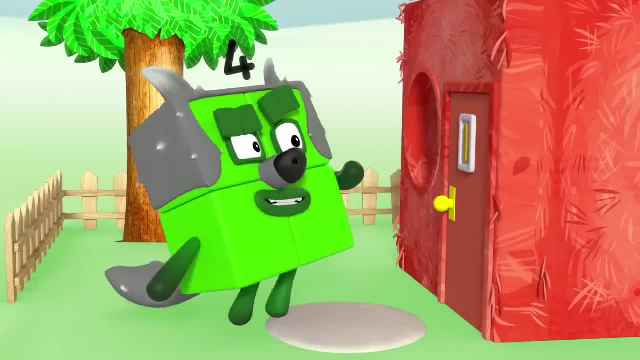 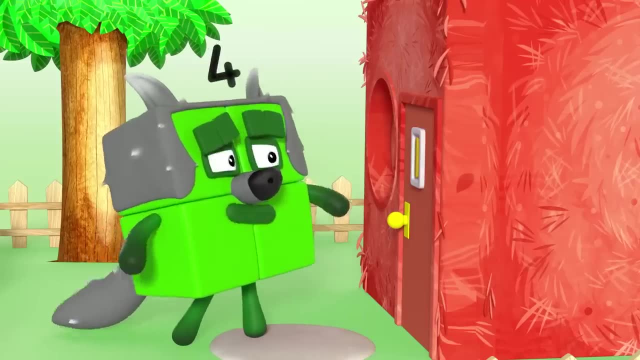 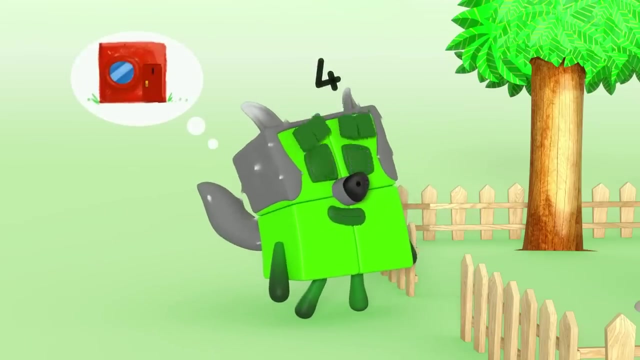 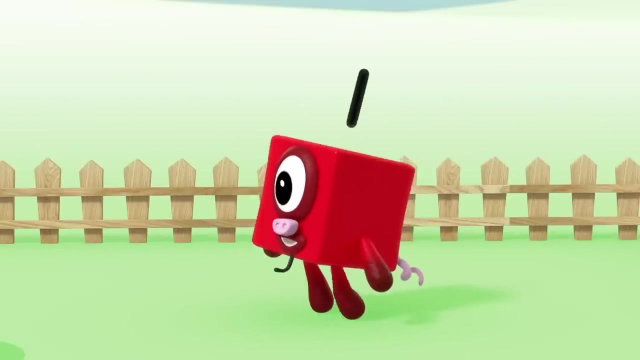 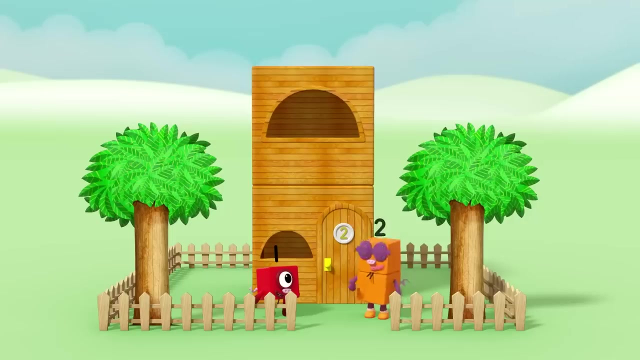 little pig, little pig, let me in. let me in, not by the hair on my chin, then i'll and i'll puff and i'll blow your house in shame. that's so square. luckily, the second little pig had a house with one room, Two rooms, Room for two, me and you. 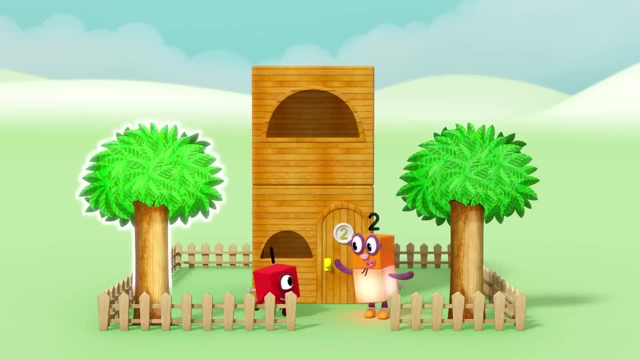 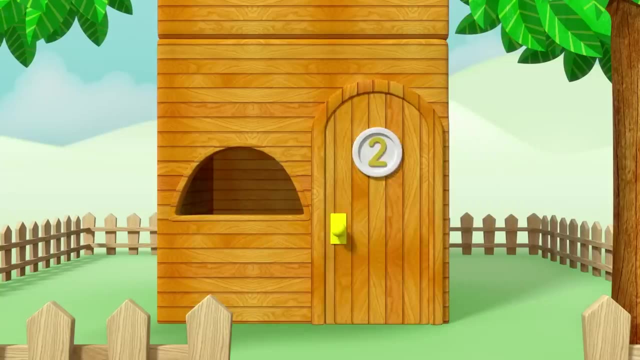 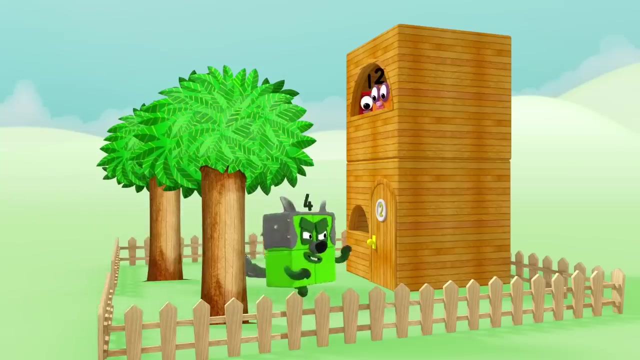 It has one two, two windows and one two, two trees in the garden And there's a number two on the door: Tea for two and two for tea. Little peg, little peg, let me in, let me in. 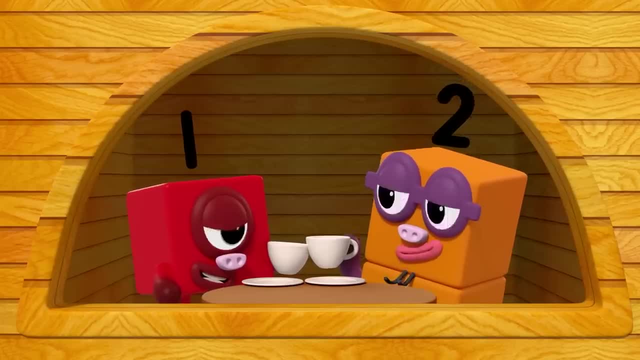 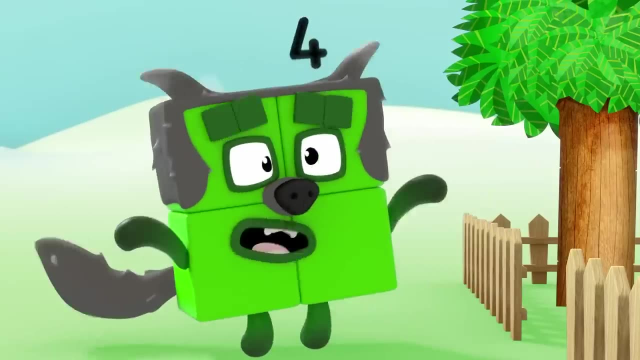 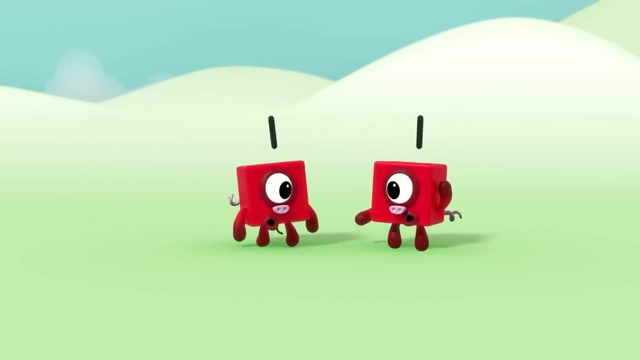 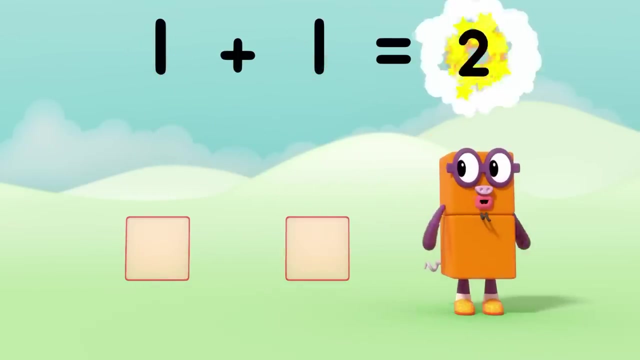 Not by the two hairs on my chinny chin. Then I'll huff and I'll puff and I'll blow your house in. Oops, Sorry, two. One plus one equals two. No worries, It's only pretend, But where will we go? 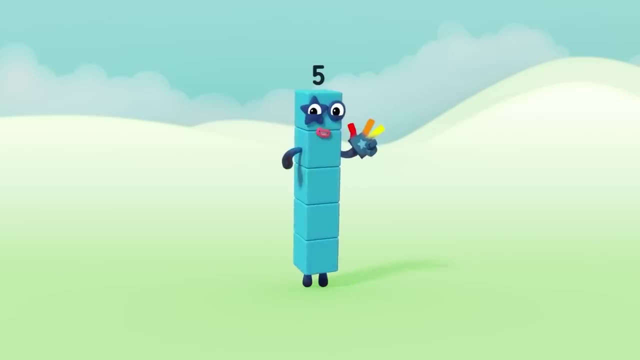 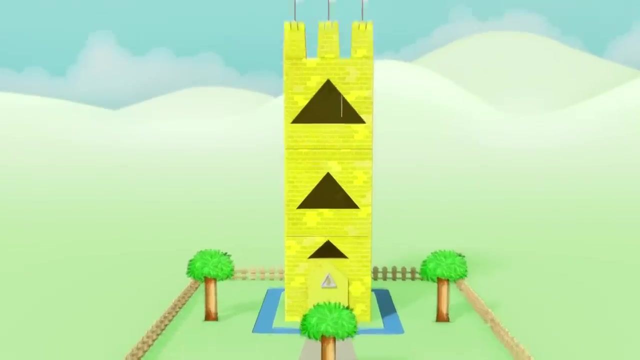 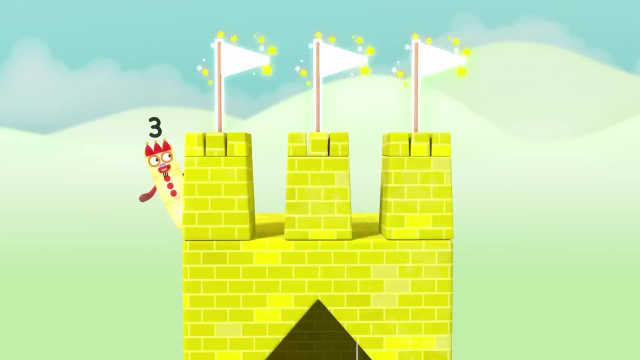 I don't know. Luckily, the third little peg- oh that's me busy, busy, busy- had a house with three rooms and one, two, three, three windows, and one, two, three, three turrets and one, two, three, three flags. 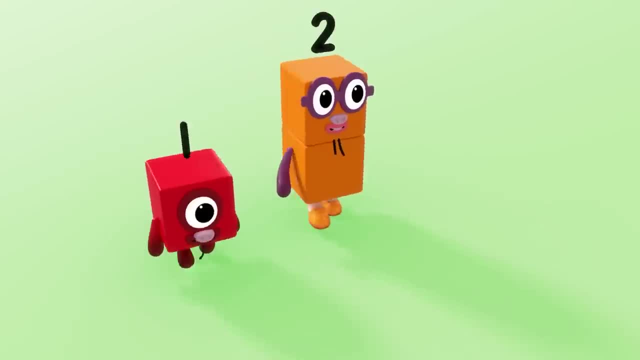 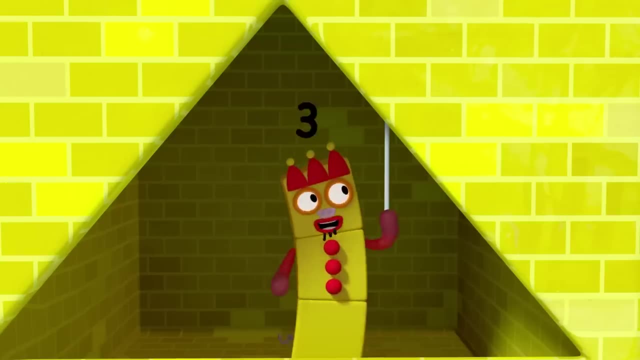 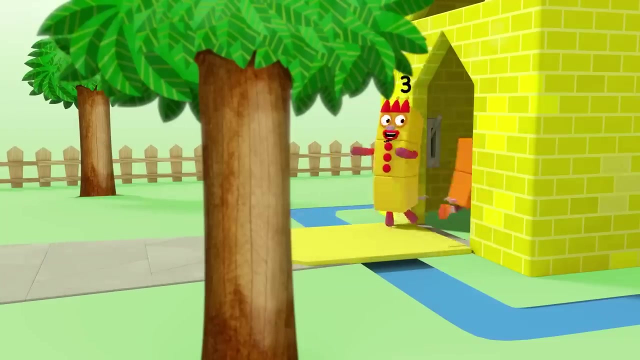 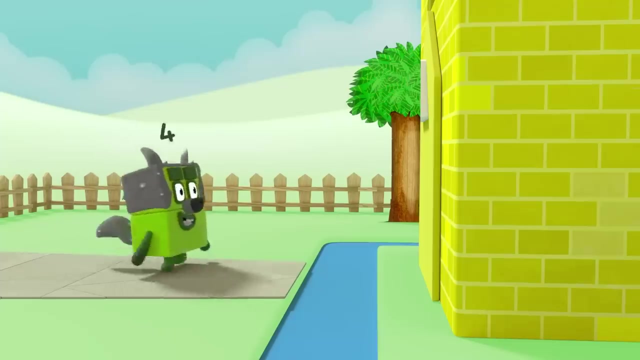 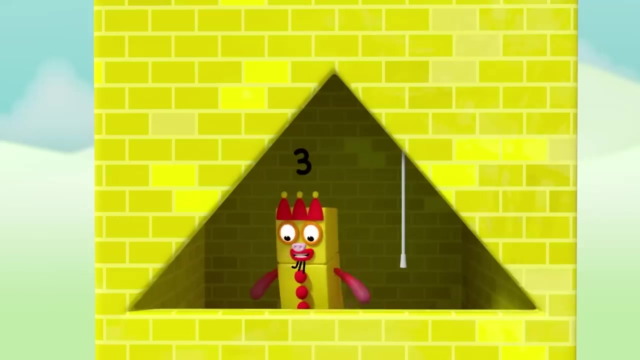 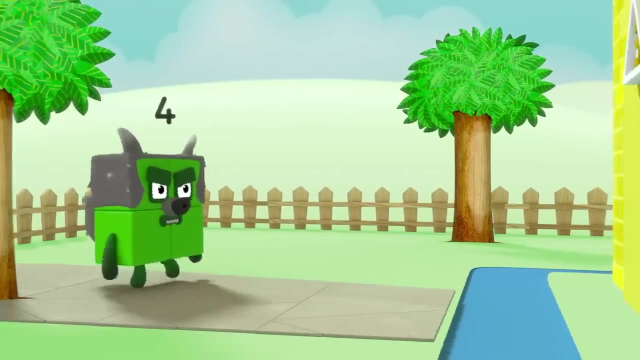 and yes, yes, thank you. three Room for a couple more. Sure, Two's company and three's a party. Lets make our house one. No, Up, up, Up, Up, Up, Down, Up Down. 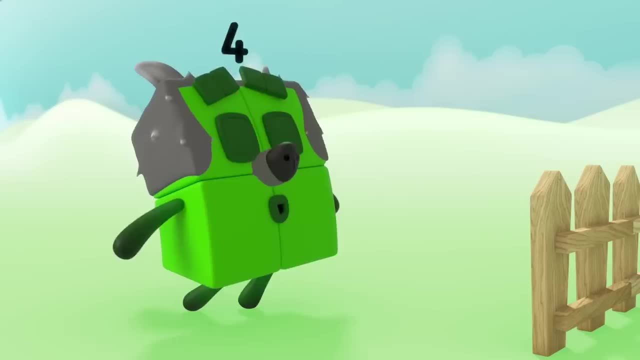 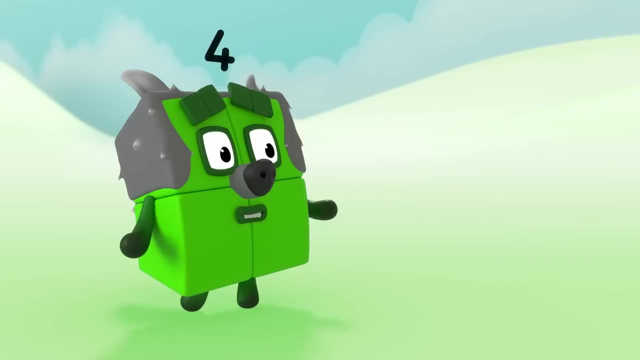 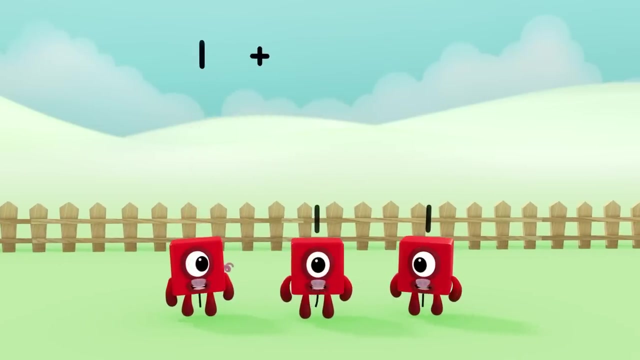 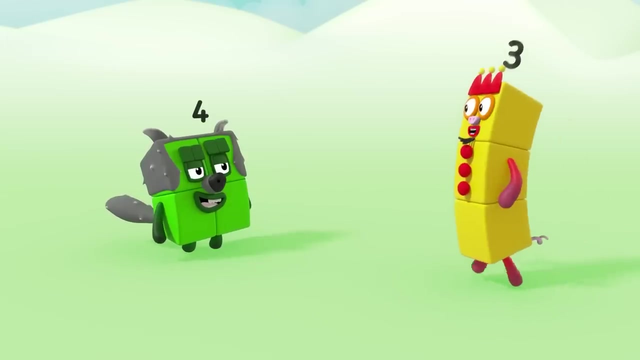 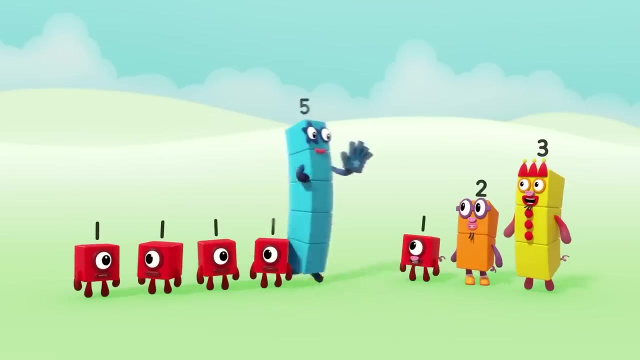 Up What? But how? Just a little huff, Huh Hey, One plus one plus one Equals three. See how you like it. Stop. This isn't how the story goes. The third house doesn't get blown down. 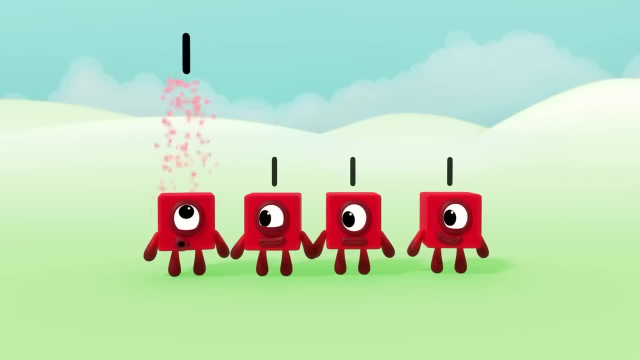 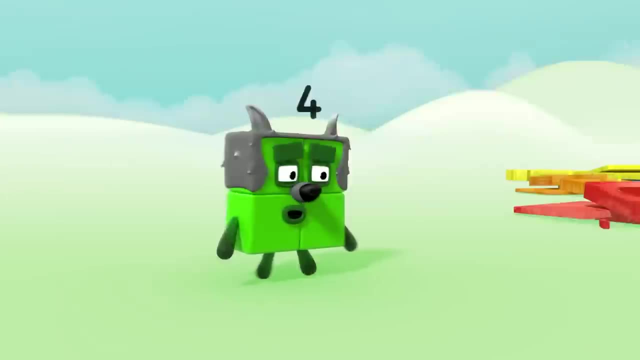 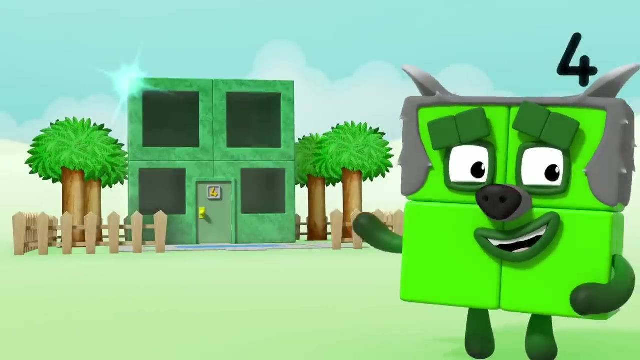 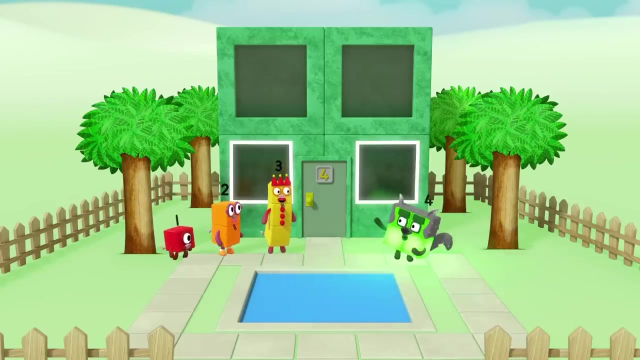 One plus one plus one plus one Equals Four. Where will the three little pigs live now? There's always my house. It's got four rooms. Oh, that's great. I'm so happy, I'm so happy. Four windows with one, two, three, four. 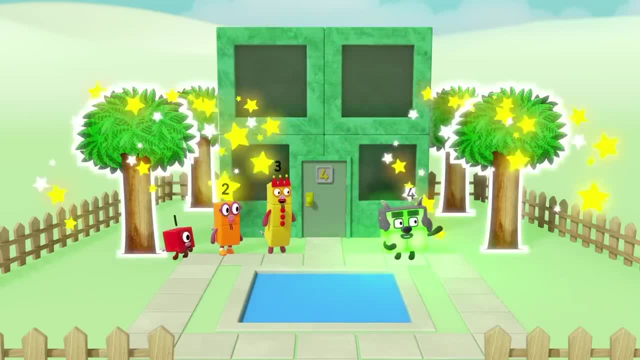 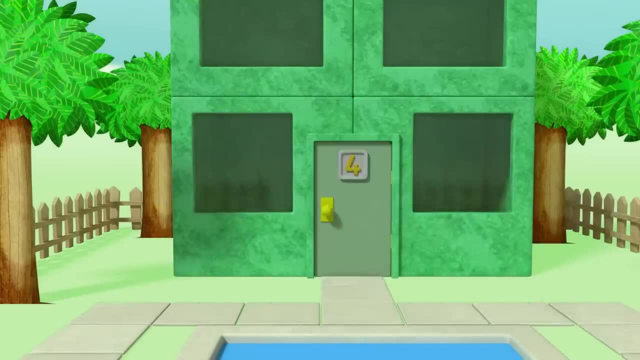 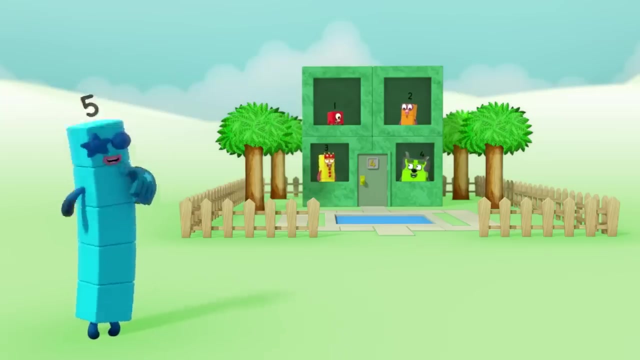 Four windows and one, two, three, four, Four, threes and a number four on the door. One, two, three, four. That deserves a big hand. Once upon a time there were three little pigs and a big bad square. 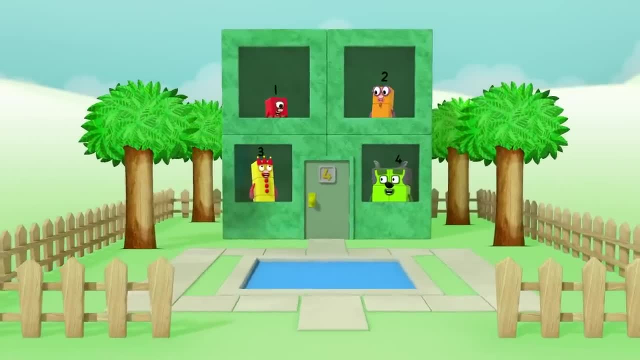 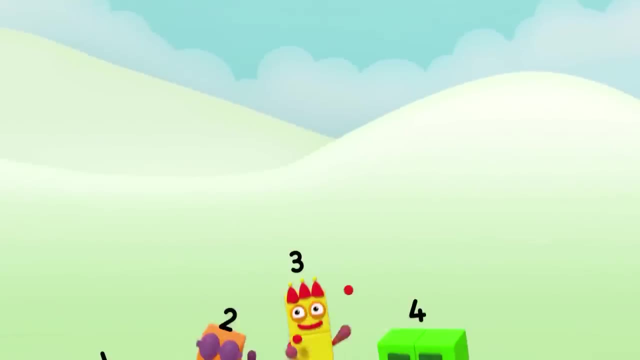 and they all lived happily ever after The end. Yay, Yay, Hop, hop, hop. One two, one, two, three, four. One two, one, two, three, four. One, two, three, four. 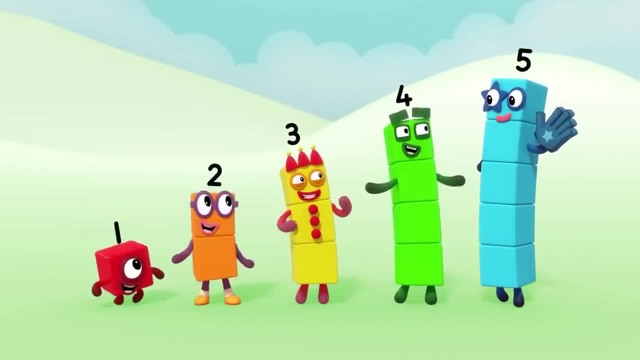 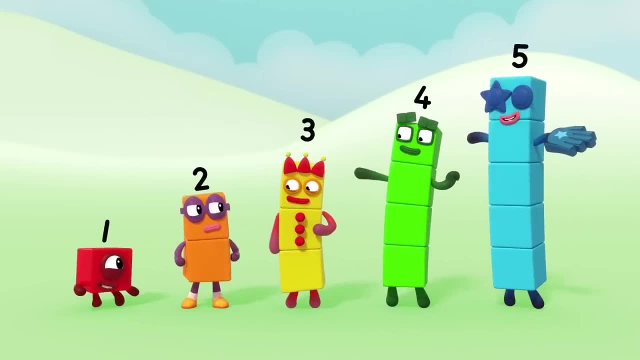 One, two, one, two, three, four, I can do my exercises. Hi team, High five. So are we all here? Um well, how can we tell? I know just the thing: Ready, steady, sing. 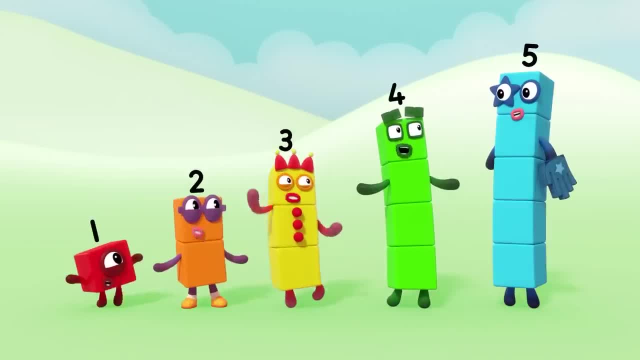 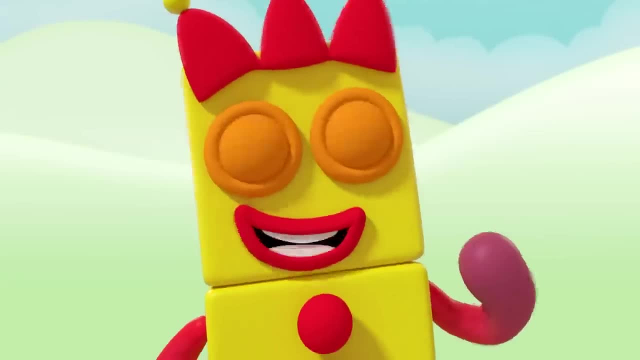 One, two, three, four, five. That sounds right. What shall we do today? Walk in the sunshine, Run through the forest, Climb to the top of a tree, Pretend to be pirates, Discover a whole new world. 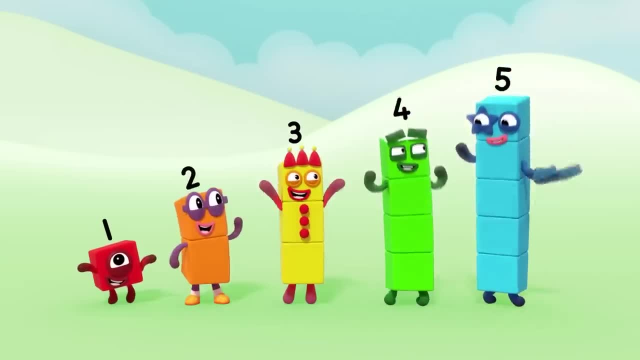 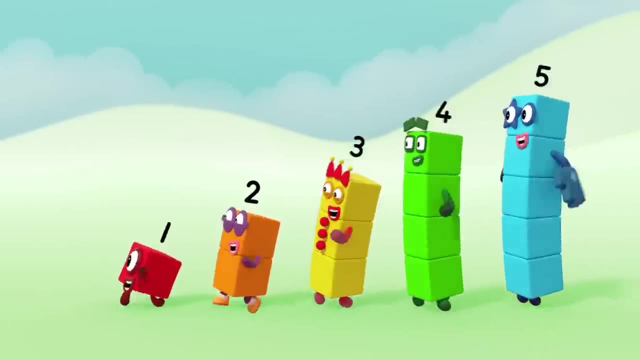 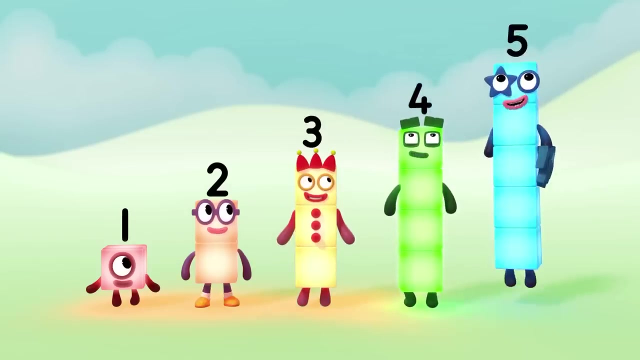 Let's have an adventure. Hooray, Everybody ready, Off, we go Off. we go on a big adventure. We don't know what the day will bring. Off, we go on a big adventure. Ready, steady, send One, two, three, four, five. 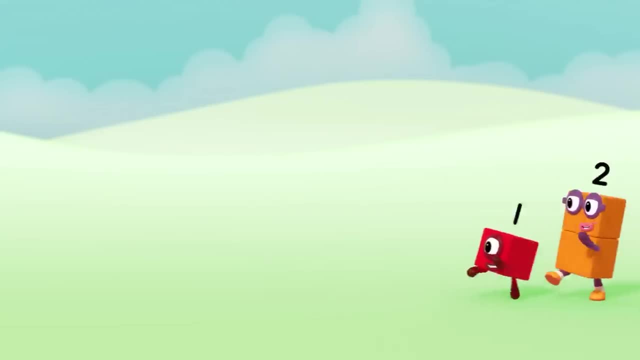 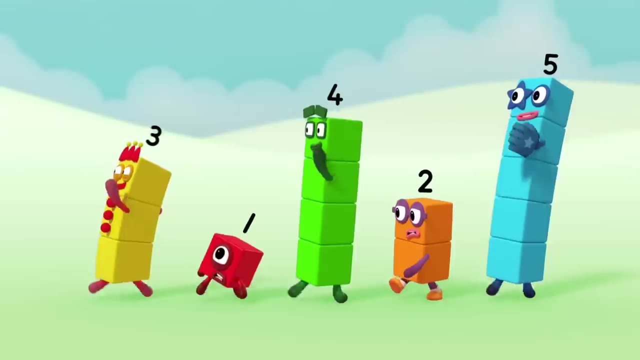 That sounds right. And off we go again. Off we go on a big adventure. We don't know what the day will bring. Off we go walking in the sunshine, Ready, steady, send. Wait Too short, Can't see. 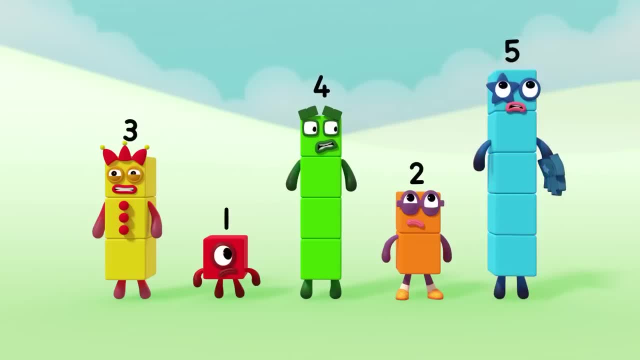 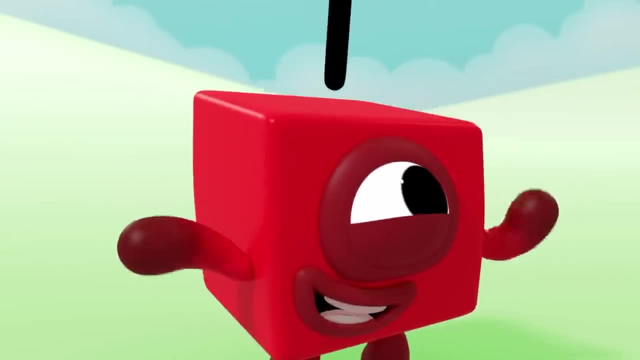 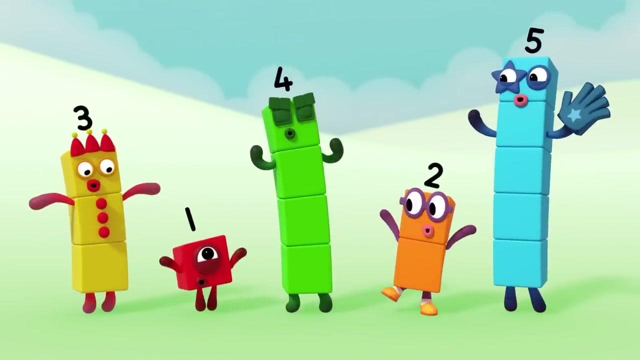 Three, one, four, five. That doesn't sound right. We're in the wrong order. I know what to do. Diddly, diddly do. Smallest that way, biggest this way Go, I'm bigger than you. 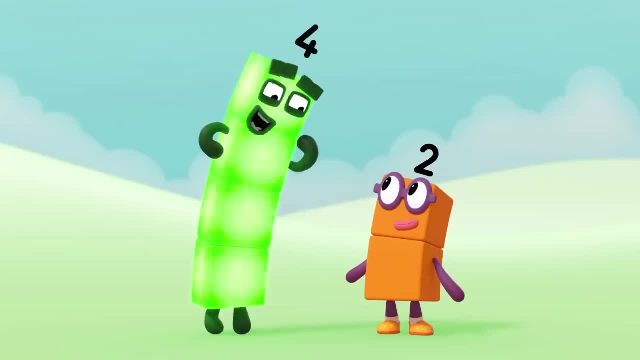 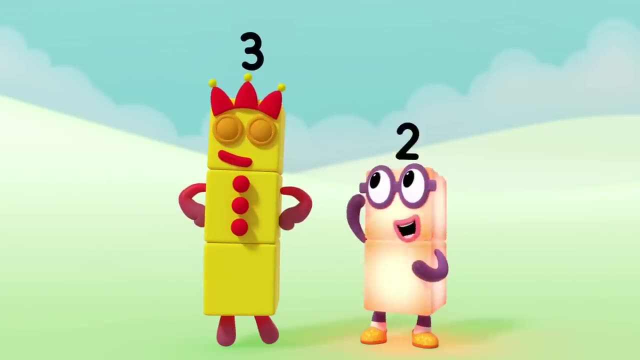 I'm smaller than you Diddly diddly do. I'm bigger than you. I'm smaller than you Diddly diddly do. I'm bigger than you. I'm smaller than you Diddly diddly do. 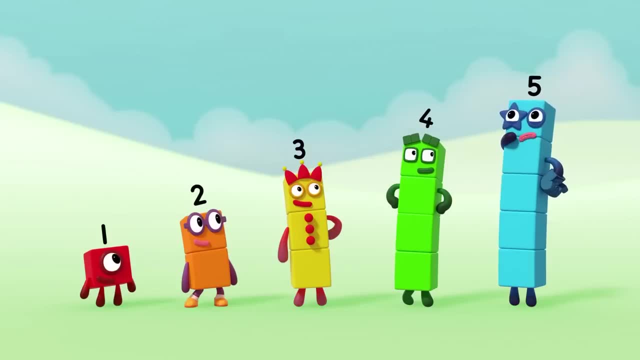 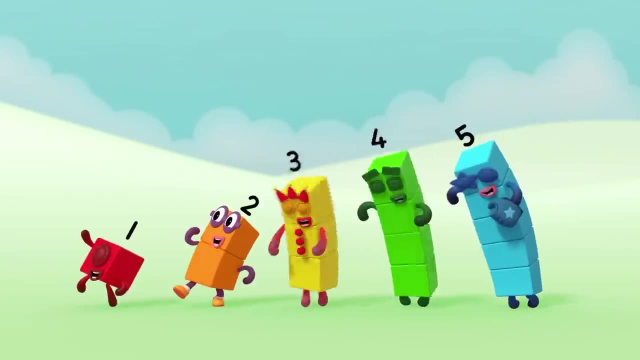 Are we all in order? Did we all do the right thing? Ready, steady, sing One, two, three, four, five. That sounds right. And off we go again, Off we go on a big adventure. We don't know what the day will bring. 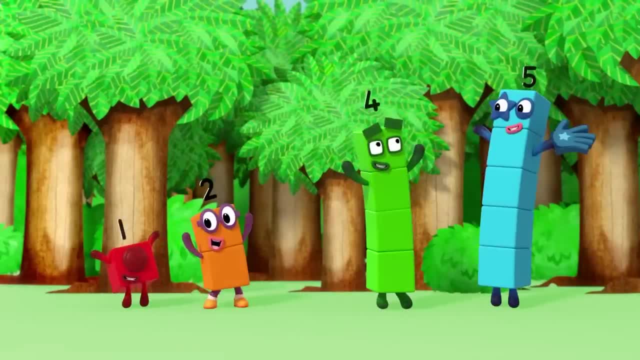 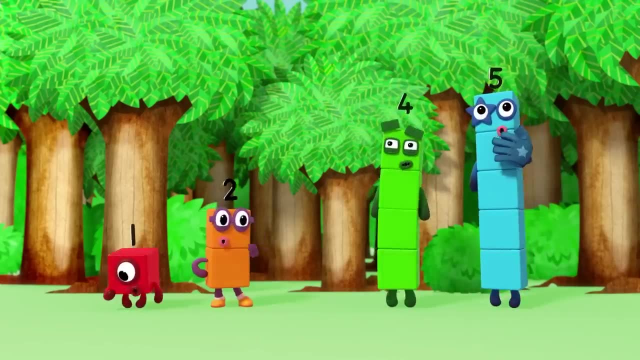 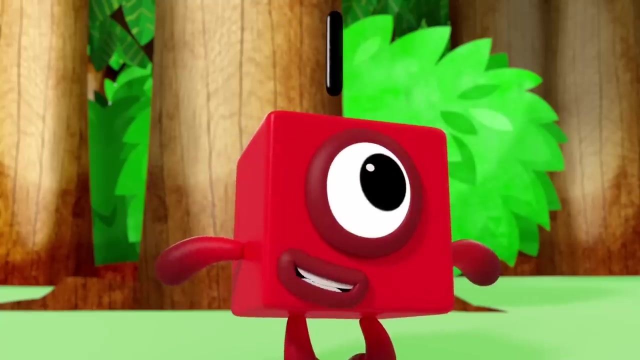 Off we go running through the forest, Ready, steady, sing One, two, four, five. That doesn't sound right. Someone's missing. Who can it be? Let's see. I'm one, Start with me. I'm two, I come after one. 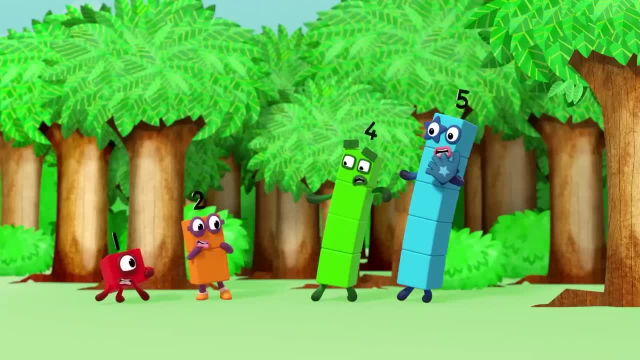 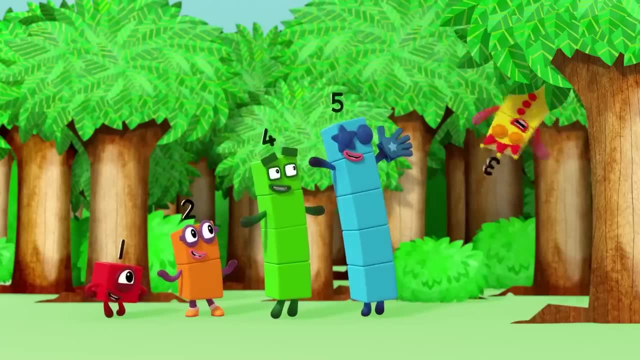 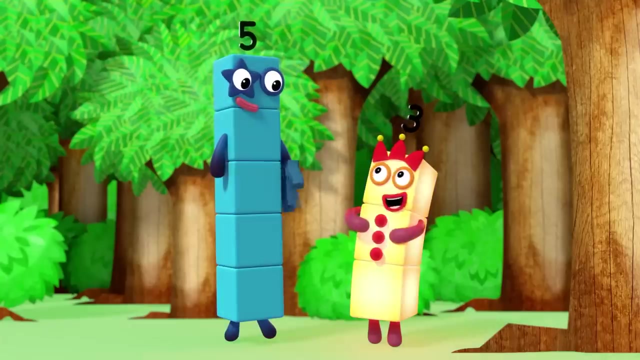 I'm four. I come after three. Three, Three's missing. Where is three? Look at me, I'm number three. Three, I know what to do. Diddly, diddly do. I'm bigger than you. I'm smaller than you. 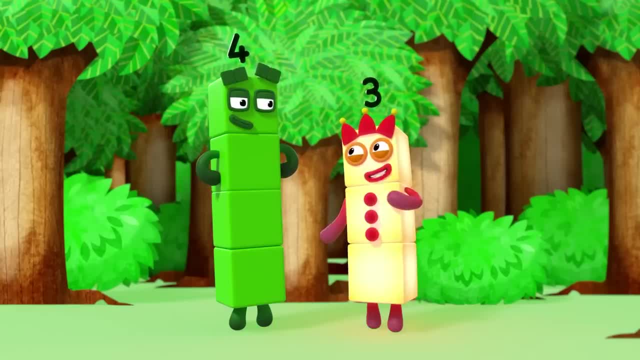 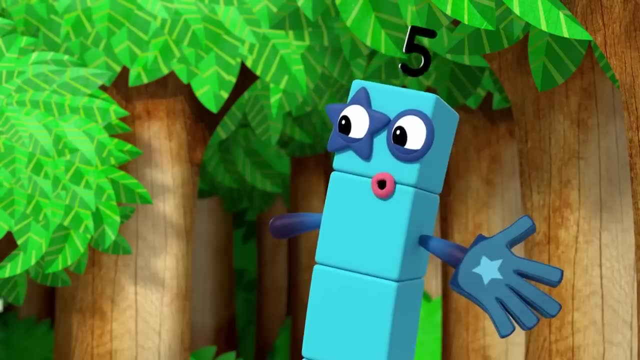 Diddly diddly do I'm bigger than you. I'm smaller than you. Diddly diddly do I'm smaller than you. Stop, Are we all here now? Did we all do the right thing? Ready, steady, sing. 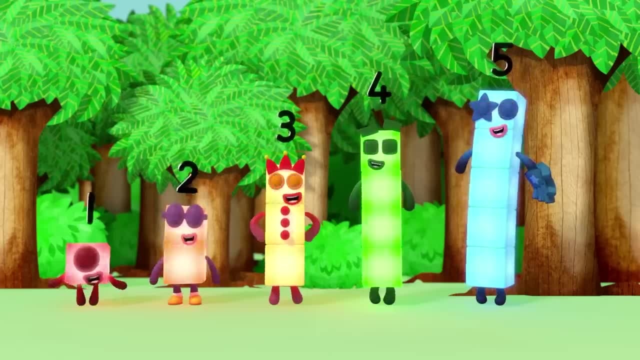 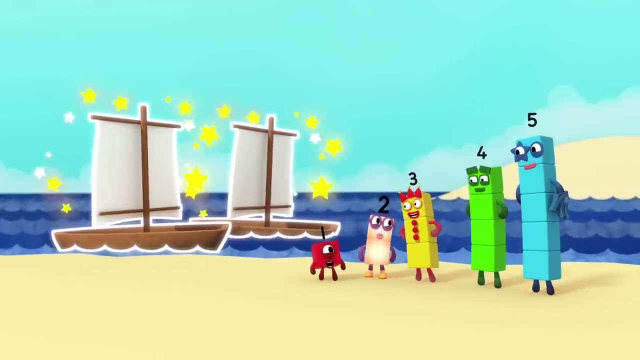 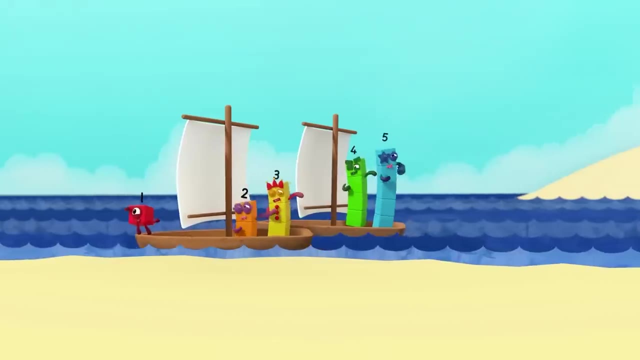 One, two, three, four, five. That sounds right. And off we go again. Look, One, two, two sailing boats. We can be pirates. Ha, ha, ha. Off we go on a big adventure. We don't know what the day will bring. 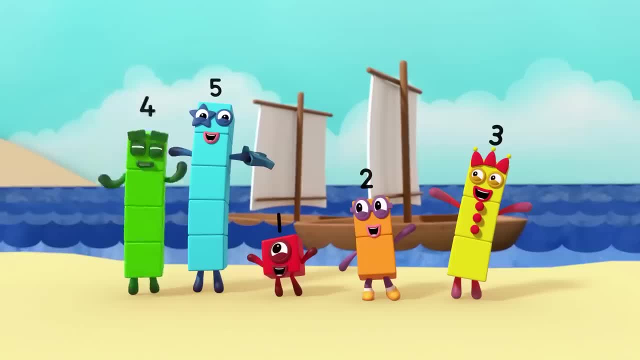 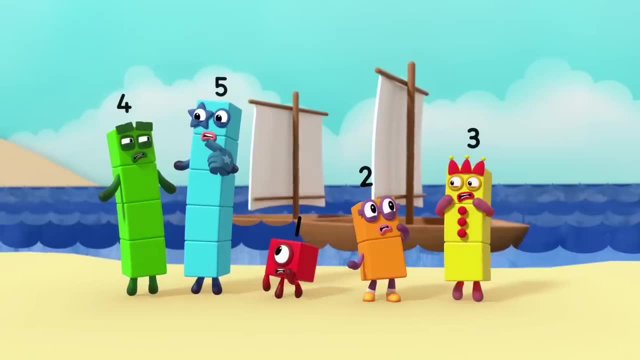 Off we go, sailing on the ocean, Ready, steady, sing Four, five, One, two, three. That doesn't sound right. We're in the wrong order. We know what to do. Diddly, diddly do. 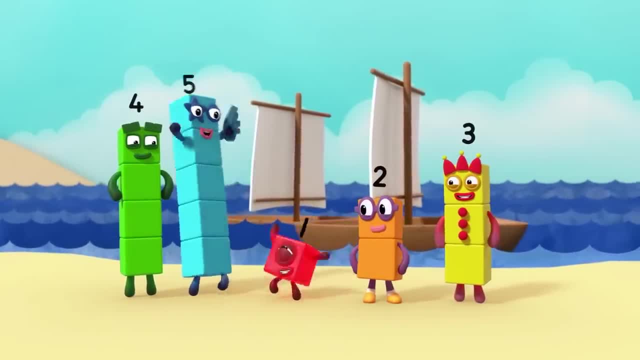 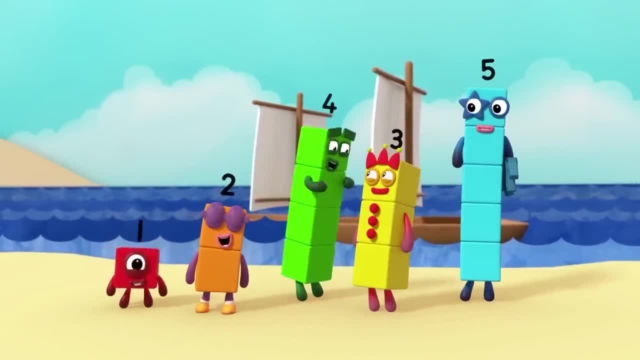 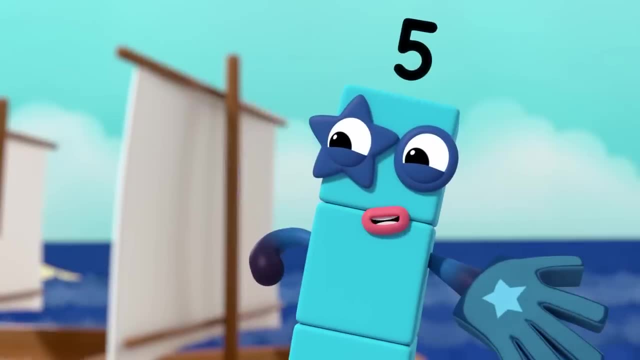 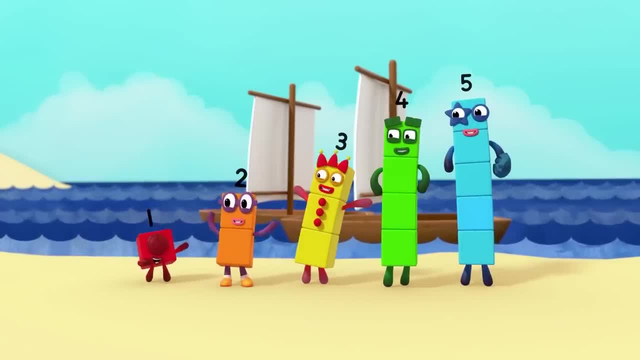 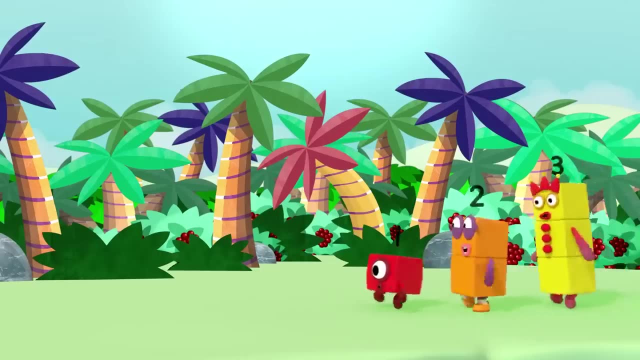 Did we all do the right thing: Ready, steady, sing One, two, three, four, five. That sounds right. And off we go, again Off we go on a big adventure. we don't know what the day will bring. 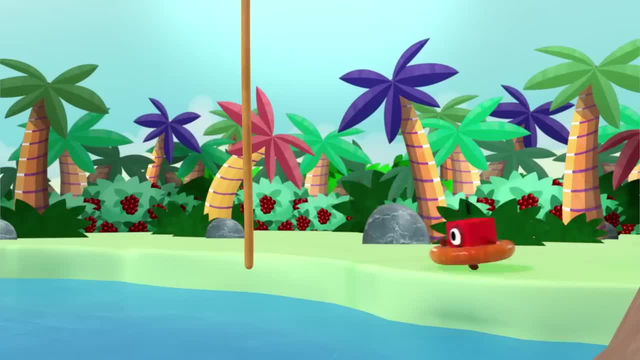 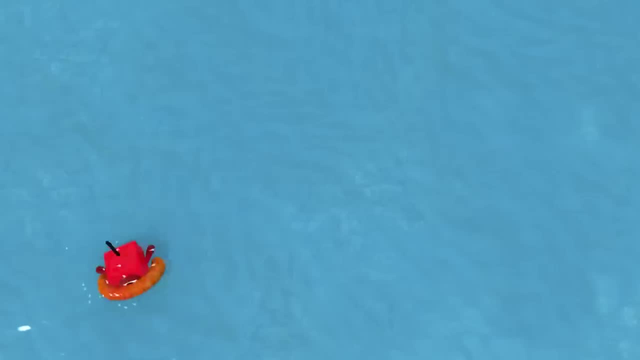 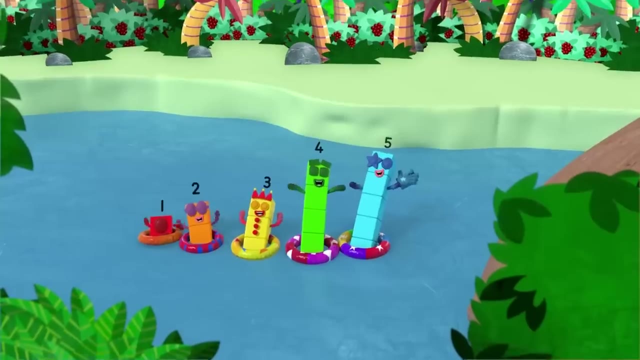 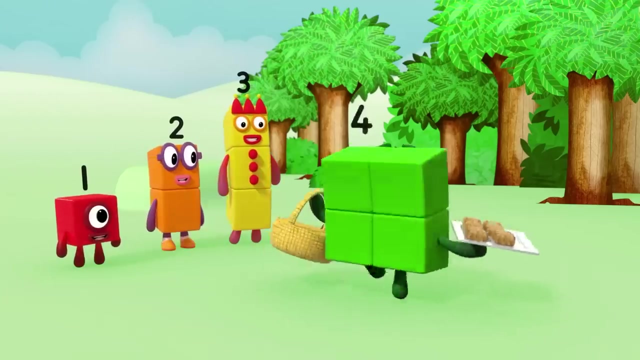 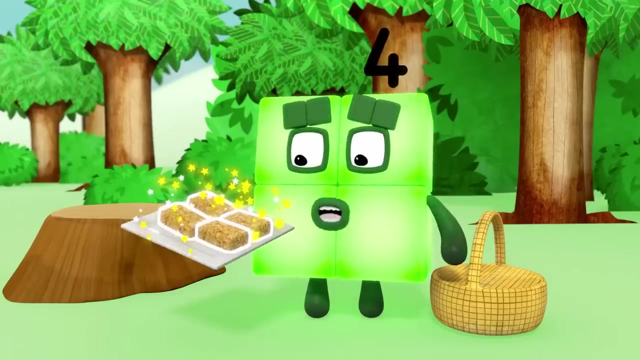 Here we are discovering a new world. Ready, steady, sing Yeah, One, two, three, four five. One, two, three, four, five. Look what I've got. Oh, one, two, three, four. 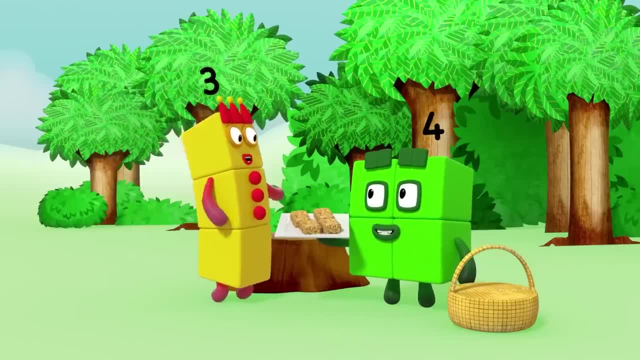 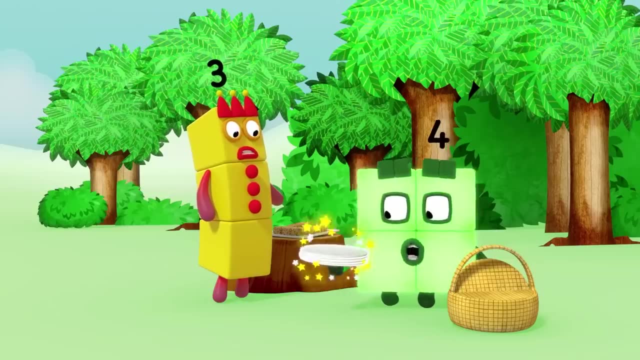 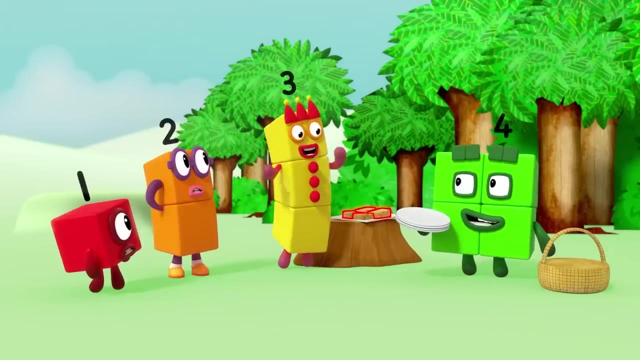 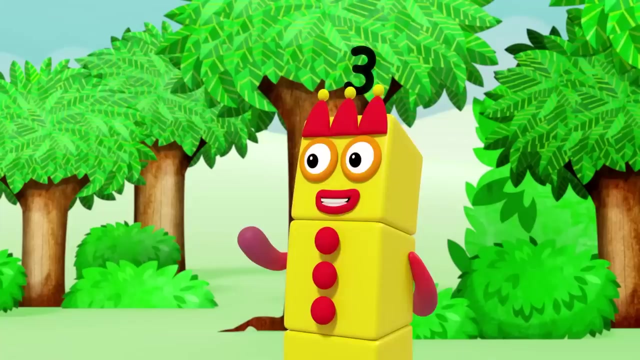 Four flapjacks, perfect for our picnic. Oh, hot, hot, hot. Better let them cool Now. one, two, three, four, Four plates. Just enough for one. one, two, three, three flapjacks, three flapjacks, once gone missing, but how, this might just be the work. 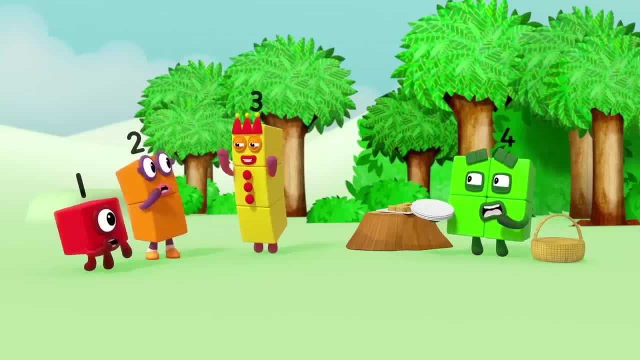 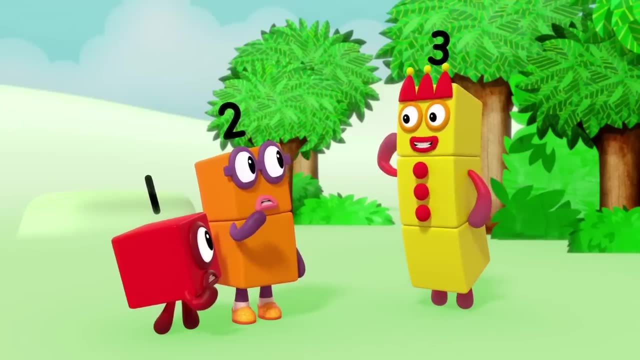 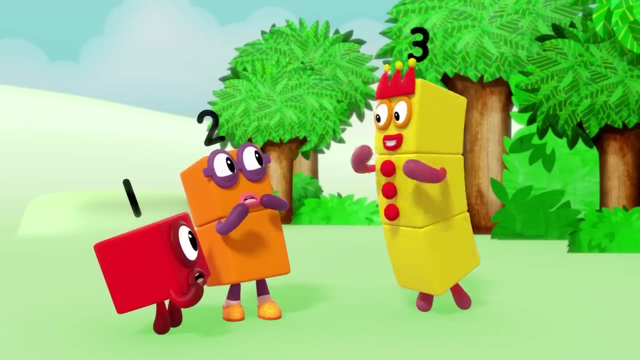 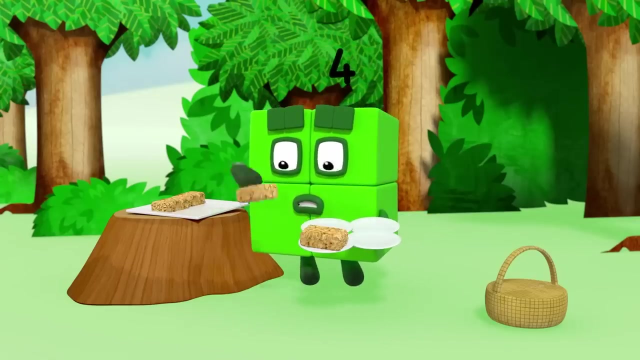 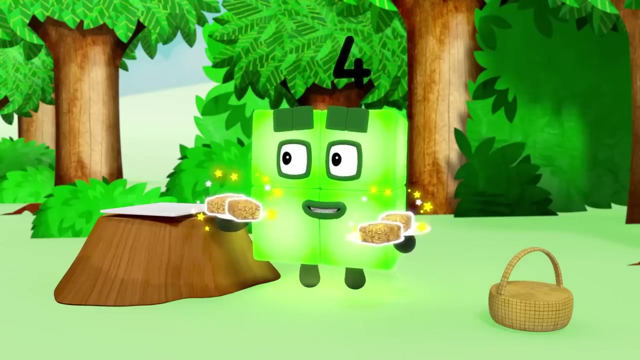 of the flapjack snafler. what's a flapjack snafler? it's a strange creature made of three blocks with three eyes to spy out flapjacks, three arms to grab flapjacks and three mouths to eat flapjacks. and there must be one hiding nearby because there are only one, two, three, four, four flapjacks. 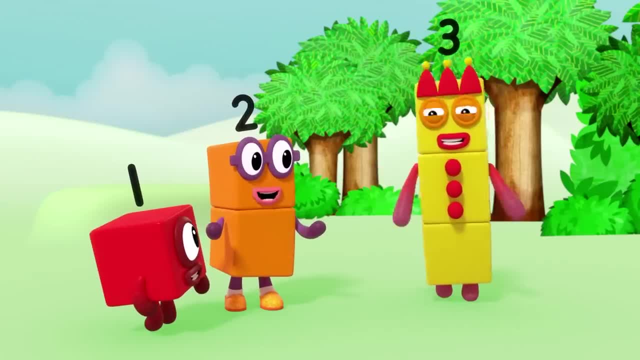 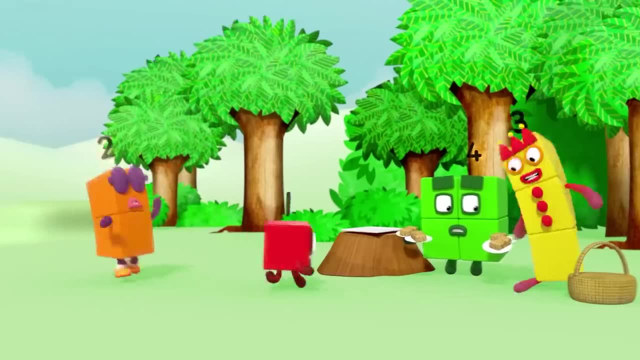 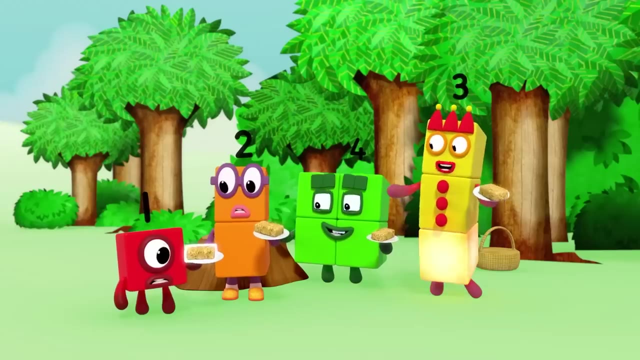 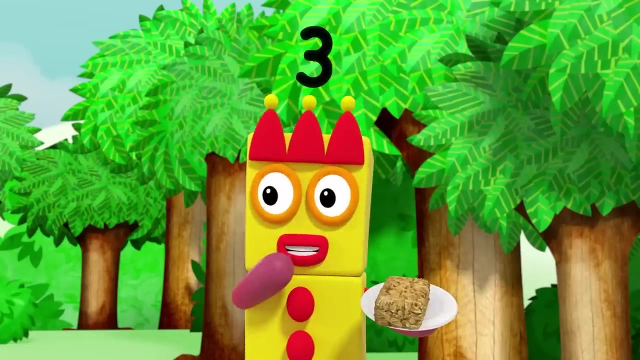 or oh no flapjack snafler's here. that's what it wants you to think. it's trying to trick us. everyone go to flapjack. i think we're safe, really. let's see one, two, four, three, three flapjacks. it struck again, the flapjack snafler. 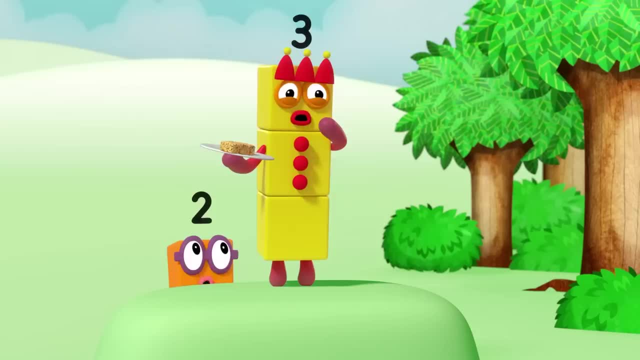 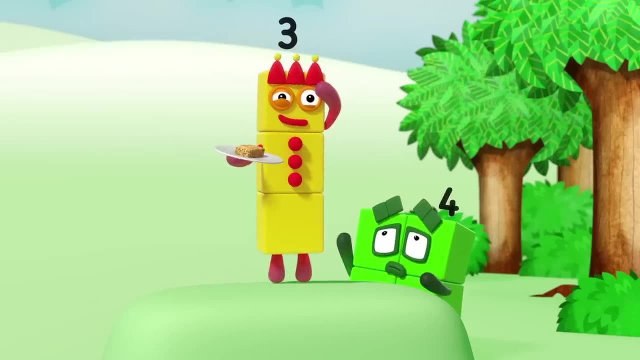 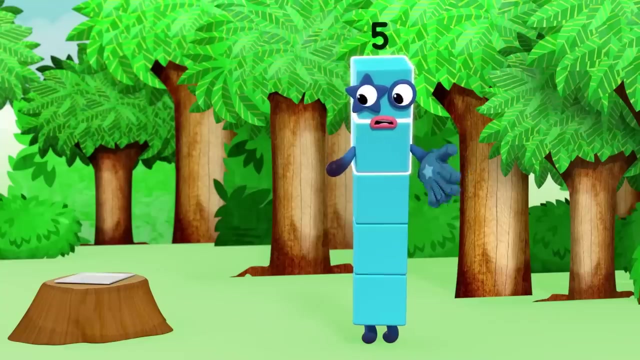 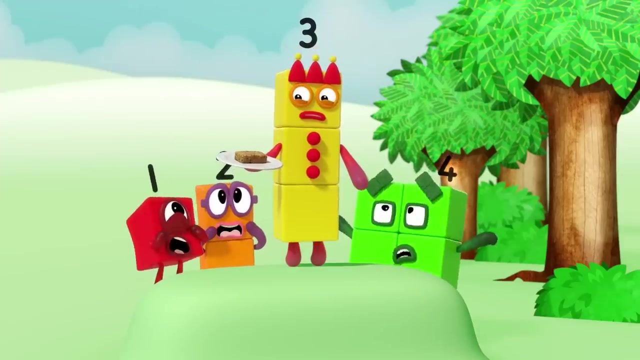 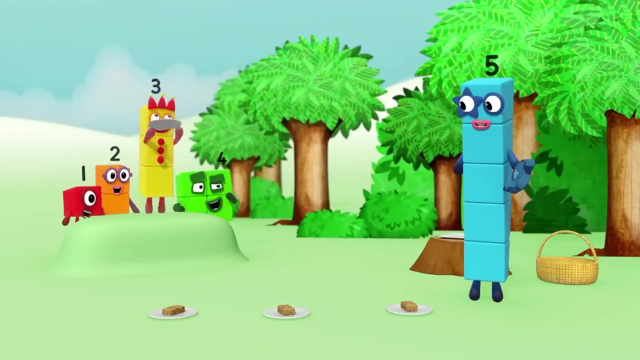 something's coming. how many eyes has it got? one, two, three? how many arms? one, two, three arms. how many blocks? one, two, three, four, five, three blocks? no, it's five. what are you all doing? five, you haven't got three eyes or three arms. whoever told you i did? 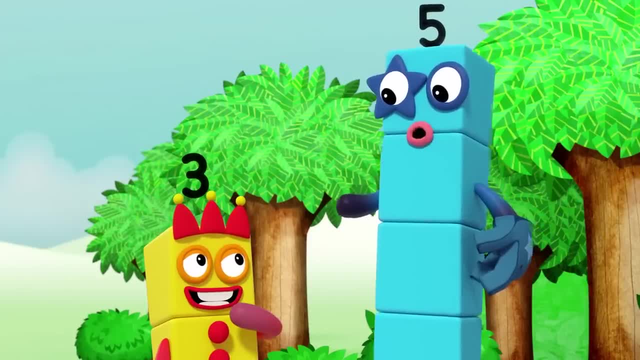 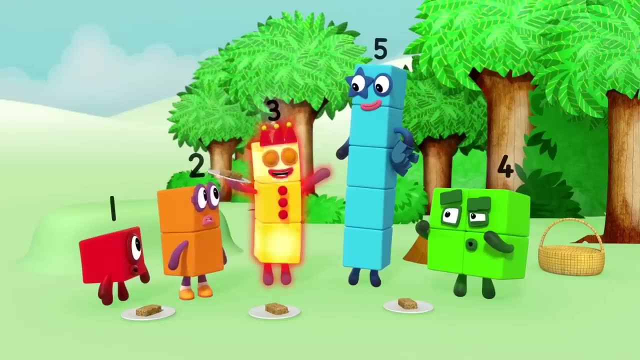 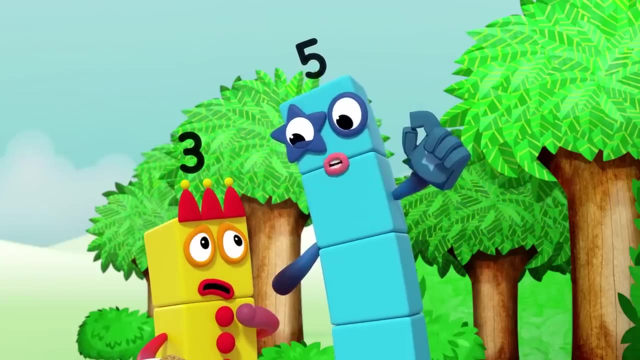 i counted them three. do you know how to count? yes, of course. look at a bunch of things, say some numbers and then say three, because three is the best number. there's a little more two than that three. there are some rules you have to follow. rule one: count everything once. try counting those. 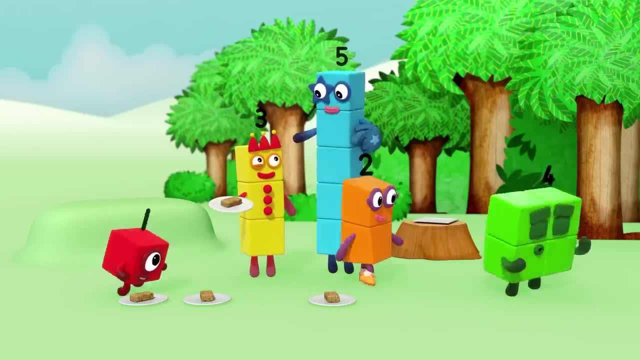 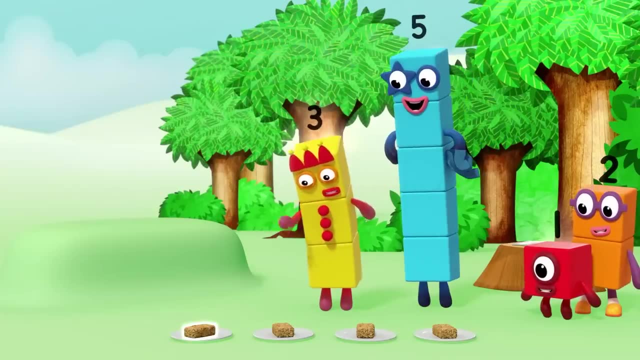 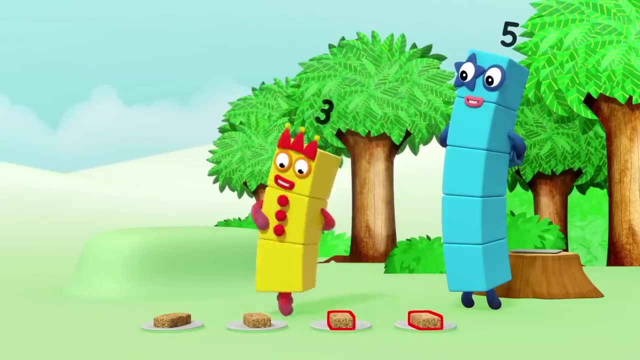 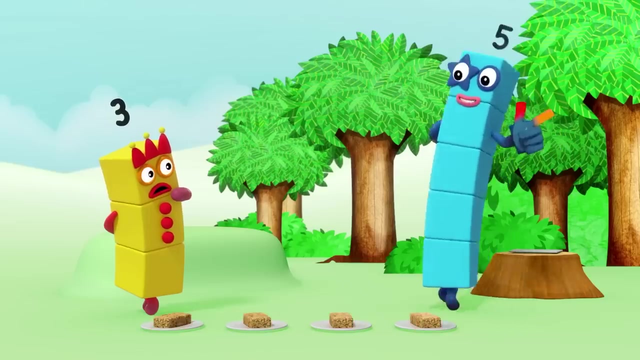 flapjacks. it can help to put them in a line and to point at them one at a time, to make sure that the one at a time, to make sure you don't miss any or count the same one twice. one, two, three, four. very good, four, three, two, one, wait one. that's not right. rule two say the numbers in the right order. 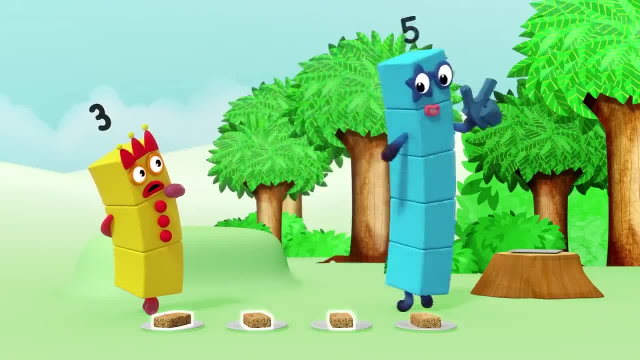 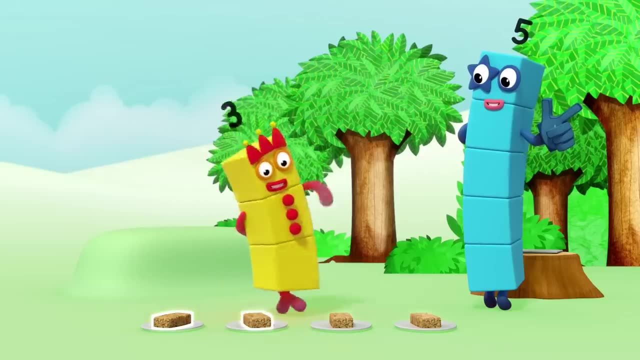 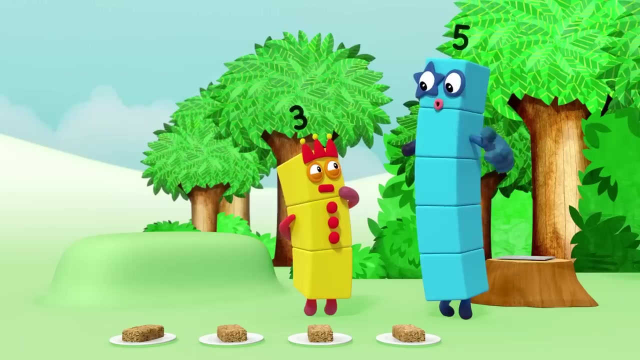 if you don't say them in the right order: one, two, three, four. you won't know how many there are. cruel one, two, three, four, three flapjacks- oh, we've been here before. rule three. the last number is how many? when you reach the last thing to count, the last number you. 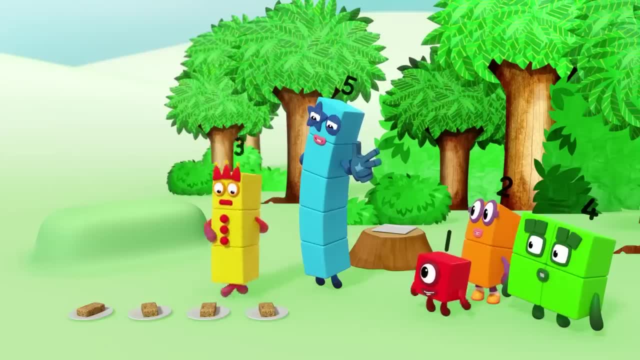 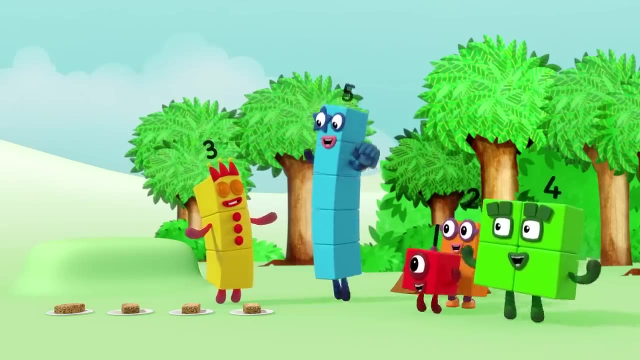 say, tells you how many there are. try, you can done one, two, three, four. that's the last flapjack, so four For Flapjacks, That's right. Hooray, I did it. I know how to count. One count everything once. 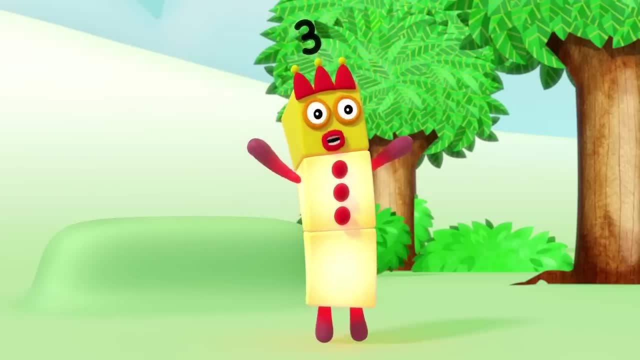 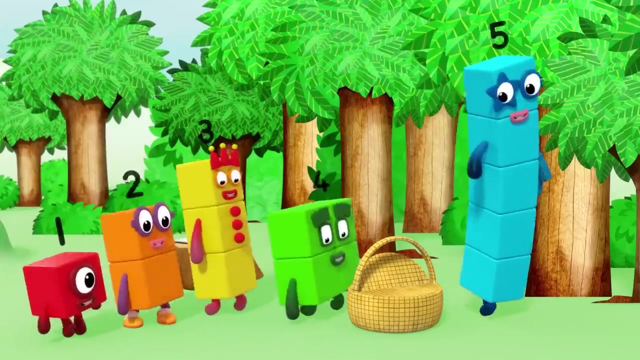 Two say the numbers in the right order. Three: the last number is: how many? Three rules of counting. All right, Let's celebrate with Flapjacks. I've packed an extra one for you. Five, Hang on, it's gone. 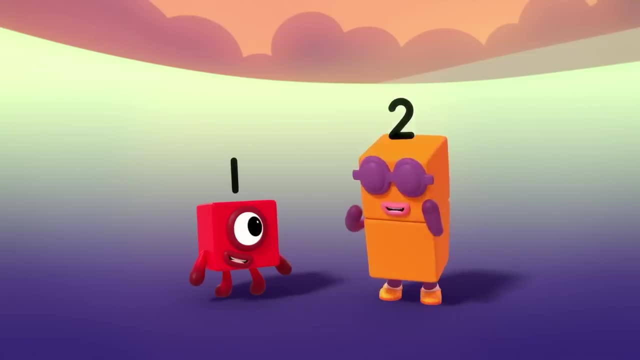 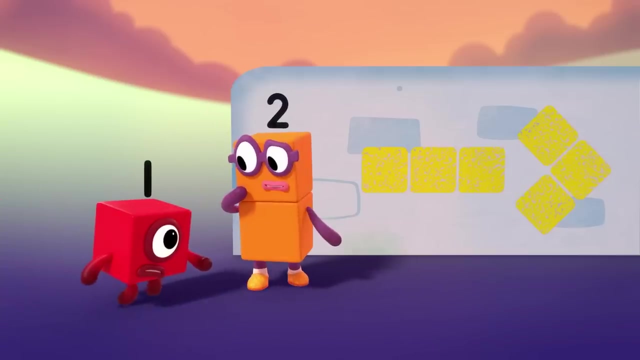 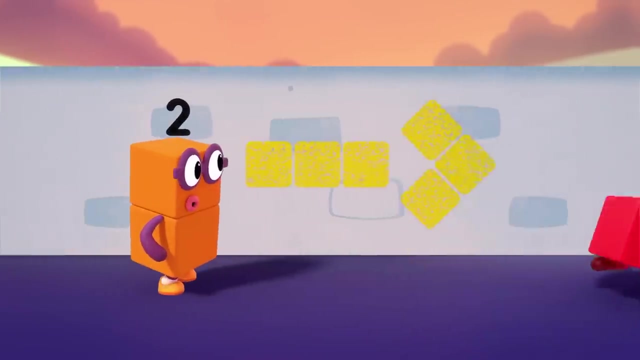 One, two And again One, two, Your turn One. I can't do it Right. What was that That way? Come on, Wait, Looks familiar. It's pointing to the sounds. Quick, Hey, it's four. 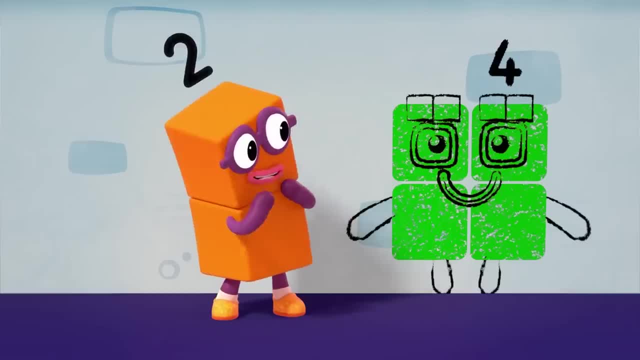 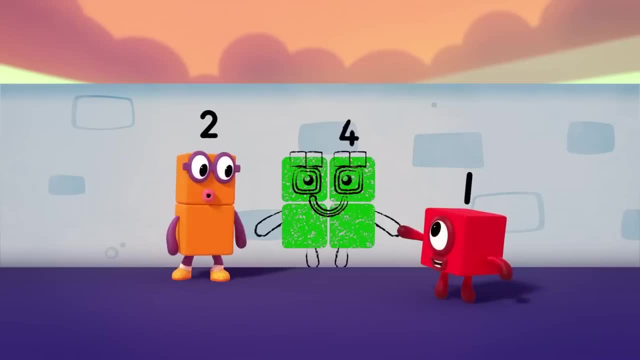 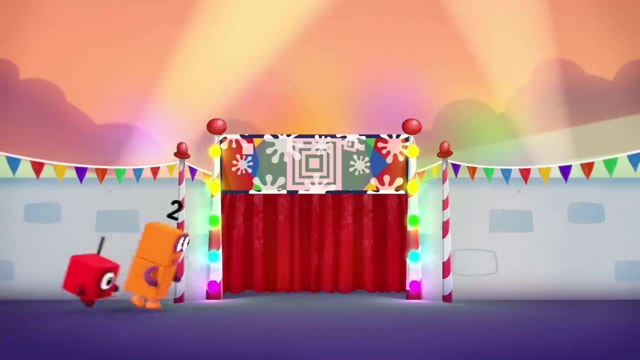 Four, Four, Four. Are we playing musicals Or are we playing with statues? A painting, A painting of four. I knew that, But what's that? Whee, Whee, Whee, Whee, Whee. 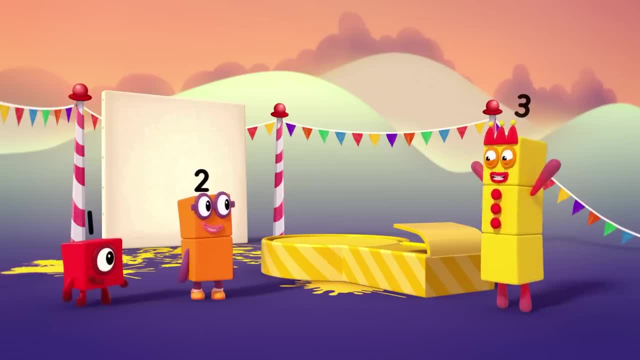 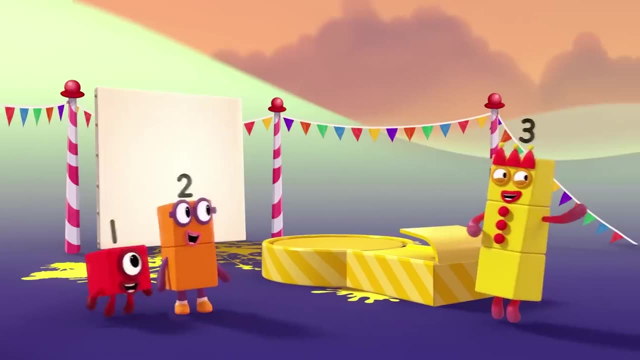 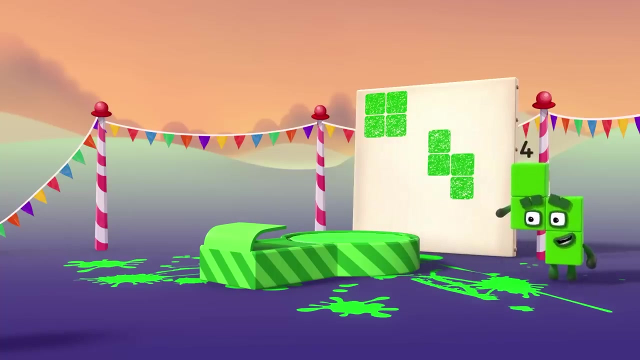 Welcome, welcome, welcome to my new Stumpoline Park. Don't you mean trampoline? No, no, no, Look, Look, Look, Look, Whee, Whee, Ooh, Ooh, Ooh. That was fun. 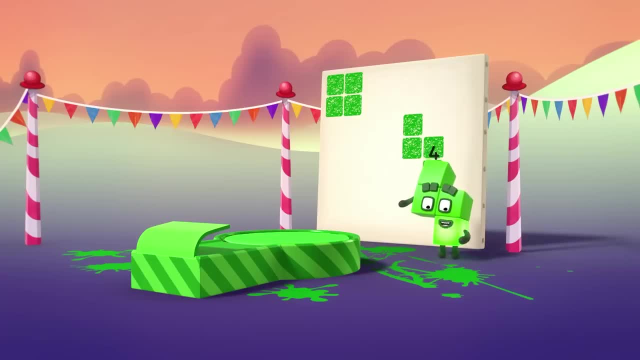 Four, Four Is that you? Of course, it is One, two, three, four, Four blocks. See Whee. Whatever way round I go, whee, I'm still four. Whee, Whee, Whee. 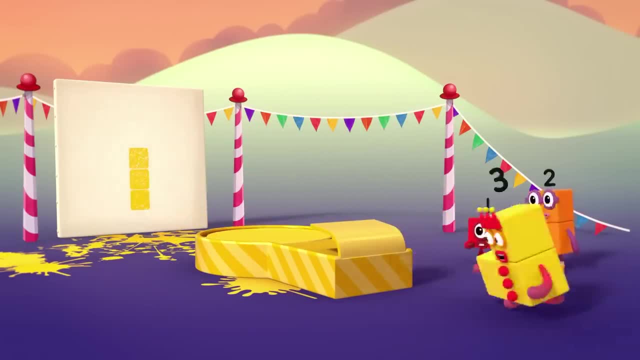 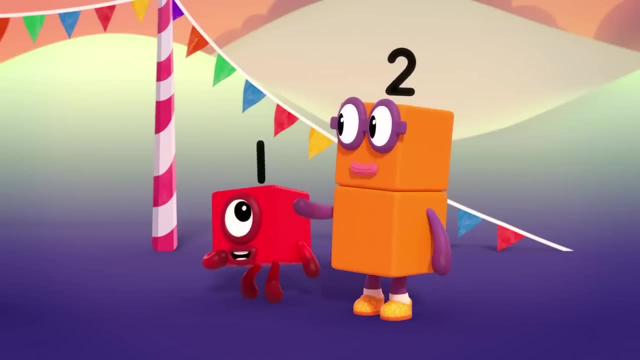 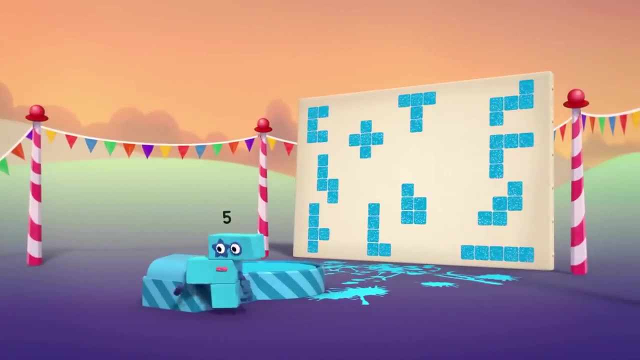 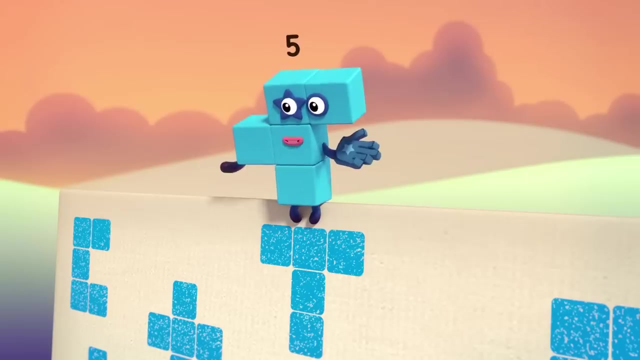 I'm still three. Whee, Ba-ba-ba. Ooh, Not bad. You think that's amazing. You should see five, Five. did you make all these shapes? I did so. The more blocks you have, the more shapes you can make. 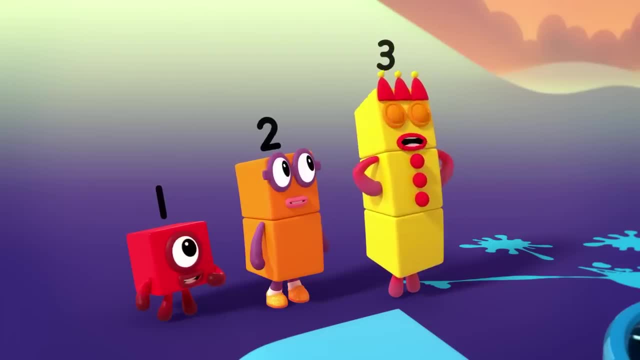 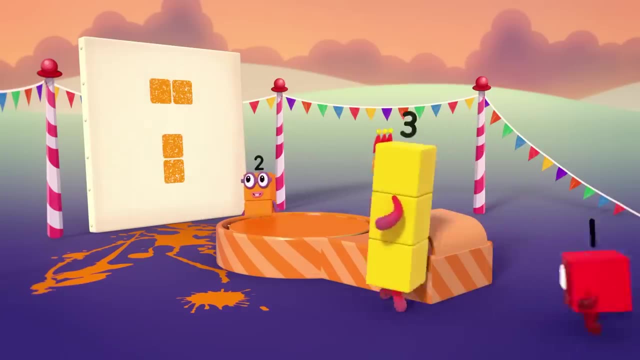 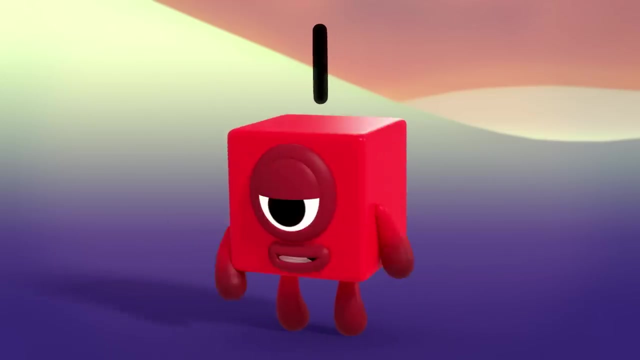 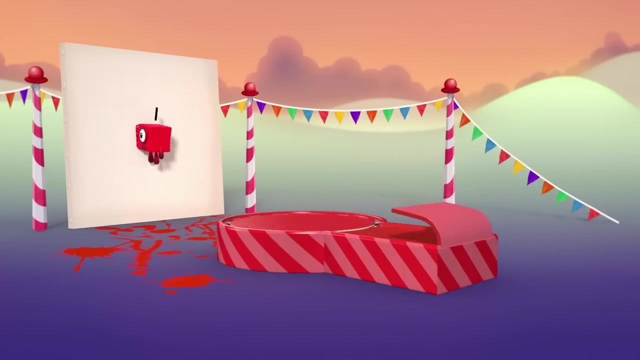 Oh, My turn. Not bad too. Of course, they're not really different shapes, are they? It's the same shape, one going up and one going across. Oh, It's still better than me Look. Oh, That's all. 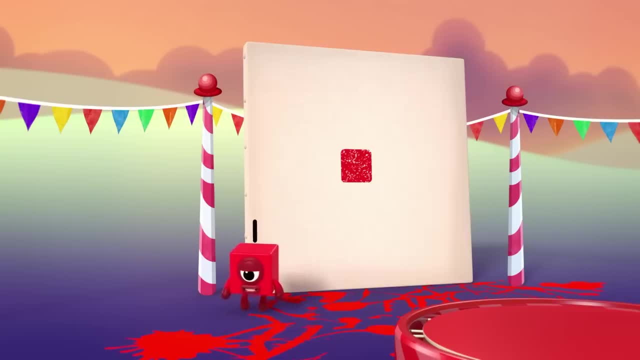 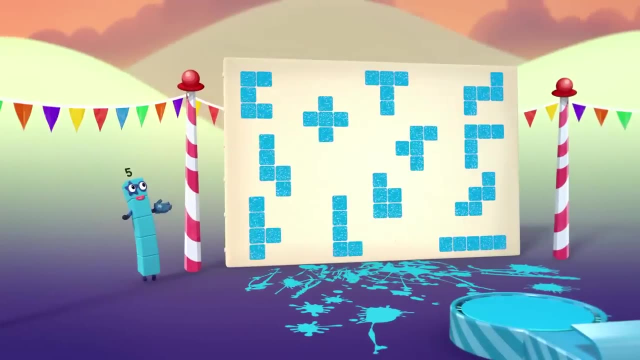 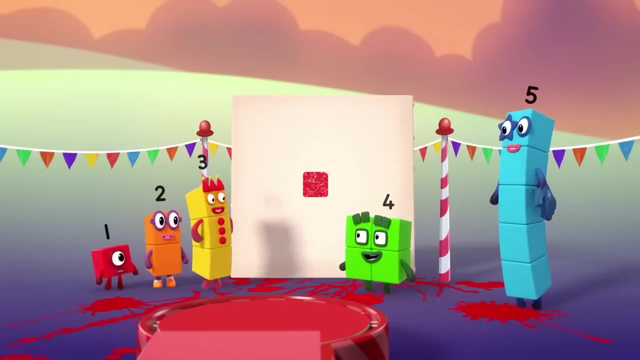 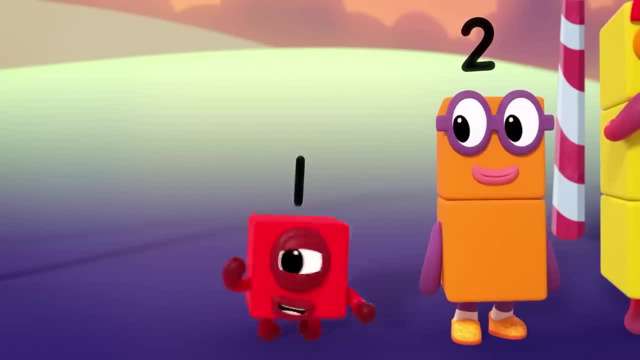 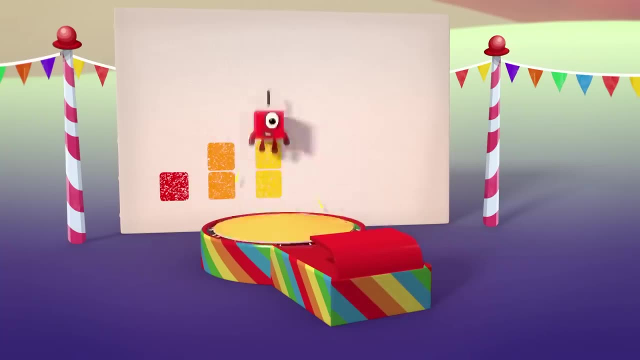 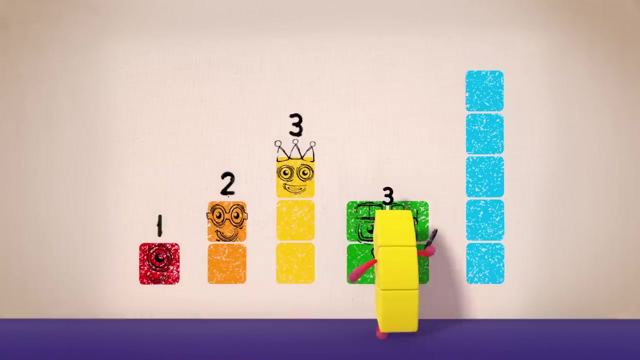 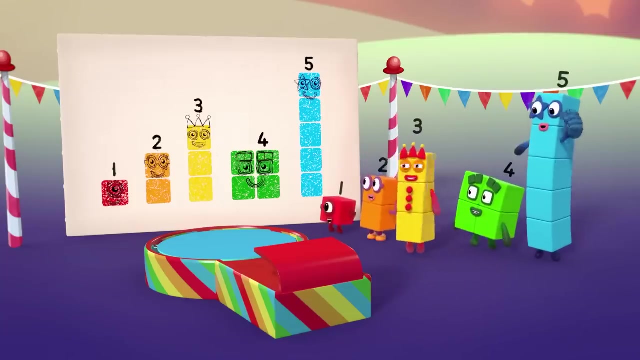 So lots of little ones can make every big shape. Look what I can do. Whee Ooh. You made all of us All right. Well done, And just in time for the grand finale, what better way to celebrate opening my new park? 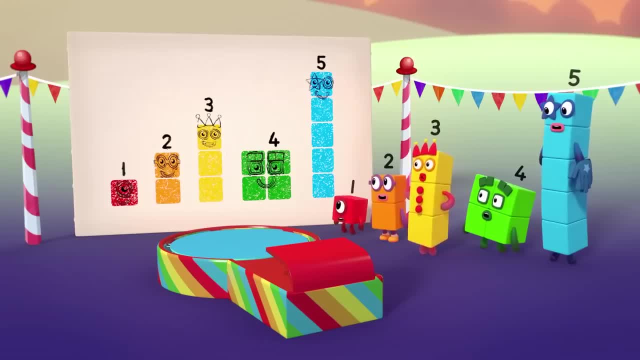 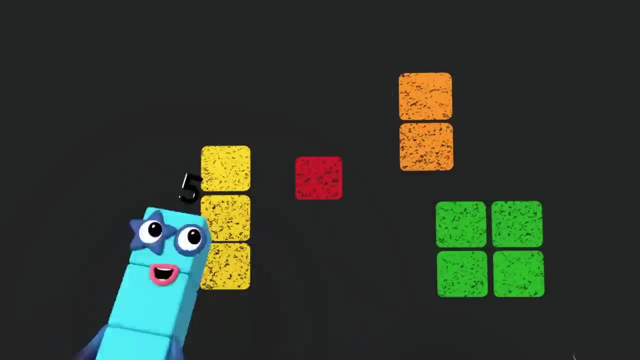 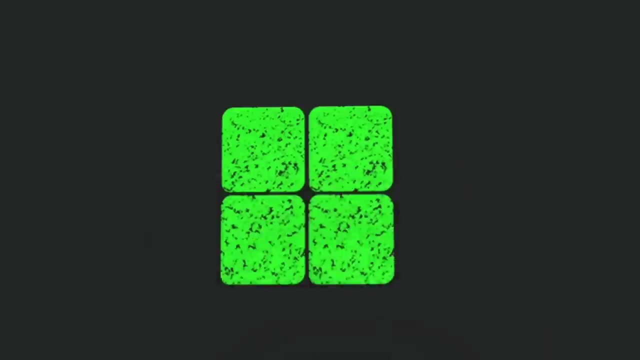 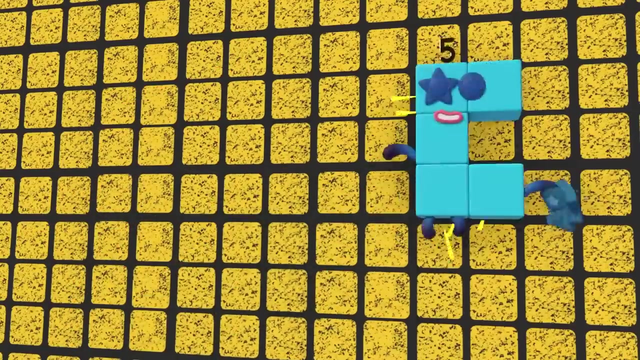 than with fireworks. Ooh, May I present the sky at night? Whee, Yay, Woo-hoo, Yay, Yes, Woo-hoo, Yeah, Ha-ha-ha, Yeah, Oh, You see one. 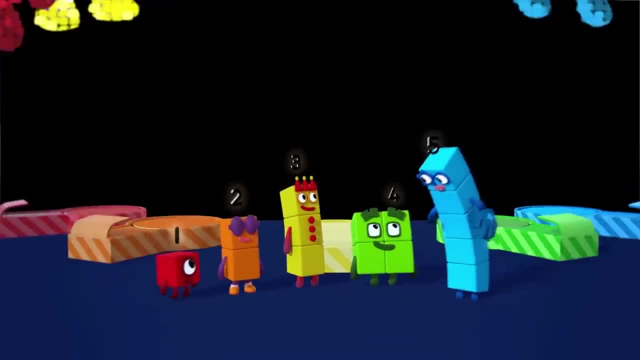 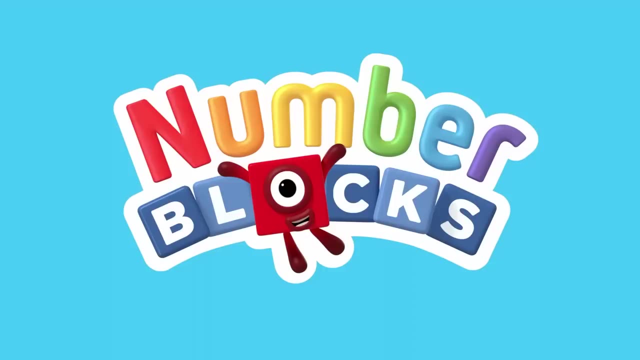 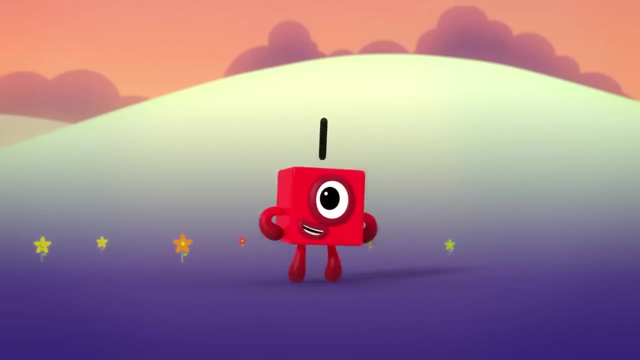 When we all work together, the sky's the limit. Ooh Yeah, I'm number one And this is fun. I've got one block to play with and the whole of me is one. One, One, two, one, two. 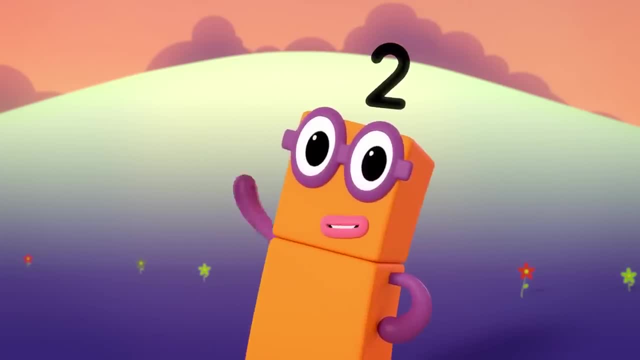 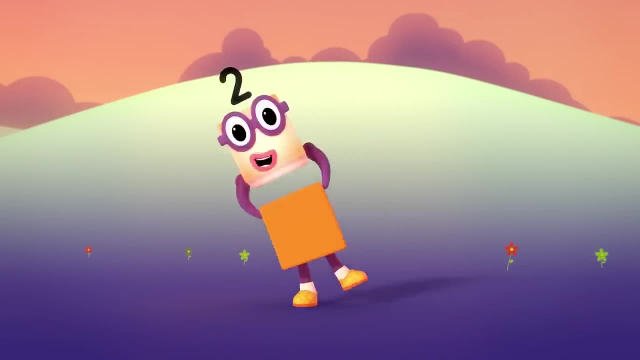 I'm number two. How do you do? I've got two blocks to play with and the whole of me is two. One, two. One is a part of me and one is a part of me, and the whole of me is two. 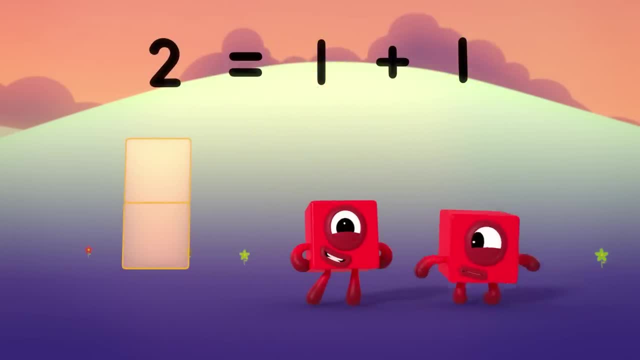 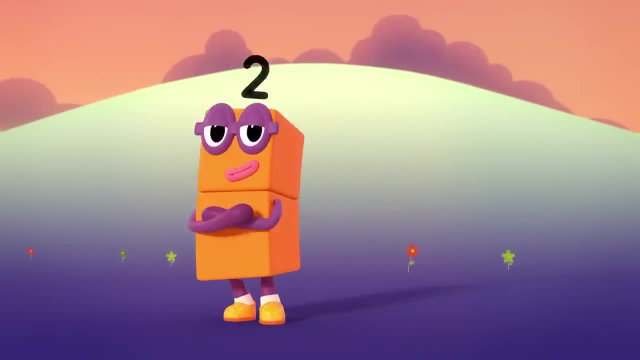 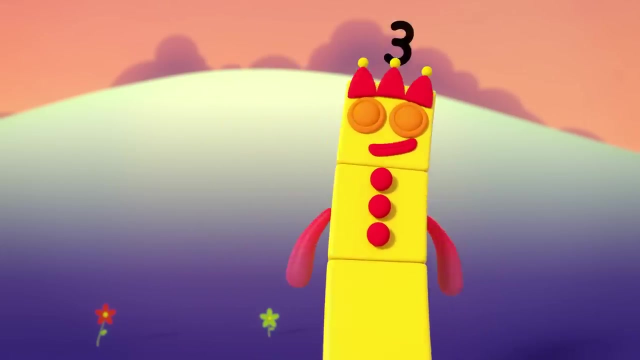 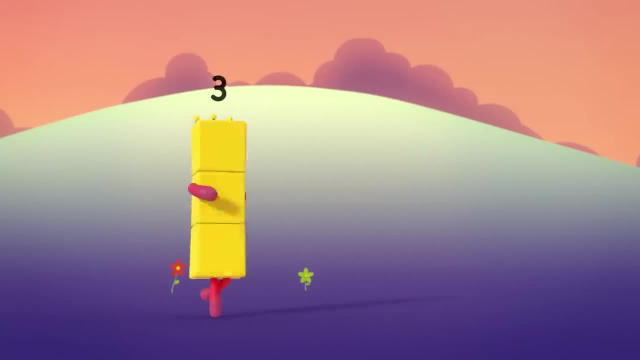 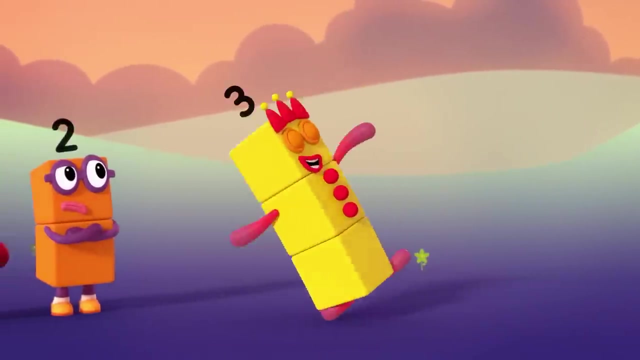 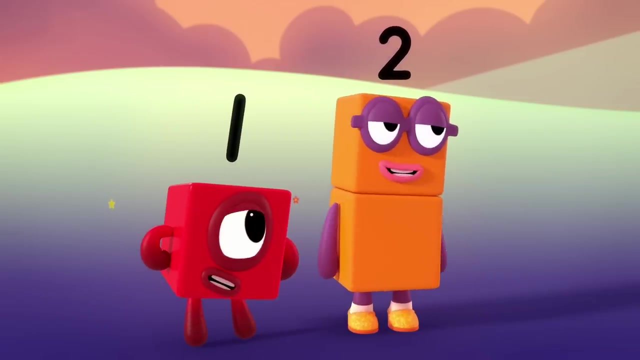 Now look at me. I'm the best of all the number blocks, as you can plainly see. The whole of me is amazing. The whole of me is so great. The whole of me is Sorry. Three, Try again, Okay. 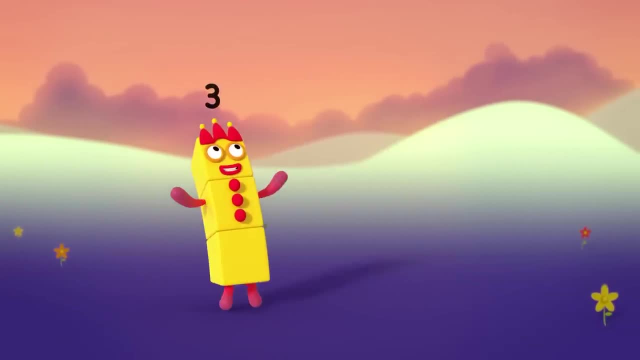 I'm number three. Yes, look at me, I'm the best of all the number blocks. Oh, you can't do it like that. Oh, you can't do it like that. Yes, I am. Oh darling, I'm number three. 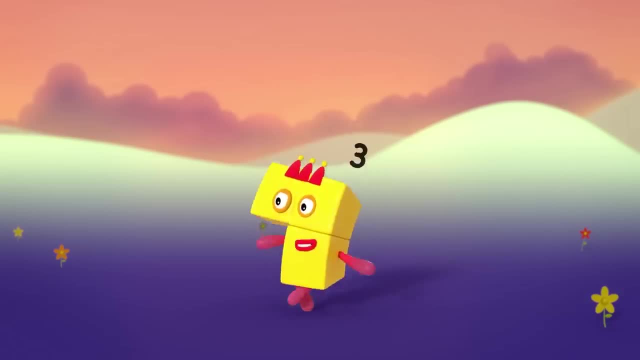 Now look at me. I've got three blocks to play with, and the whole of me is three. One, two, three, One, two, three. One is a part of me and two is a part of me, and the whole of me is three. 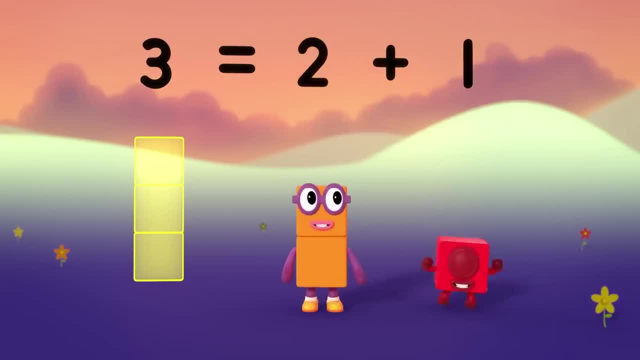 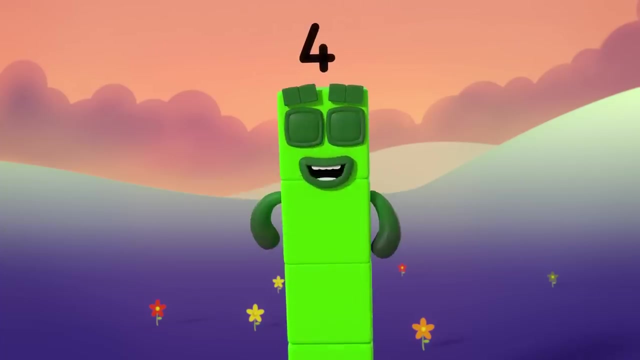 What? I'm two and I'm a part, I'm one and I'm a part, And the whole of me is three And the whole of me is three. One, two, three. I'm number four and I am sure. 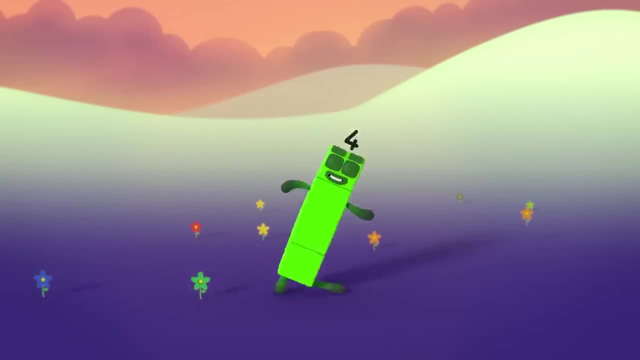 that I've got four blocks to play with and the whole of me is four. One, two, three, four. One is a part of me and three is a part of me and the whole of me is four. What? 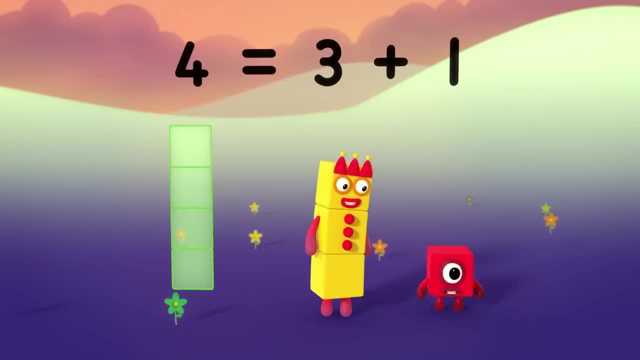 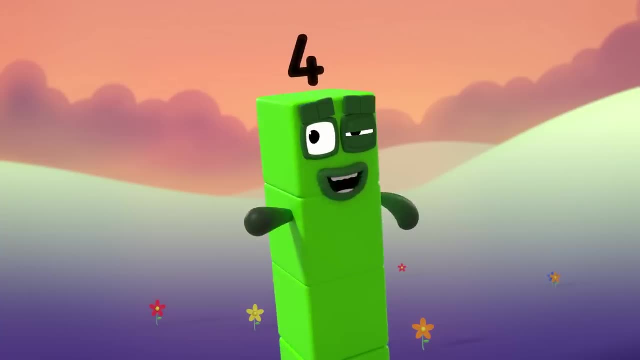 I'm three and I'm a part, I'm one and I'm a part, And the whole of me is four. Shhh, And the whole of me is four. Now, here is something more that's different from before. 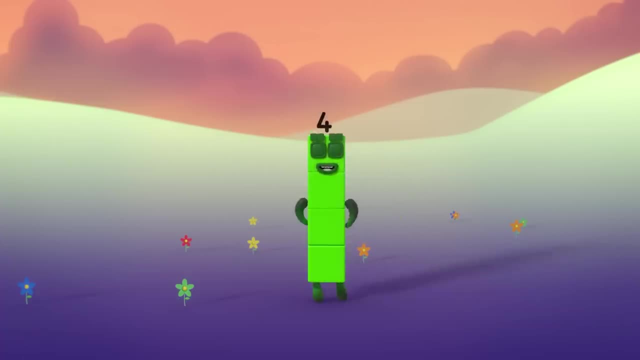 Two is a part of me, It's a part of me, And the whole of me is four. Watch, I'm two and I'm a pot. I'm two and I'm a pot, And the whole of me is four. I'm a square, look. 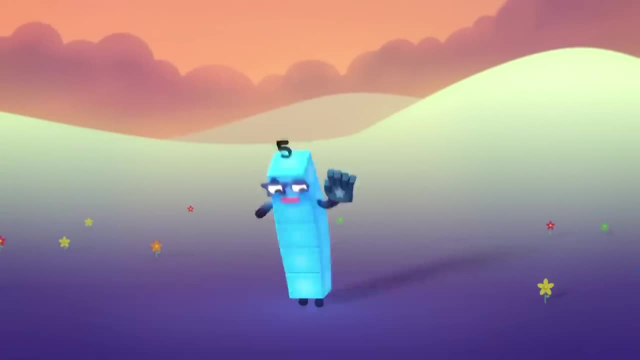 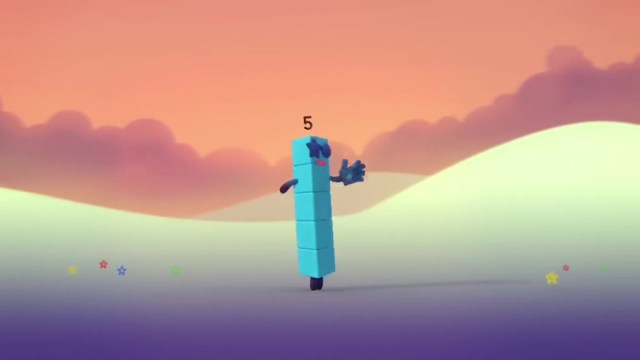 Four sides, four corners. I'm number five, I am alive. I've got five blocks to play with And the whole of me is five. One, two, three, four, five. One is a part of me And four is a part of me, And the whole of me is five. 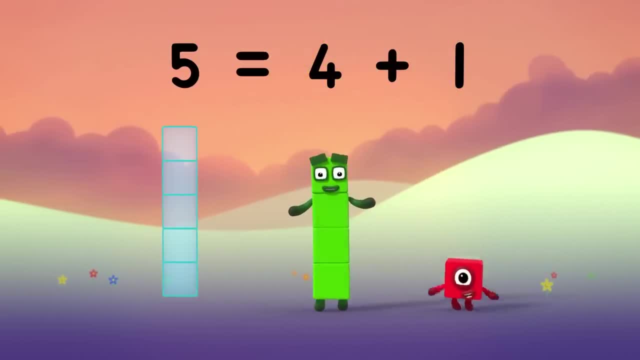 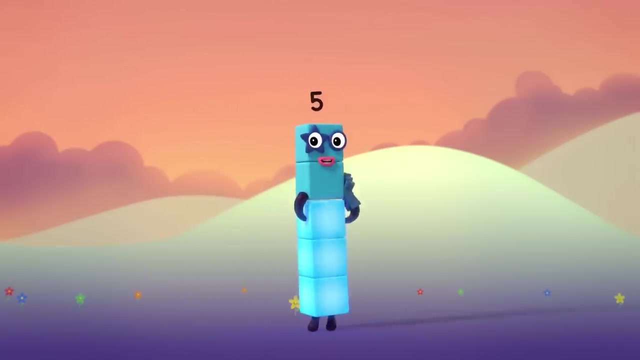 Watch, I'm four and I'm a pot, I'm one and I'm a pot And the whole of me is five. But now I feel alive going into overdrive. Two is a part of me, And three is a part of me, And the whole of me is five. 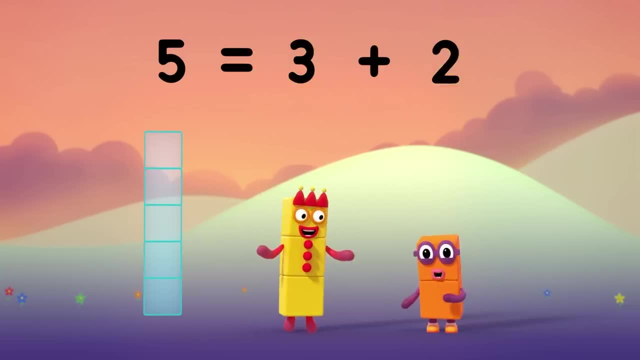 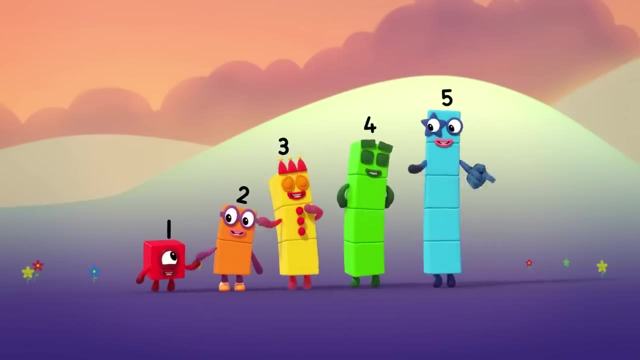 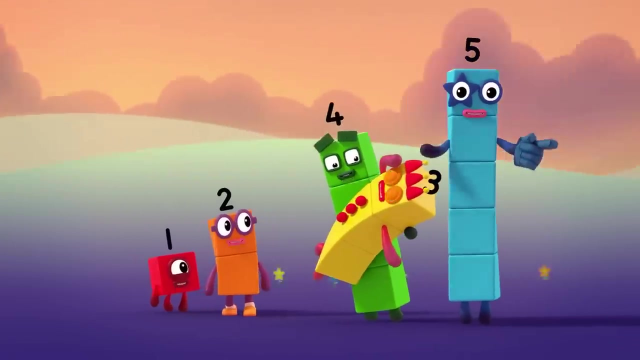 Watch, And three And I'm a pot, I'm two and I'm a pot And the whole of me is five High five. Making friends is easy when you can come apart. Splitting up is not so hard. it won't break your heart. So when we fall to pieces, we have lost control. 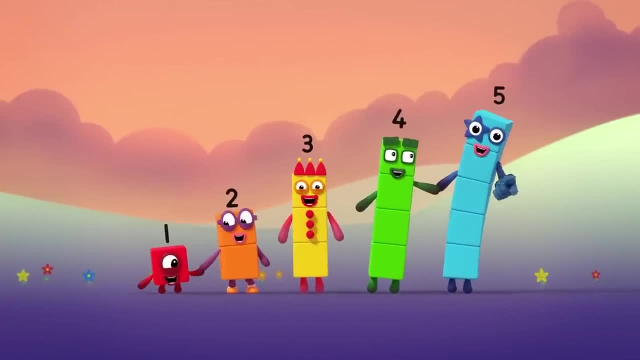 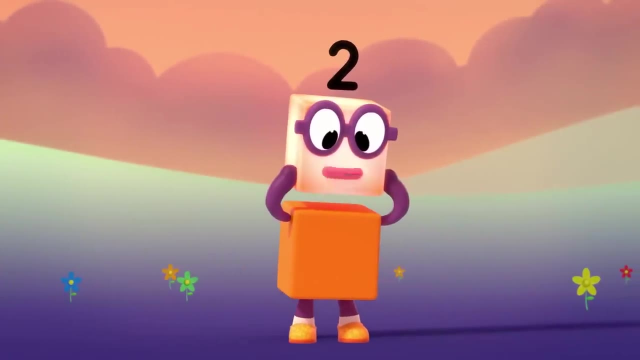 A hole is made of all its parts And the parts they make of the whole. Just remember that One is a part of me And one is a part of me. One is a part of me And two is a part of me. One is a part of me. 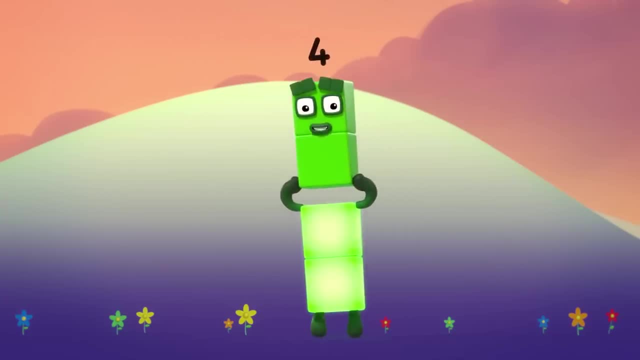 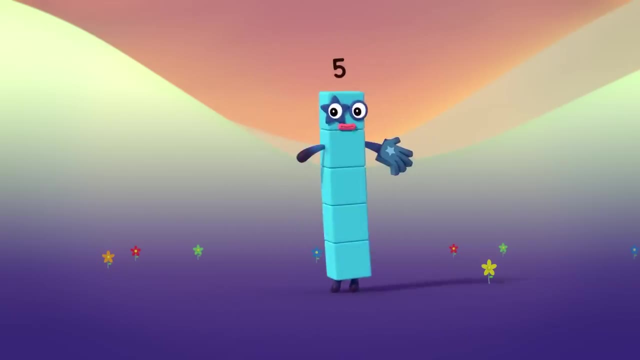 And three is a part of me, Two is a part of me And two is a part of me, One is a part of me And four is a part of me, Two is a part of me And three is a part of me And the whole of me is. 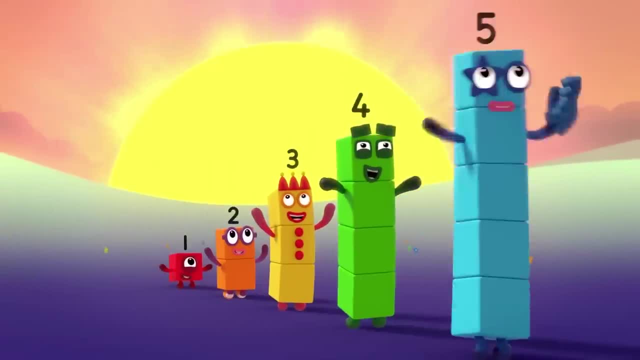 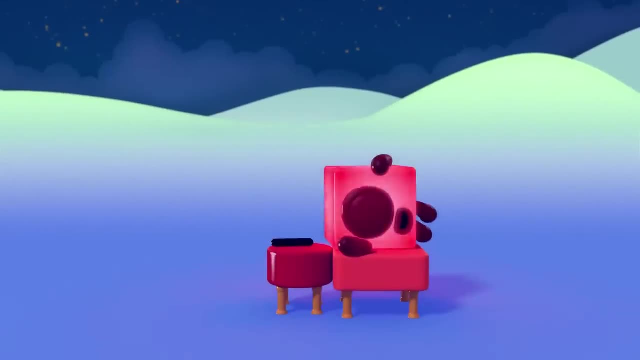 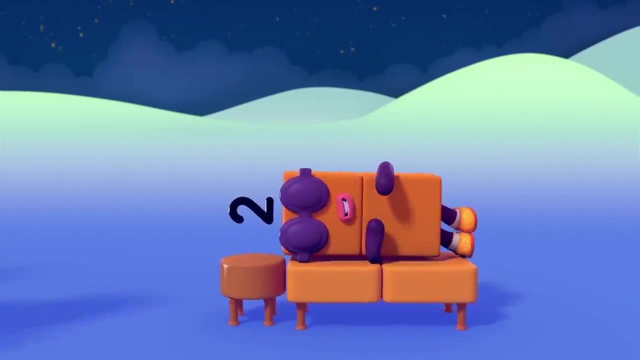 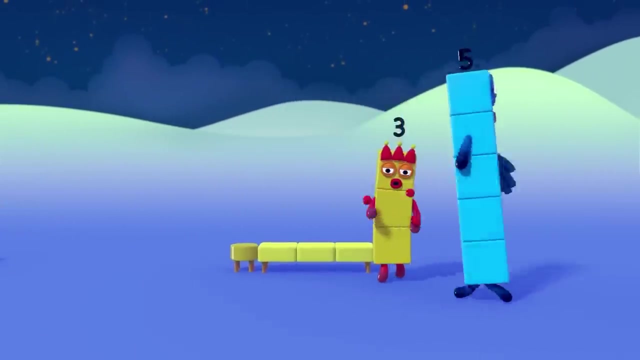 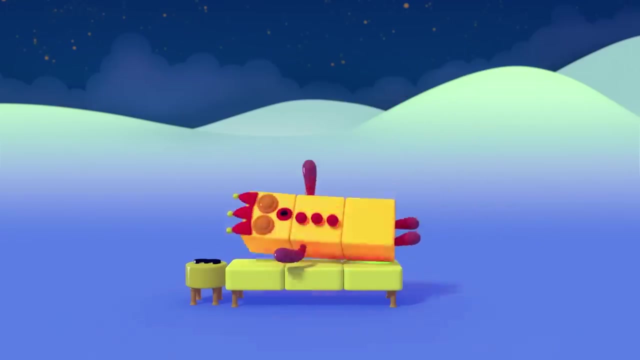 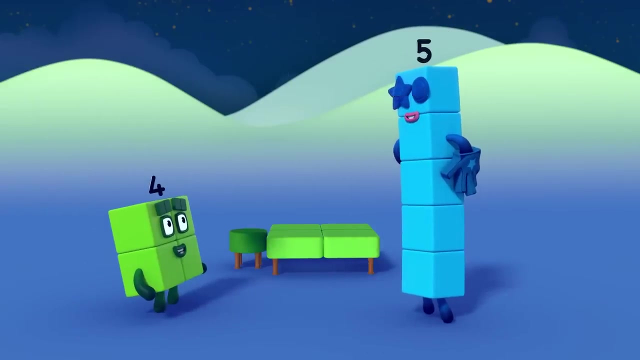 One, two, three, four, five. Night night. Oh, tired, tired, tired. It's time for bed. Four, I know. Oh, stay up, Go to bed. Make up your own mind: Stay up or sleep. Stay up or sleep. 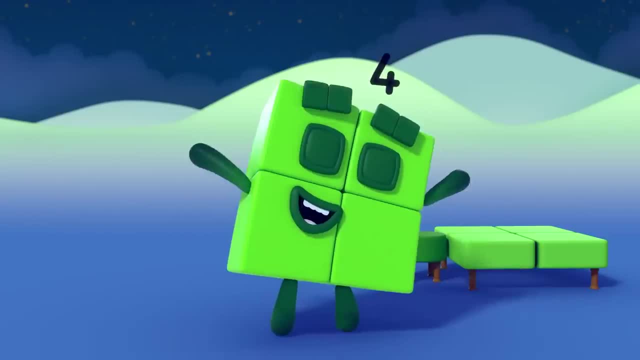 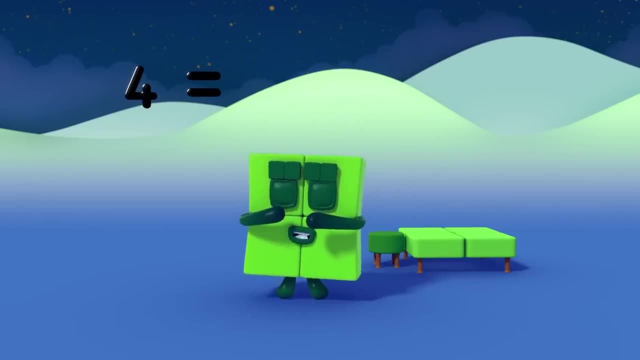 I can't do both. Ugh, He can. No, no, no, no, Not you two. Four equals two plus two. You look like me, I look like you. We're two of a kind. We're the Terrible Twos. 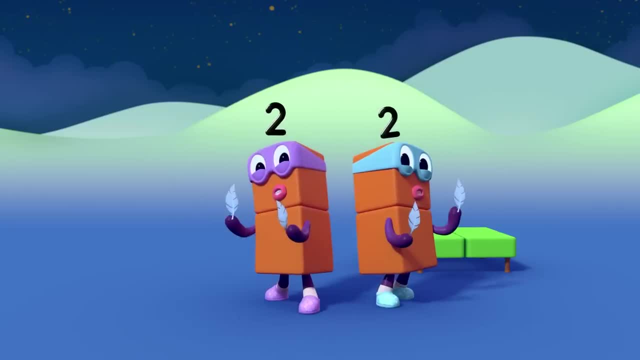 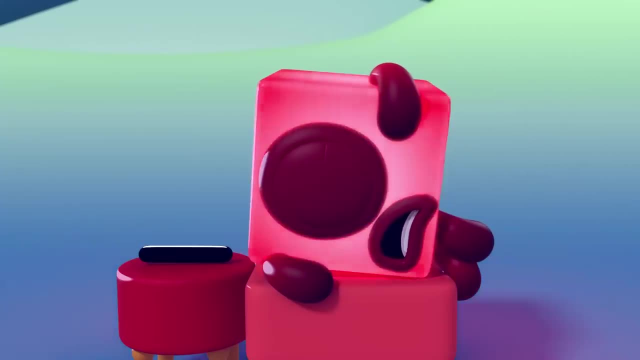 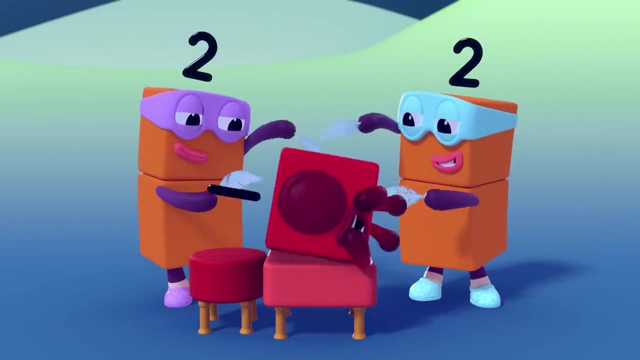 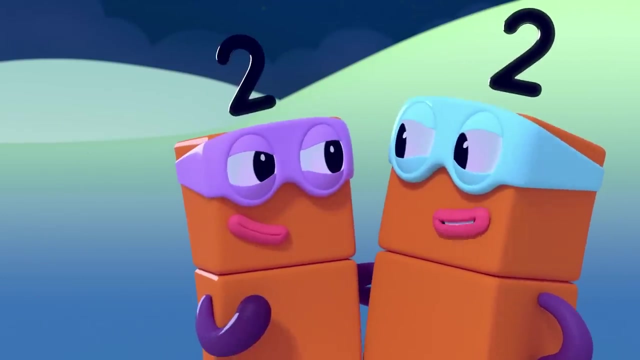 Yeah, Two, lots of two feathers. It's tickling time. One, two, One, two, Tickle, tickle, Tickle, tickle. Oh, is someone there? Not someone, Some twos, And we're both here to say: 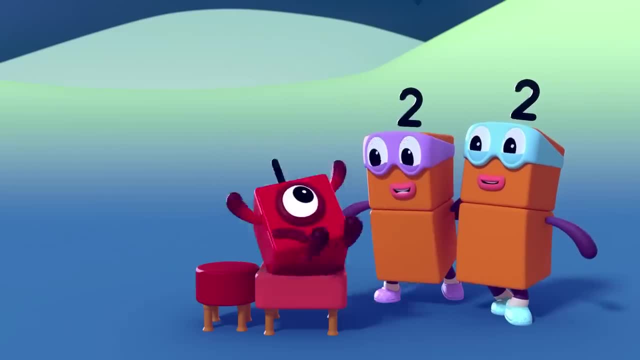 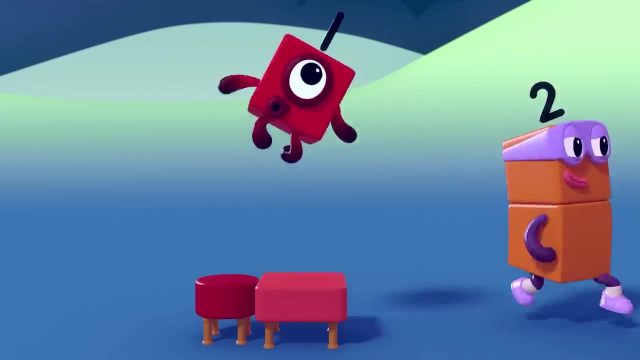 Two of a kind, Two of a kind. Boo Oh, Oh, Oh, That was fun. Let's do it again. Woo-hoo, Yeah, Oh, Oh, Hee-hee. He reminds me of someone, Amigo. 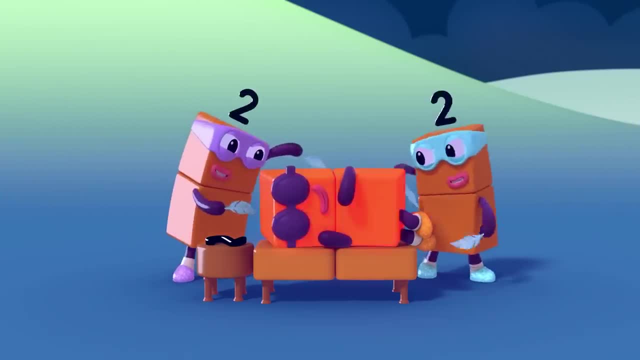 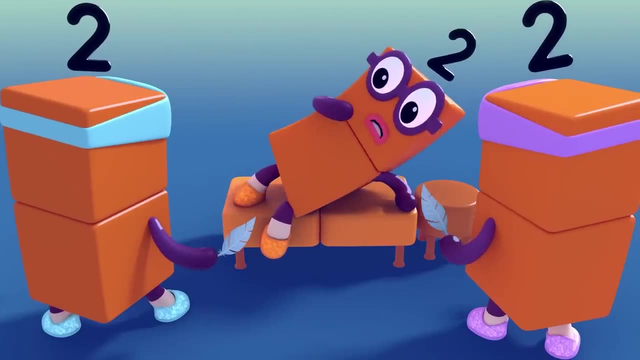 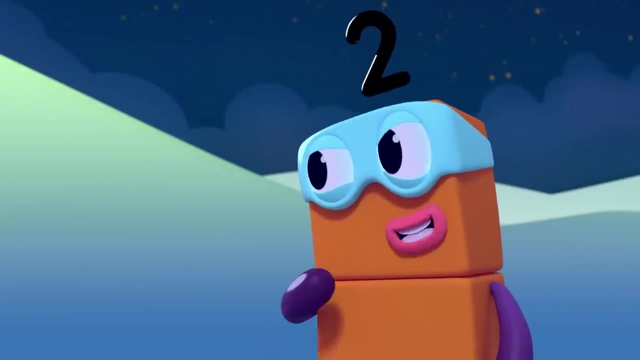 Can't think who, Amigo, Tickle, tickle, Tickle, tickle, Ugh. Another me, Doubler, Another another me, Him, me and you are two minutes away. So it's time for the both of us to say: 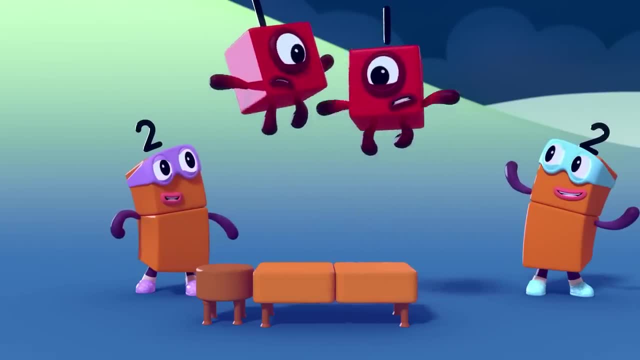 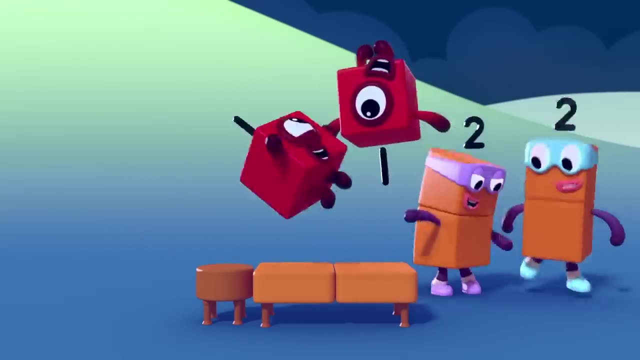 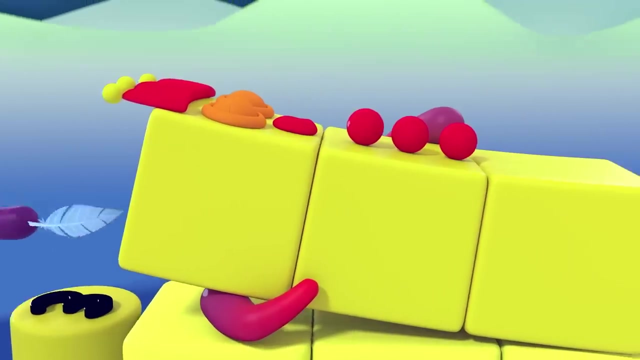 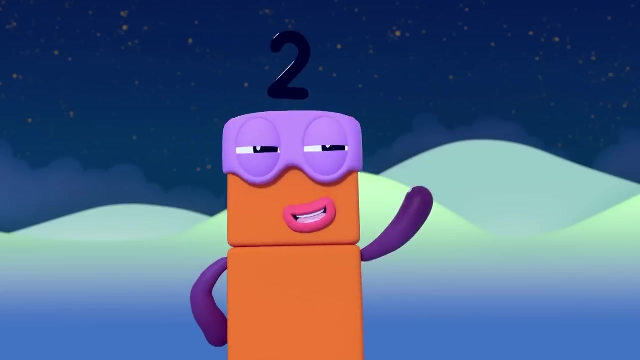 Boo, Oh Oh, Two, twos, two ones. It's time to be gone. Yeah, Oh Oh, Oh, Hee-hee, Woo-hoo, One, two, Three. Bum-bum-bum. Looks like fun. Let's try it too. 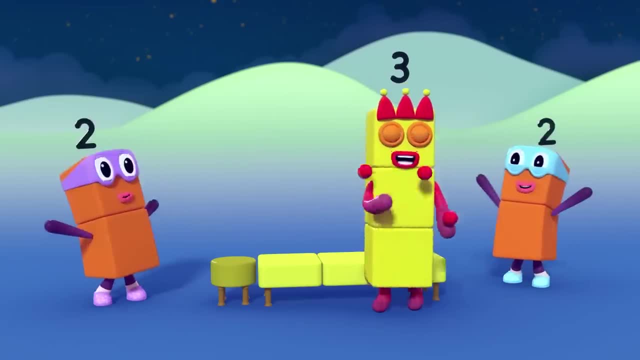 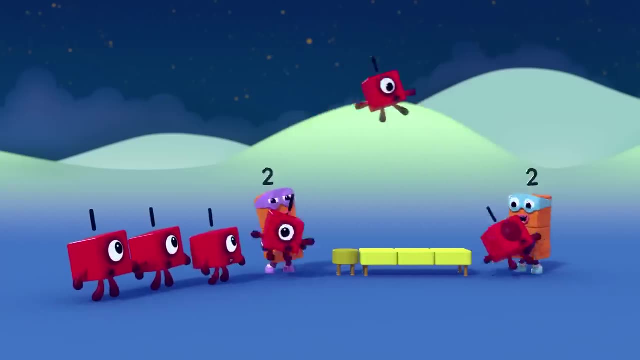 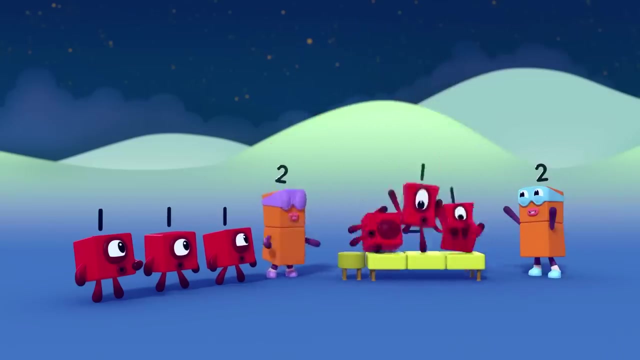 Just as soon as we both say Boo Hey, Oh, Oh, Oh, Oh, Oh, Oh, Hey, stop Huh. Oh, A terrible two say Boo Toodle-loo, Oh Oh Hey. 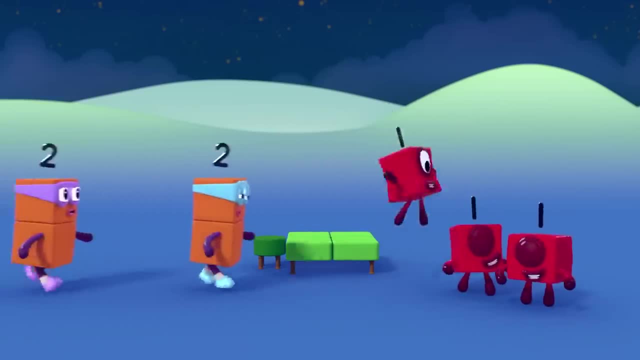 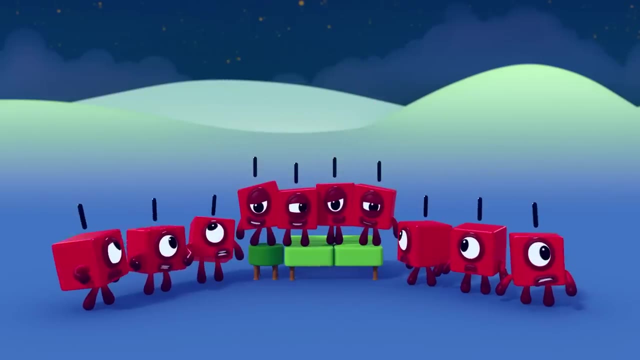 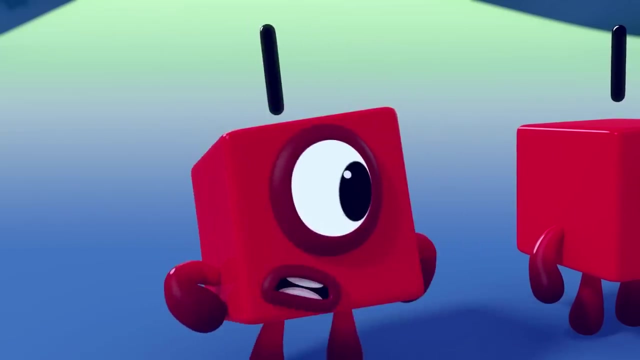 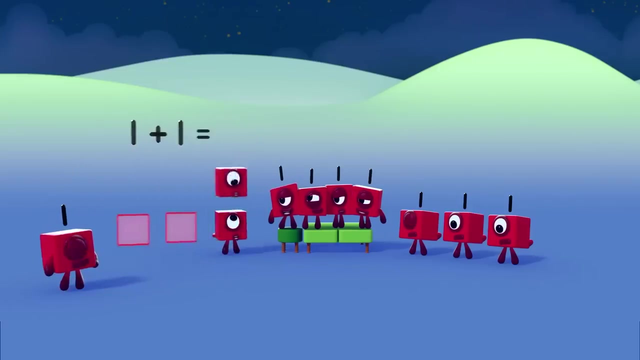 Oh, Oh, Oh, Oh, Oh, Oh, Oh, Everyone, pull yourselves together. One, One block. One plus one equals Two. Two is two ones. One plus one plus one equals three. Three is three ones. 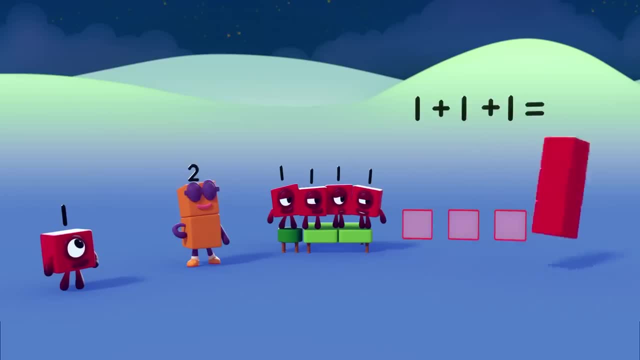 Two is three ones. Two is three ones. Three is three ones. One plus one plus one plus one equals Four. Four is four ones. Where are they? Where did those terrible twos go? Don't look at me. 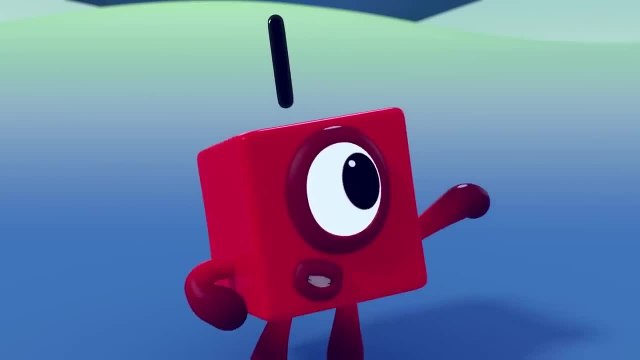 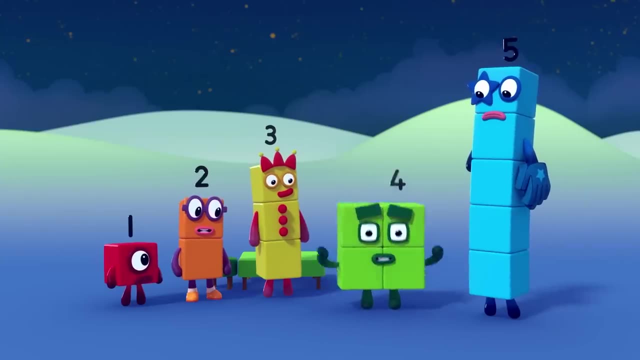 What's all of the noise? The terrible twos are playing tricks on us. And where are they now? I have to be square with you. They made me. What did they make you? You can tell us Four. No, they made me. 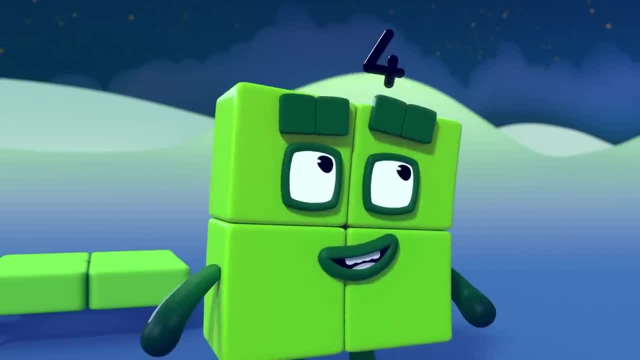 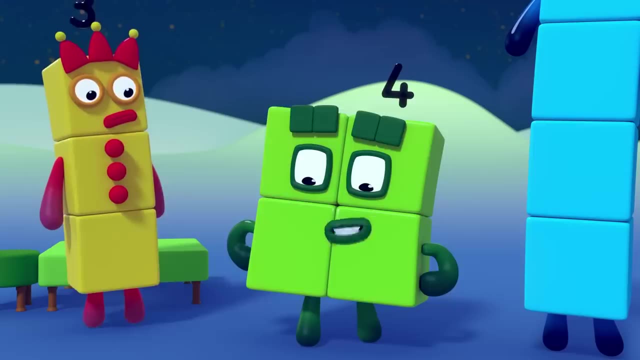 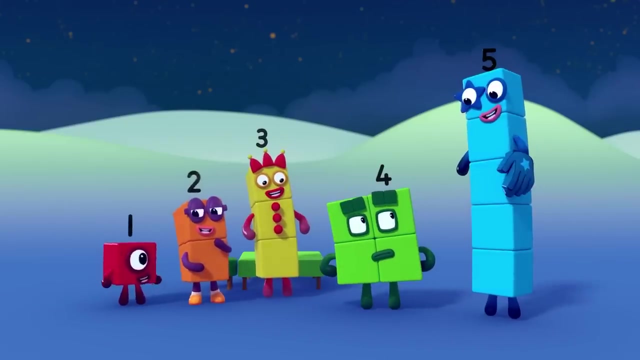 Well, I made them, Then they made me. Huh, I'm the terrible twos, I'm four lots of one, but I'm also two lots of two. You're funny, Don't be silly. That's a very funny joke. 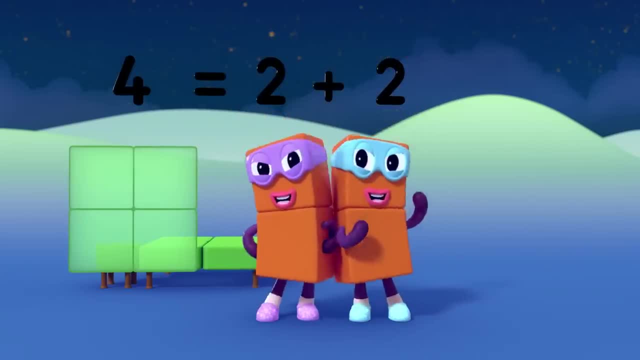 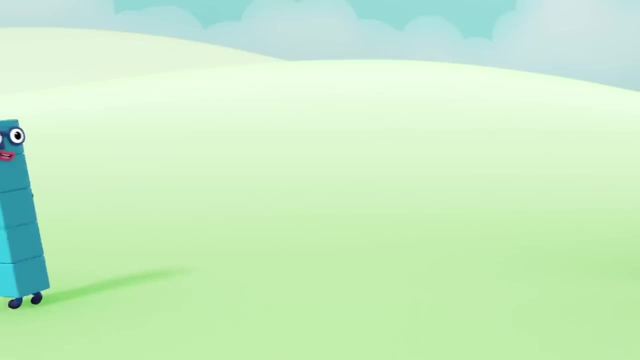 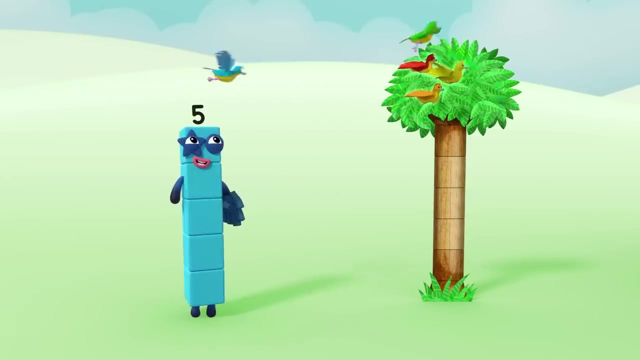 Four equals two plus twos. The terrible twos, Shhh, One, two, three, four, five. Here I am, I am five. One, two, three, four, five. Five little birds have just arrived. 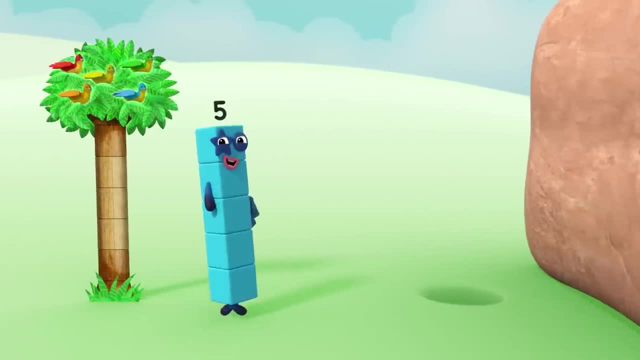 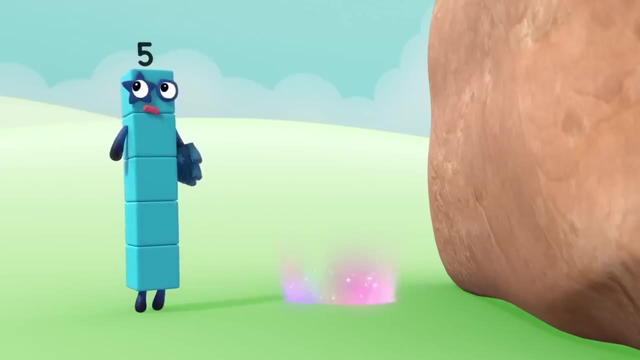 One, two, three, four, five. What a wonderful day to be alive. A giant rocket. Look in front of me. How can I get where I need to be? What is that silly sucking sound? Oh, look a hole. so big and round. 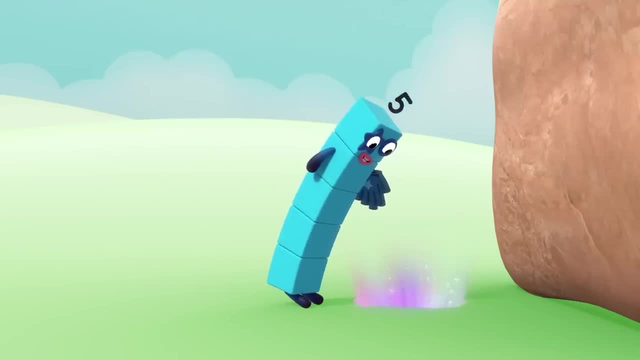 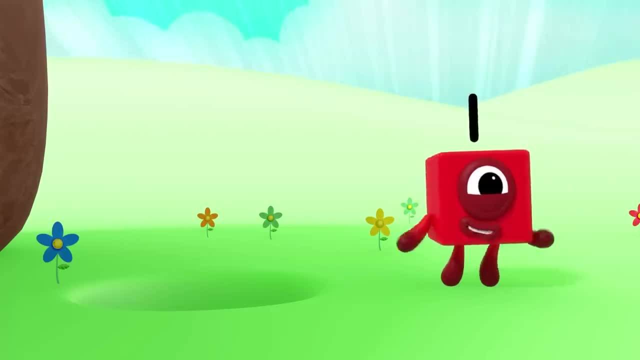 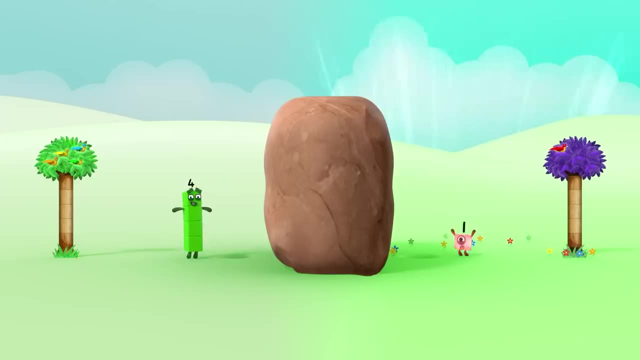 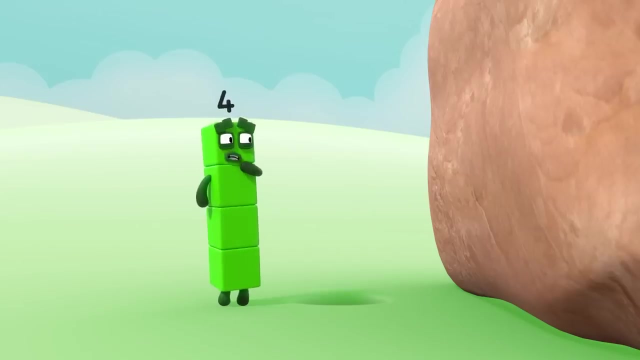 Woo-hoo, I am one. That was fun. Now I am four, and here I am. I am one, Here I am. What a wonderful day to be alive. Where, oh, where, oh, where is five? Five is gone. Where did she go? 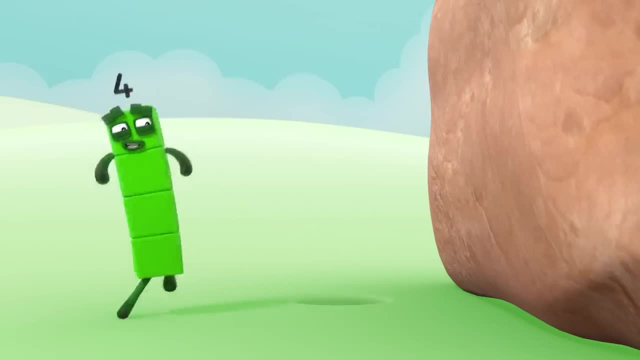 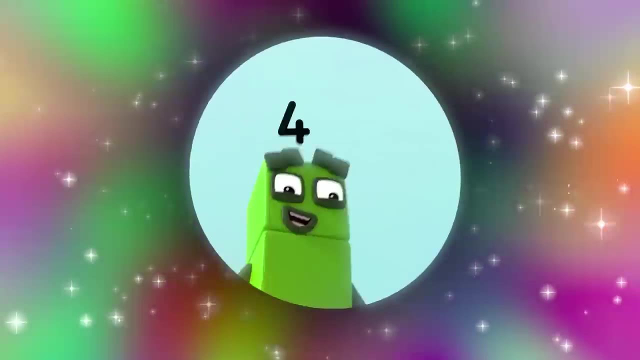 Is she all right? I do not know. Is she here, Is she there? I must keep looking everywhere. What is that silly sucking sound? A giant hole so big and round. Why is it there? I do not know. I wonder what is down below? 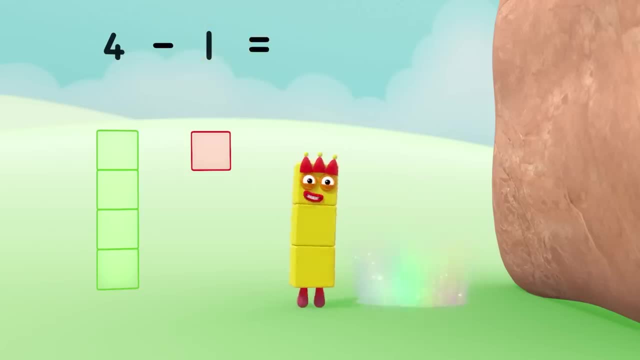 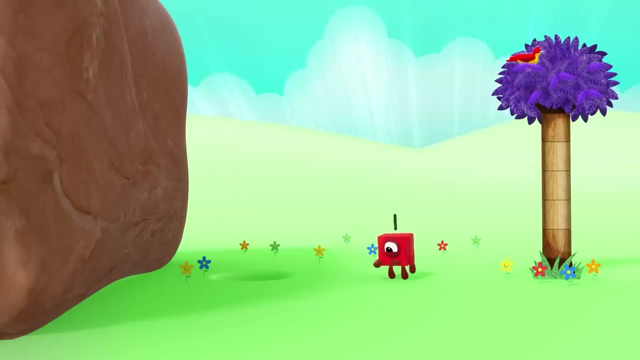 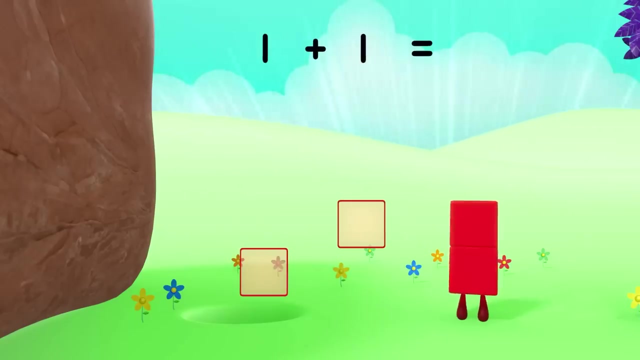 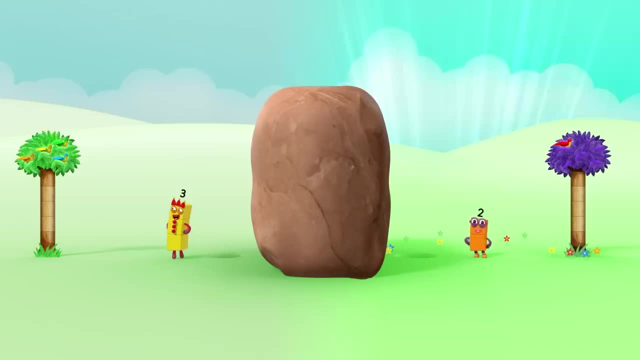 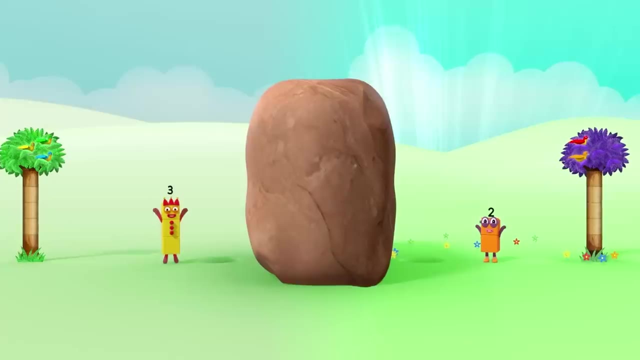 What is happening to me? I just got bigger, Did you see? Now I am three and here I am. Now I am two and here I am. What a wonderful day to be alive. But where, oh, where, oh, where is five? 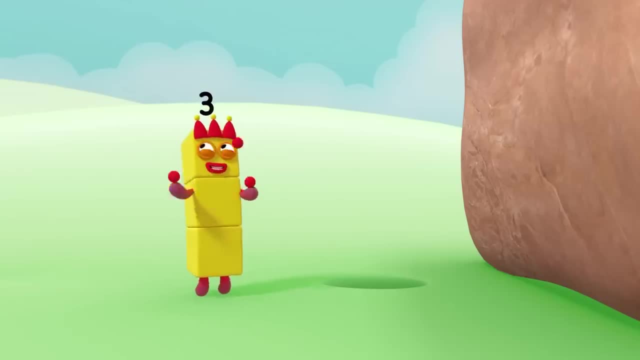 I was five, then four, then three. Someone has played a trick on me. I do not mind at all. you see, Three is who I want to be. What is that silly sucking sound? A giant hole so big and round. 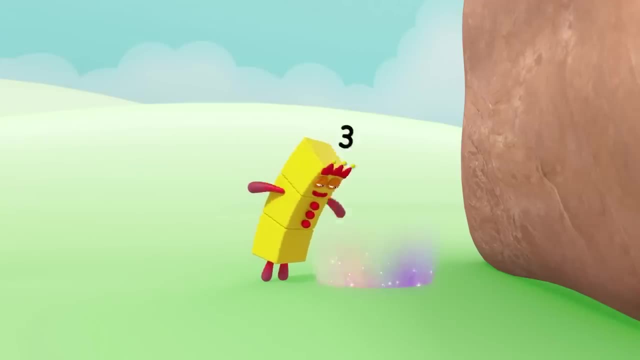 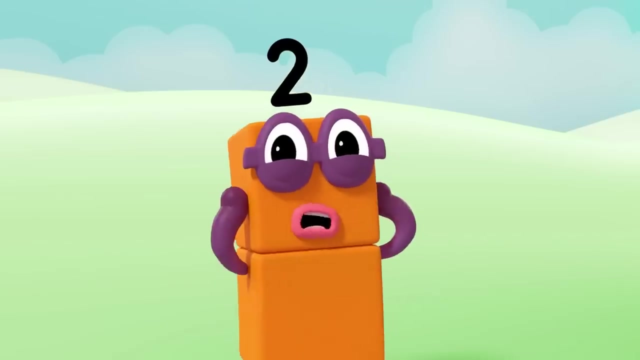 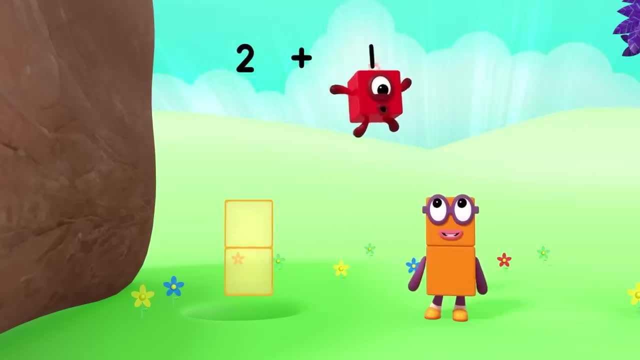 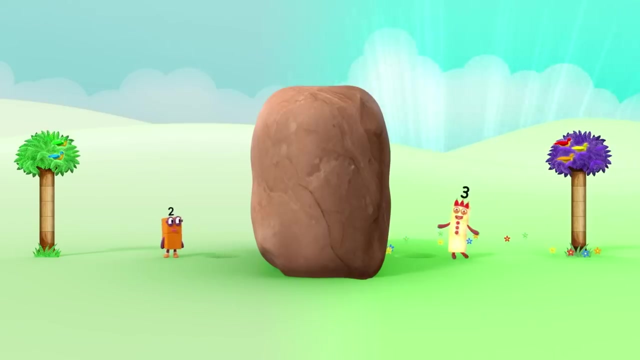 I am one. That was fun. Two plus one equals three. What is happening to me? I just got bigger, Did you see? Now I am two, and here I am. Now I am three, and here I am. 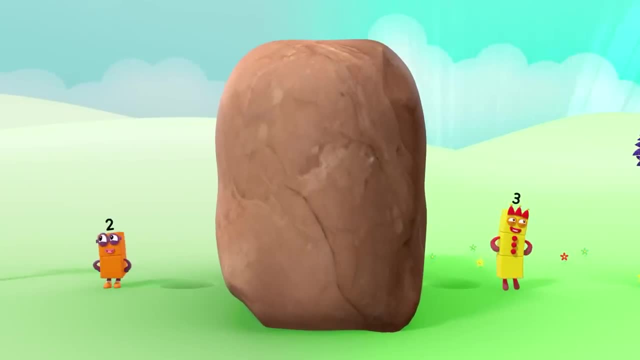 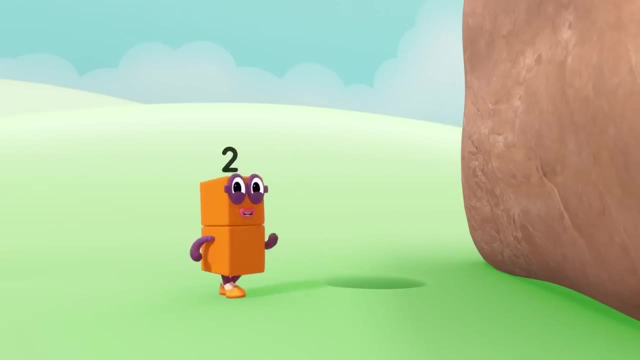 What a wonderful day to be alive. But where, oh where, oh where? is five? I wonder where the ones will go. I think I've got it Now. I know Every time we get one smaller, someone else is getting taller. 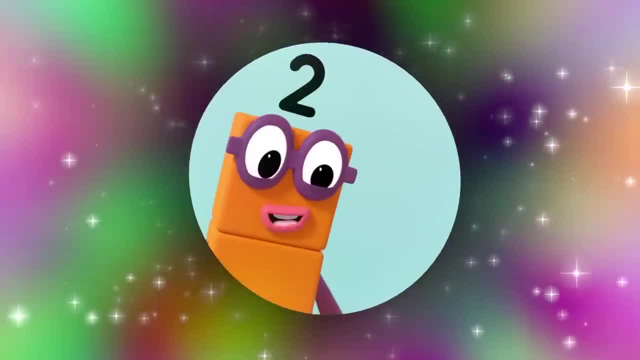 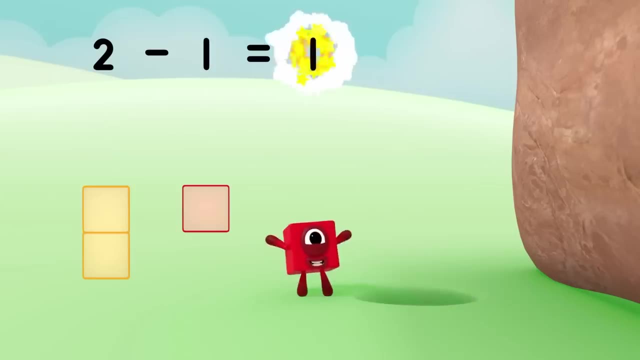 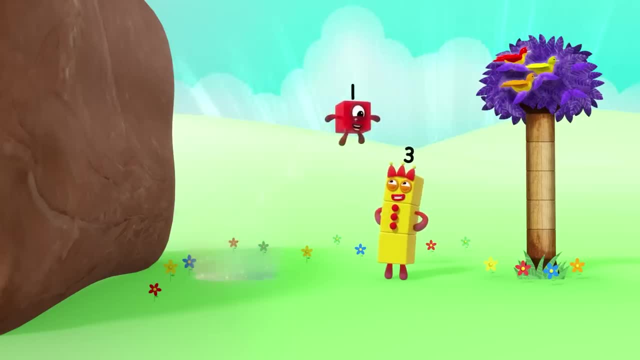 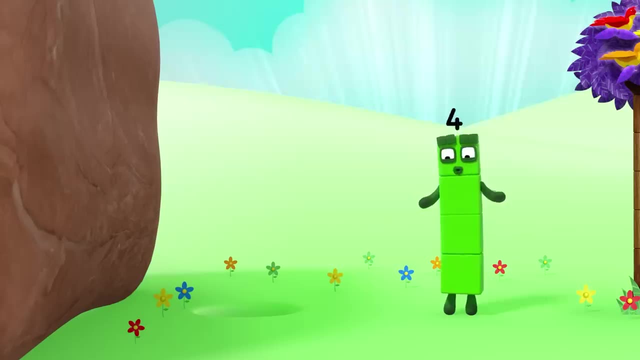 Where did it go? I am one. That was fun. Three plus one equals four. What is happening to me? I just got bigger, Did you see? What is happening to me? I just got bigger, Did you see? 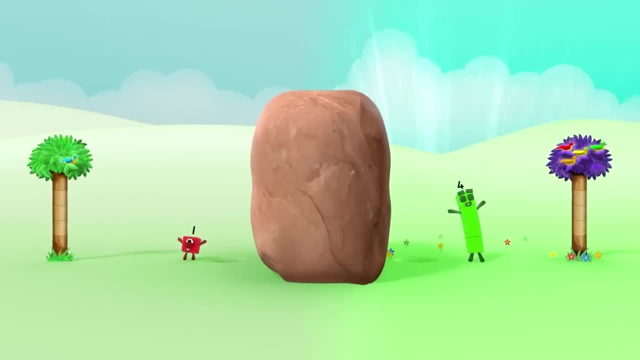 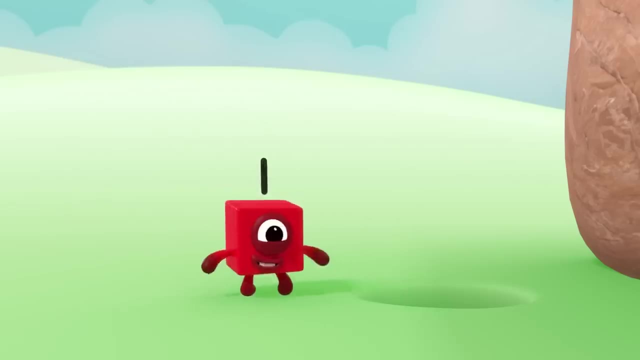 Now I am one, and here I am. Now I am four and here I am. What a wonderful day to be alive. But where, oh where, oh where? is five, Five, four, three, two, one, Someone's having lots of fun? 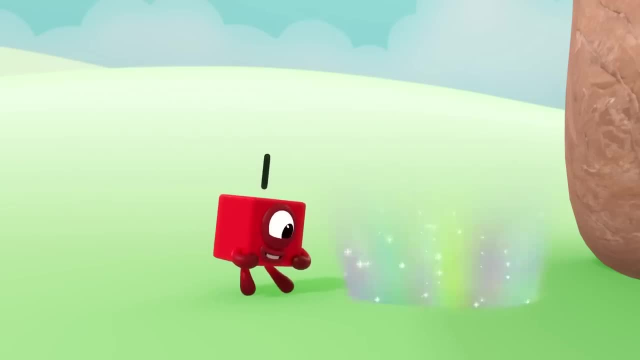 Now I know where five will be. Four is waiting there for me. What is that silly sucking sound? A giant hole so big and round? Why is it there? I think, I know. I think I know what's down below: Woo-hoo. 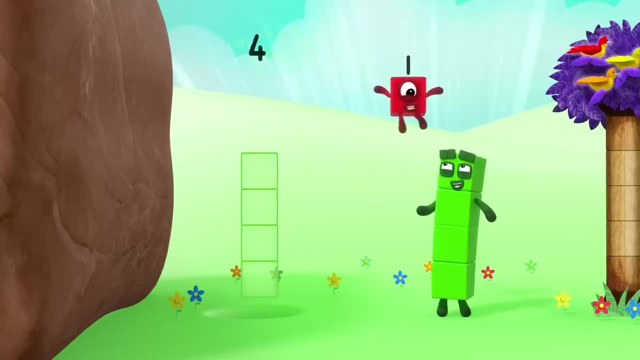 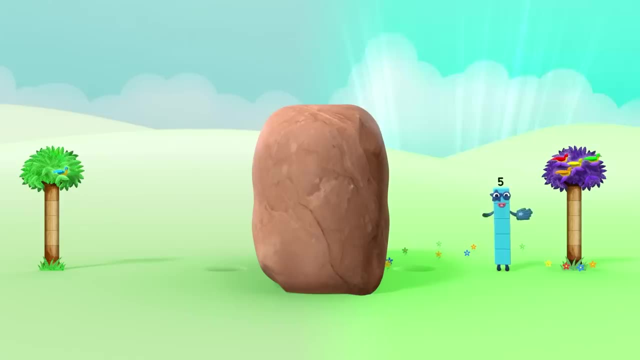 I am one. That was fun. Four plus one equals five. What is happening to me? I just got bigger. Did you see? What a wonderful day to be alive. But where, oh, where, oh, where is five? 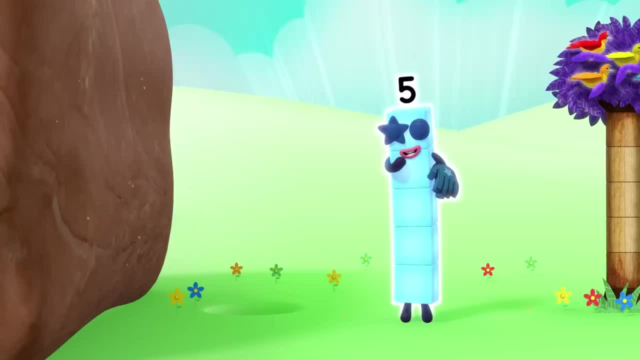 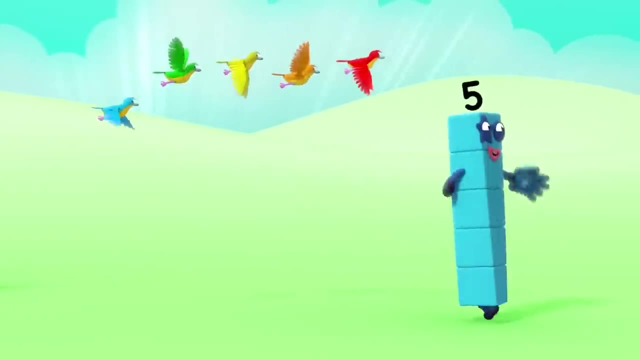 Here I am and I am five. What a wonderful way to arrive. One, two, three, four, five. What an amazing, fantastic, terrific and wonderful day to be alive. One, two, three, four, five. 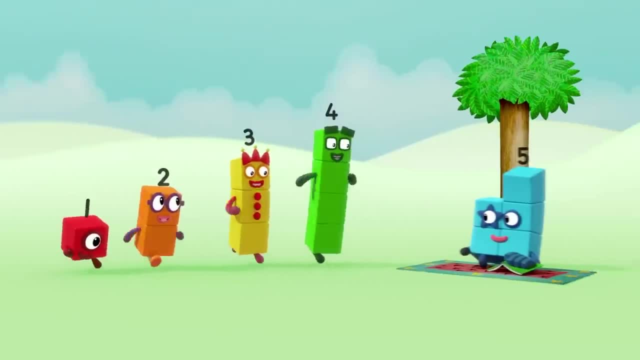 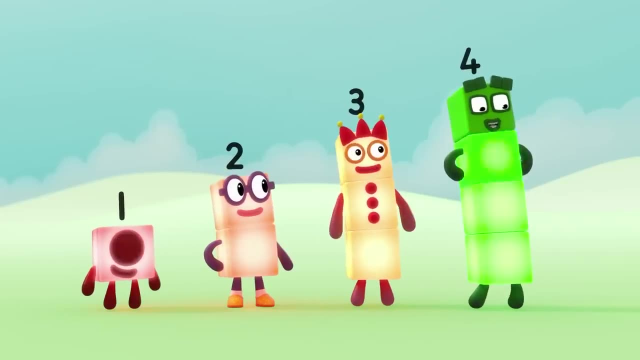 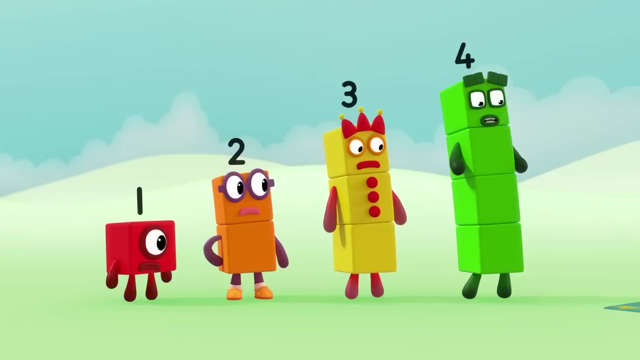 Oh yeah, Oh Hey, Found you There she is. Hello, We're playing hide-and-seek. Want to join in? I would absolutely love to You hide and I'll seek. You won't find us sat there. 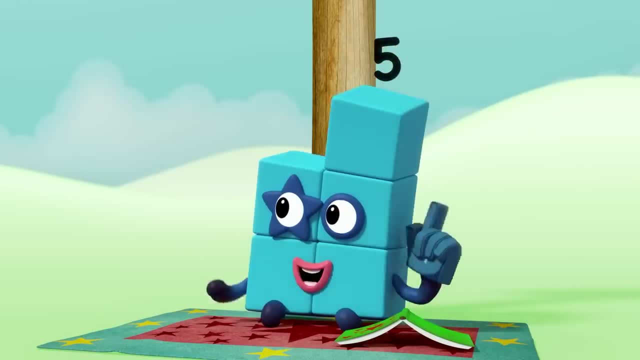 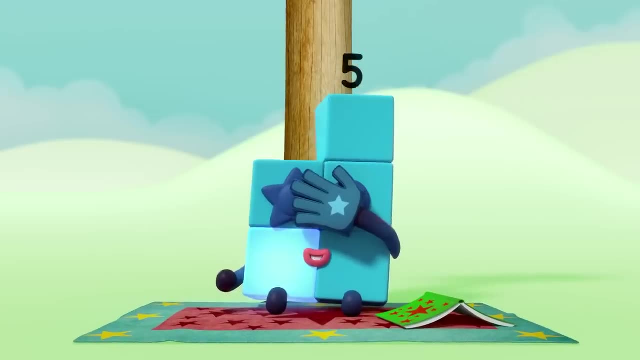 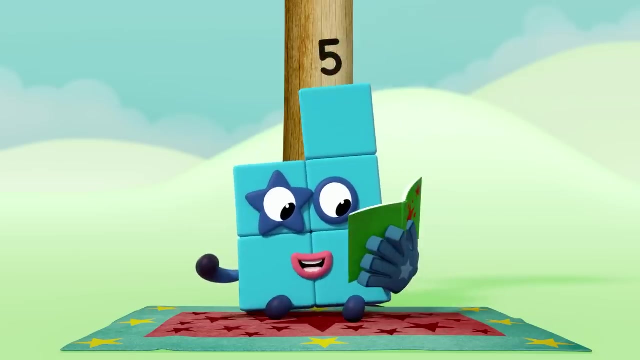 Oh, will I not? now I'm good at this game. I'll find you and point you out: One, two, three, four, five, Ready or not. here I get on with my book. HE LAUGHS. 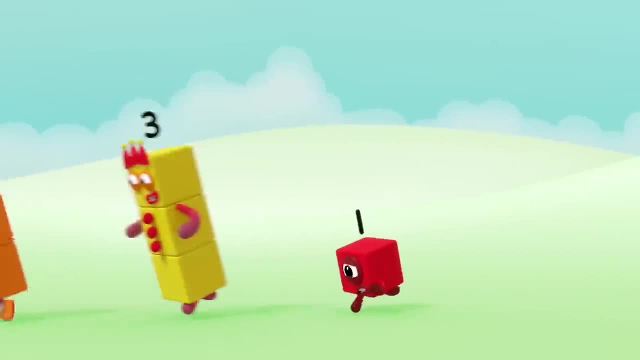 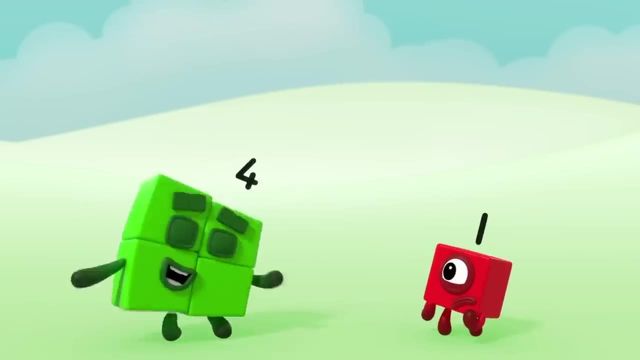 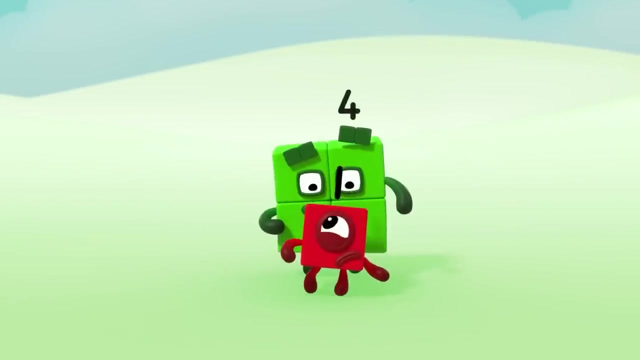 HE LAUGHS, HE GASPS, HE SIGHS, HE GASPS, HE GASPS, HE SIGHS. Hey, Hide behind me. HE SIGHS, HE GASPS, HE SIGHS. Where can I hide? I know behind you. Four Er psst. 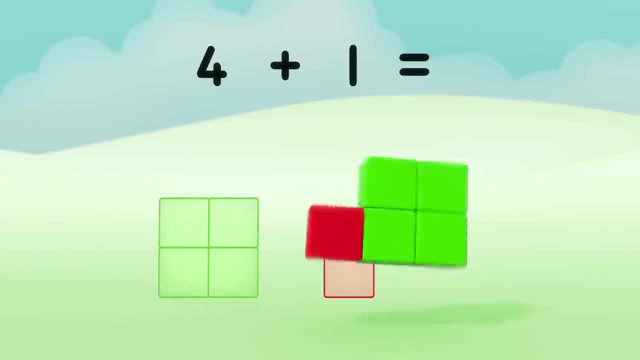 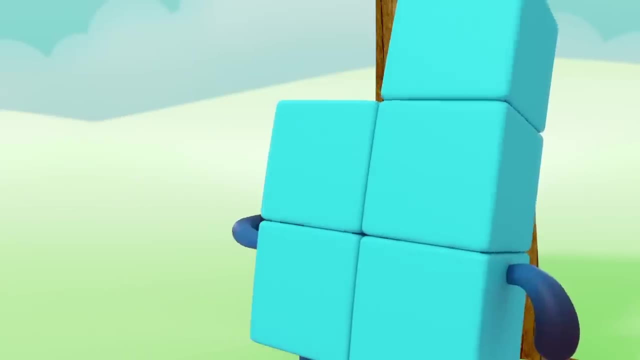 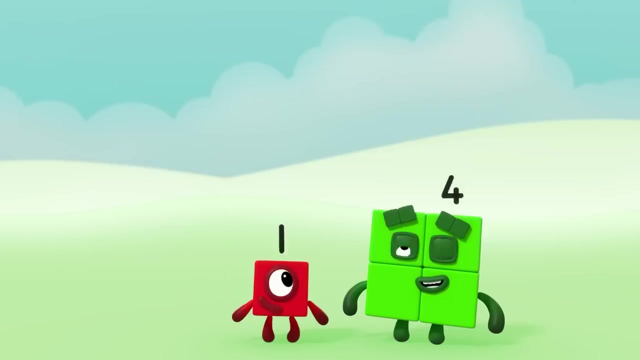 HE GASPS: Four Plus one, equal five MORE. SINGING, Ready or not, here I come, Found you four. Oh, a new one. Five minus one Equals four. Look Five, said she'd point us out. 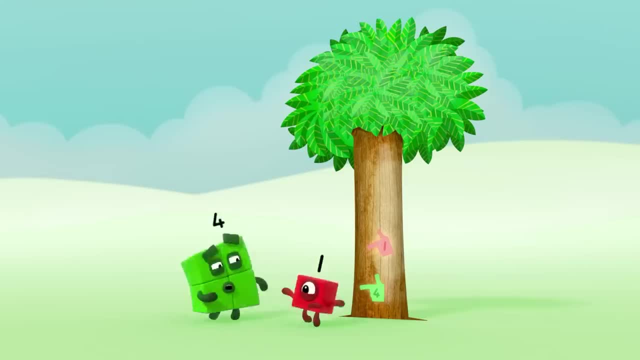 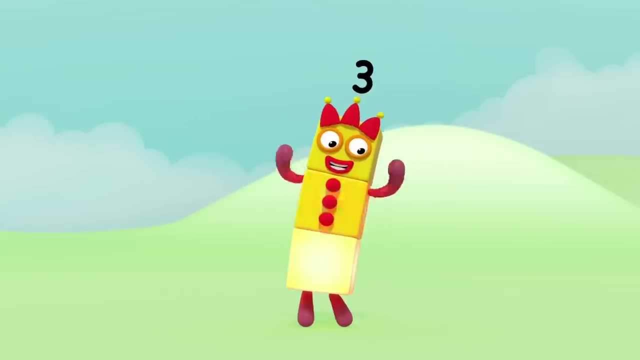 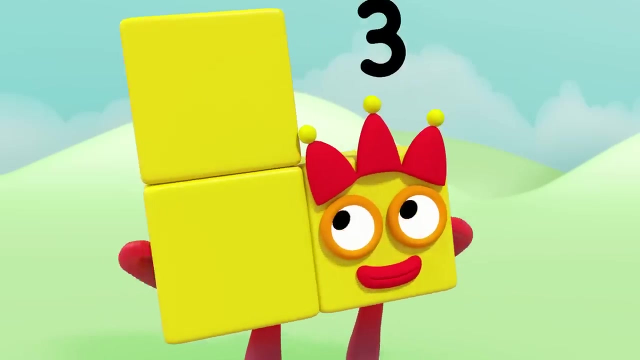 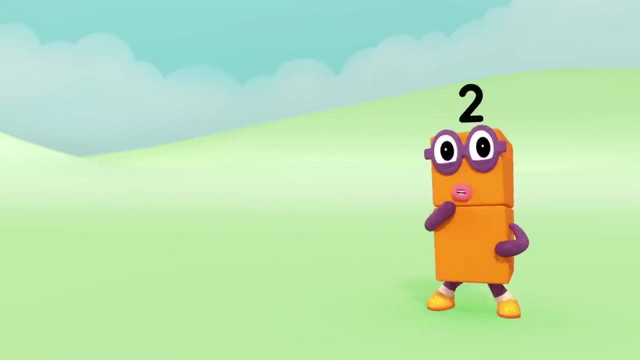 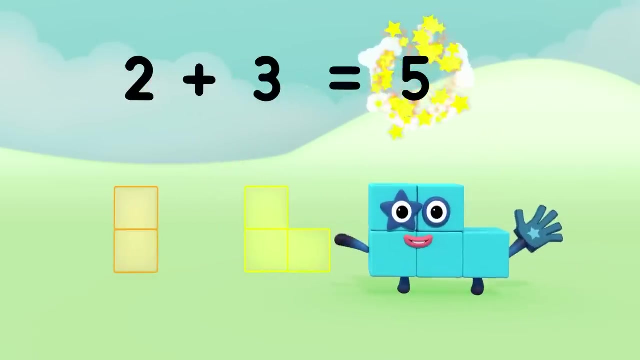 Five was right here. How I am. Three, Master of Disguise. Ah, Ah, Ah, Shhh, Shhh. Two Plus three Equals five. Ready or not, here I be. Find you two, find you three. 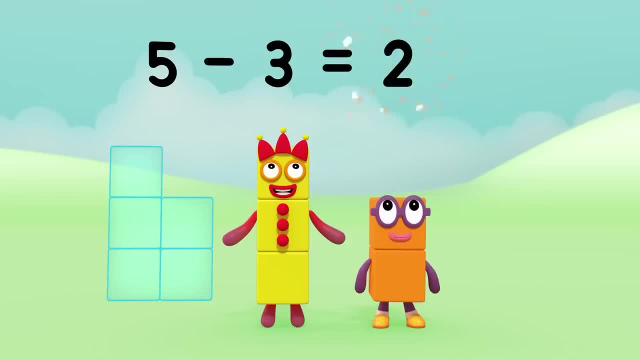 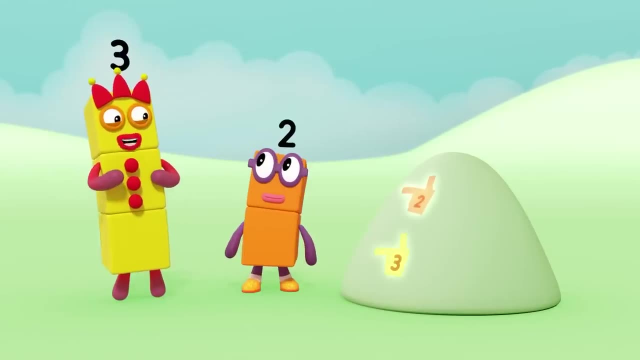 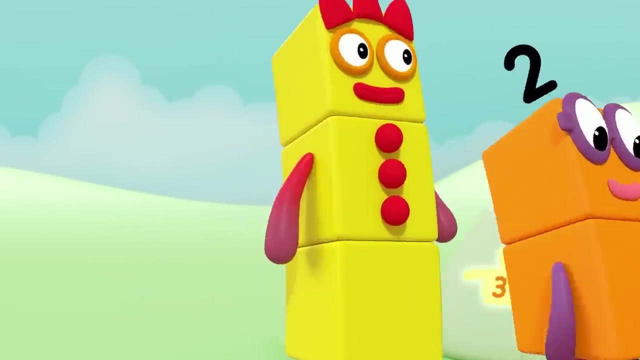 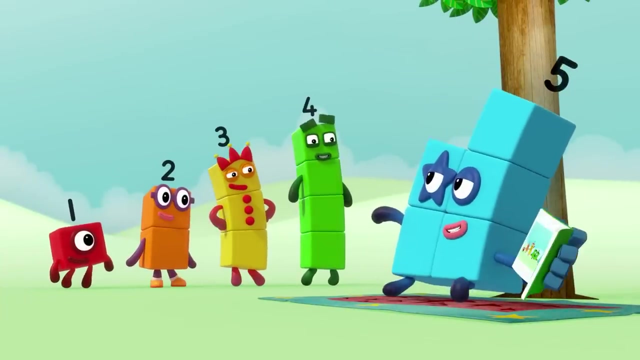 Five minus three Equals two. A pair of pointing prints. Five found us, But but how, Er Five, You're here. How did you Told you I was good. Now my turn to hide Only day. 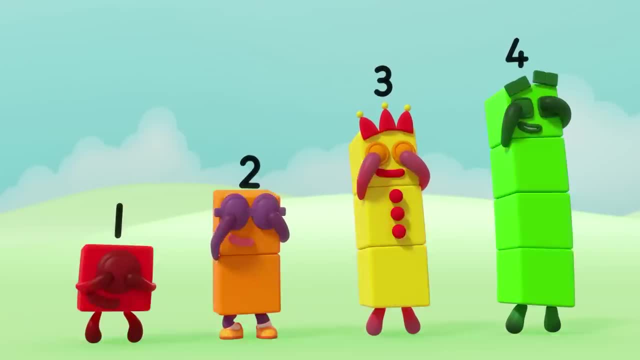 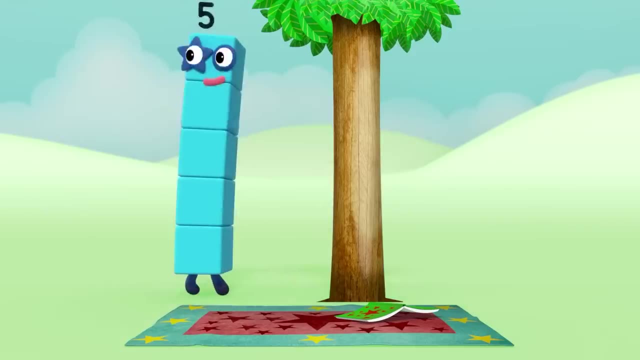 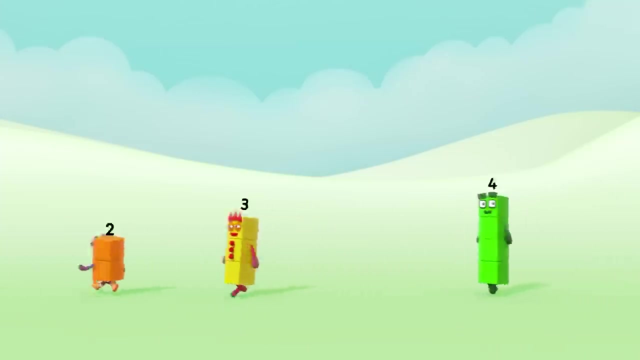 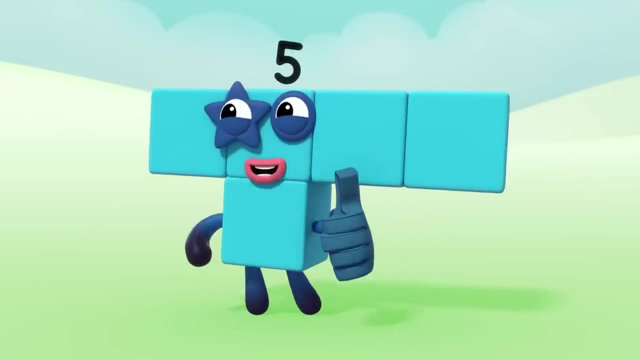 One, Two, Three, Four, Ready or not? Five, here we come, Ooh Rock. One Plus four Equals Five. Found you Amazing? Can you find me again? Five Minus four Equals one. 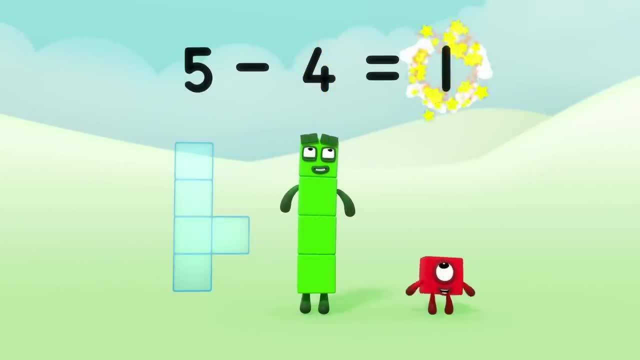 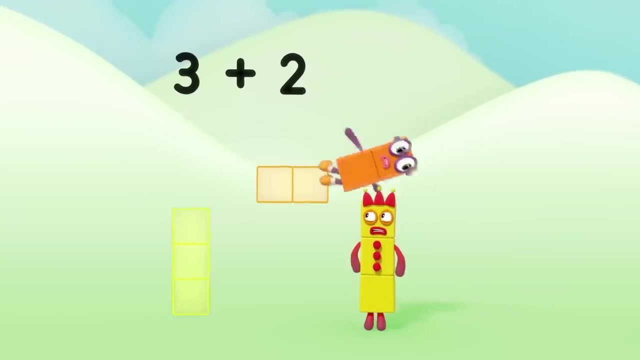